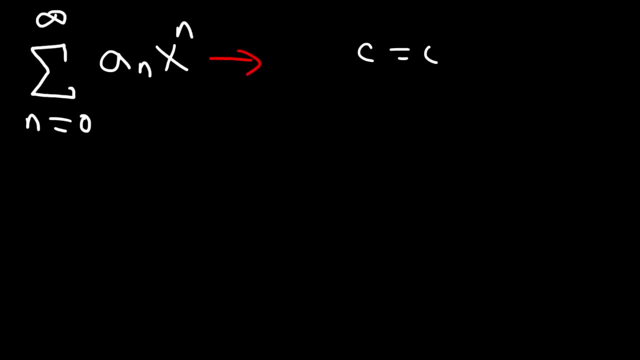 at zero. So c is equal to zero for this one. And here's another power series, but this one is not centered at zero. In this case, the center is c. Now, the first thing you need to be able to do is determine where it's centered at. So let 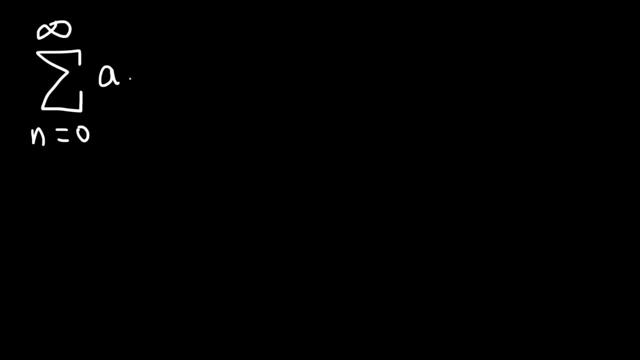 me give you some examples. So for each of these examples determine where each power series is centered at. Feel free to pause the video and try it Now. let's consider the first one on the upper left. Where is the power series centered at? So just by looking at it, you can see that it's centered at c equals. 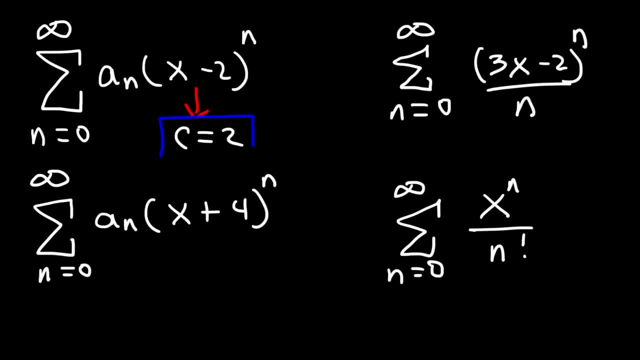 two. Now what about the second one on the bottom left? Another way you could find the answer is by setting the inside. in this case x plus four, equal to zero, and solve for x, So at negative four this whole thing becomes zero. So it's centered at c equals negative four. Now for this one. if 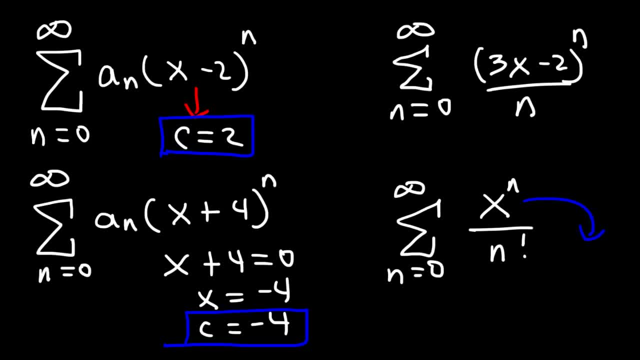 you don't see a c value. if it's just x to the n, then it's centered at zero. You can write this as x minus zero to the n, and that's the same as x to the n. Now, what about the last example? If you don't see what it is, immediately set the. 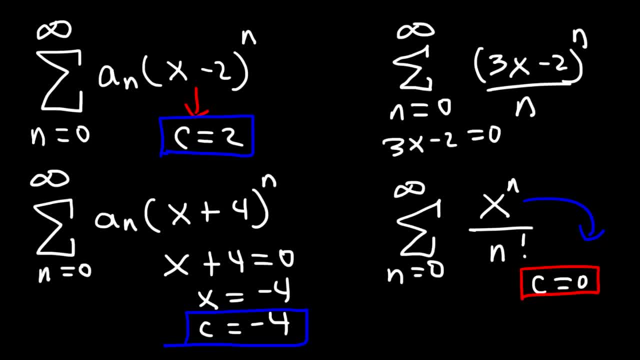 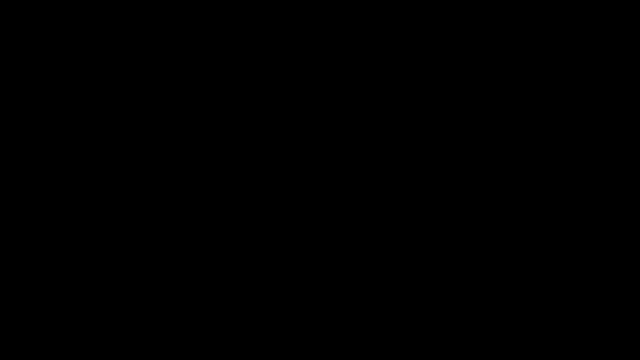 inside part three: x minus two equal to zero, and solve for x, And so you should get: x is two over three, and so it's centered at that value. Now, the next thing that we need to be able to do is we need to determine. 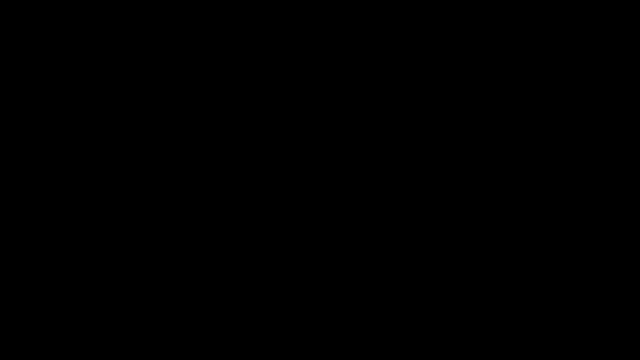 where the power series is centered at. So let's go ahead and do that. So let's take the radius of convergence and the interval of convergence of a power series, And so you need to use the ratio test to do that. So let's say, if you use 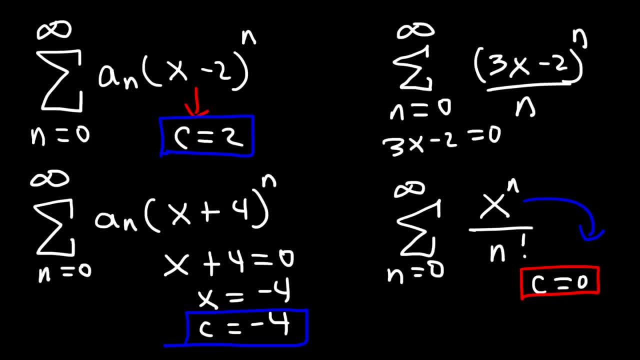 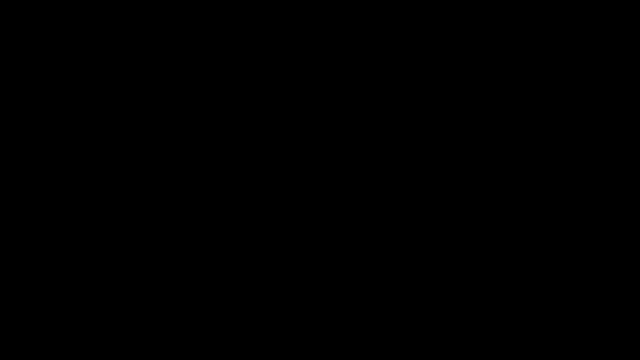 inside part three: x minus two equal to zero, and solve for x, And so you should get: x is two over three, and so it's centered at that value. Now, the next thing that we need to be able to do is we need to determine. 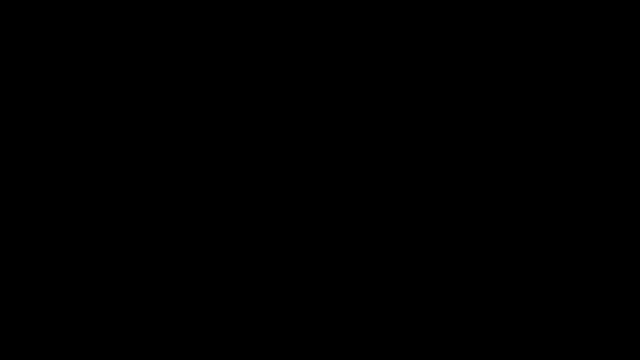 where the power series is centered at. So let's go ahead and do that. So let's take the radius of convergence and the interval of convergence of a power series, And so you need to use the ratio test to do that. So let's say, if you use 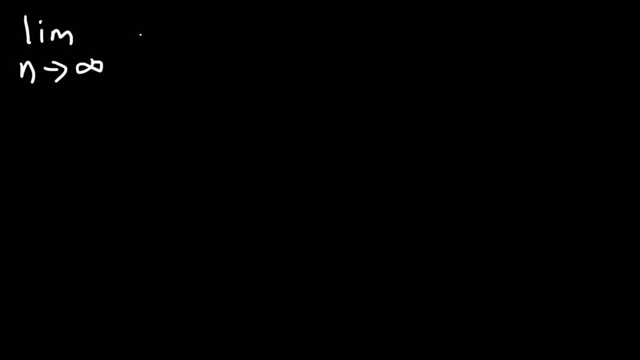 a ratio test. you take the limit- as n goes to infinity, of u sub n plus one divided by u sub n. Now let's say, if you get zero, What does this mean? There's three scenarios you need to be familiar with. This is the first one. So if the ratio 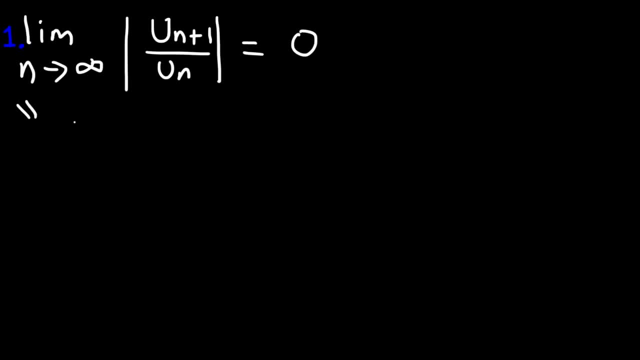 test gives you zero, then it means that the series it converges for all x values It's always convergent. So the radius of convergence, that's r, that's equal to infinity, And the interval of convergence, it's from negative infinity to infinity. 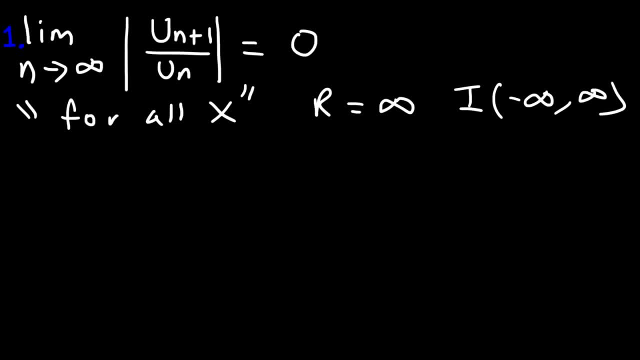 So what this means is that at any x value, the power series will converge. Now the solution is: after doing the ratio test, let's say you don't get zero. Let's say this time you get infinity instead of zero. So what does that mean? Now, if you recall, in order, 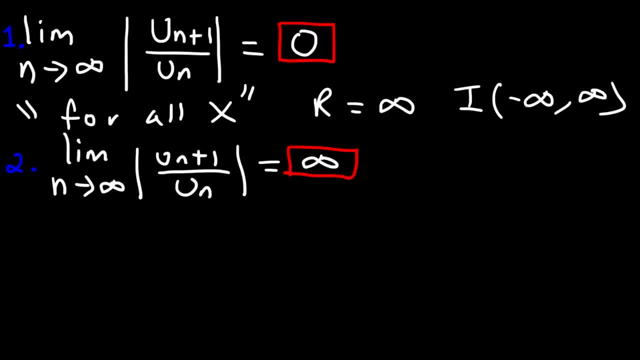 for a series to converge, the ratio tests have to give you an answer that's less than one. So if it's greater than one or if it's infinity, that means that it diverges for all x values except one particular x value. It will only converge when x is equal. 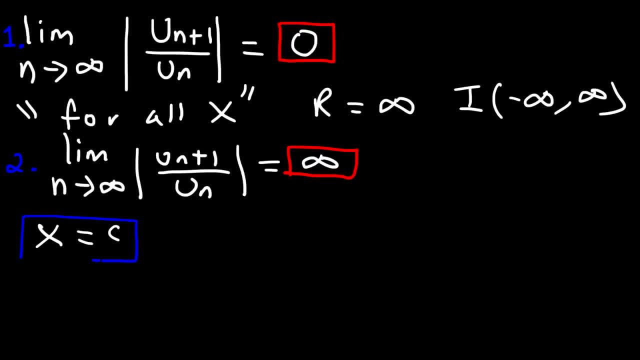 to c. At this point you're going to get a limit with some expression of n times zero. So the whole limit is equal to zero And because, according to the ratio, test is less than one, it's going to converge for that point, But for everywhere else, for all other x values. 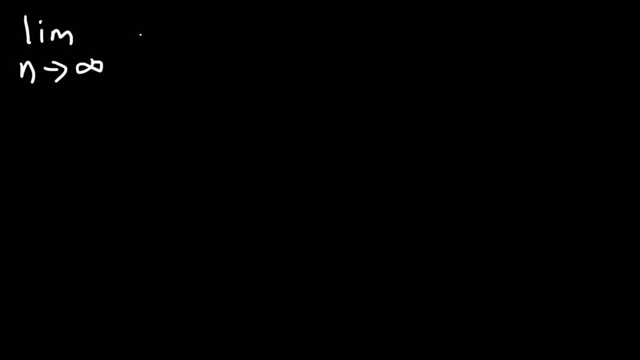 a ratio test. you take the limit- as n goes to infinity, of u sub n plus one divided by u sub n. Now let's say, if you get zero, What does this mean? There's three scenarios you need to be familiar with. This is the first one. So if the ratio 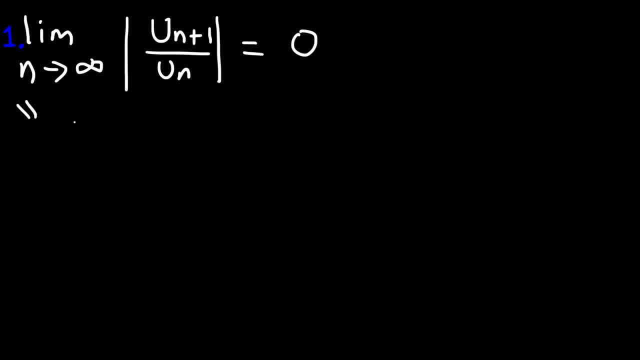 x gives you zero, then it means that the series it converges for all x values, it's always convergent. So the radius of convergence, that's r, that's equal to infinity, And the interval of convergence, it's from negative infinity to infinity. 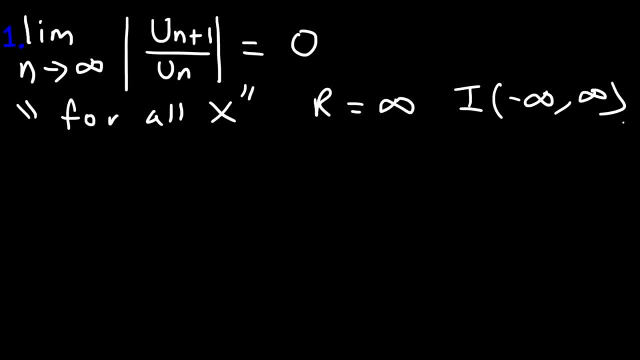 So what this means is that at any x value, the power series will converge. Now The second situation is after doing the ratio test. let's say you don't get 0.. Let's say, this time you get infinity instead of 0.. 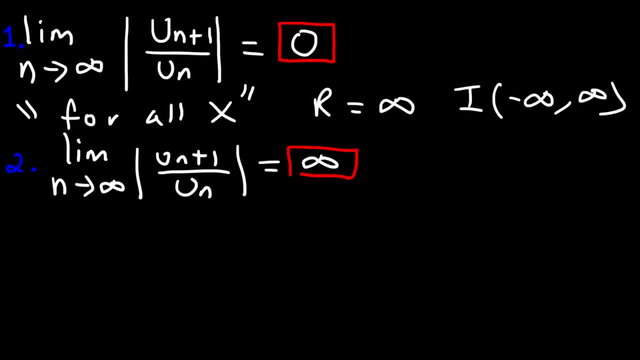 So what does that mean? Now, if you recall, in order for a series to converge, the ratio tests have to give you an answer that's less than 1.. So if it's greater than 1 or if it's infinity, that means that it diverges for all x values. 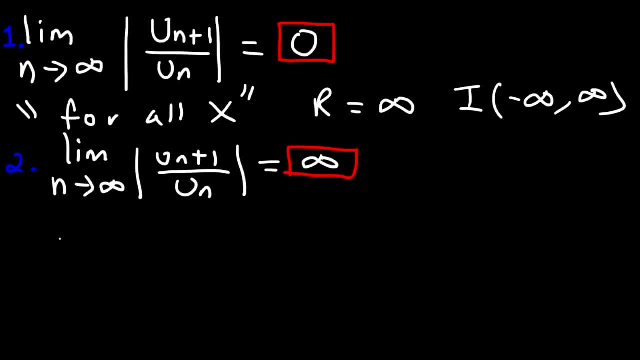 except one particular x value. It will only converge when x is equal to c. At this point you're going to get a limit with some expression of n times 0, so the whole limit is equal to 0. And because, according to the ratio test, it's less than 1, it's going to converge. 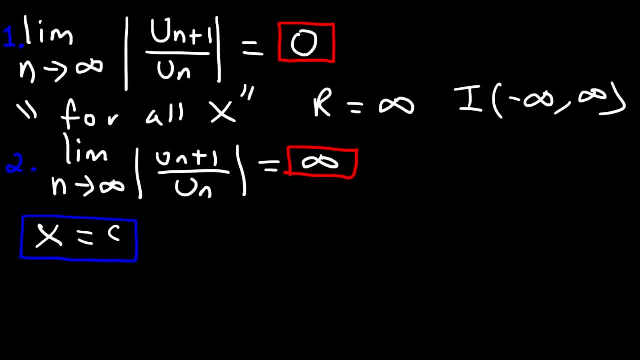 for that point, But for everywhere else, for all other x values, that is not equal to c, you're going to get infinity, and so the series will diverge for all other x values, But for this particular x value, where x is equal to c, it's going to converge. 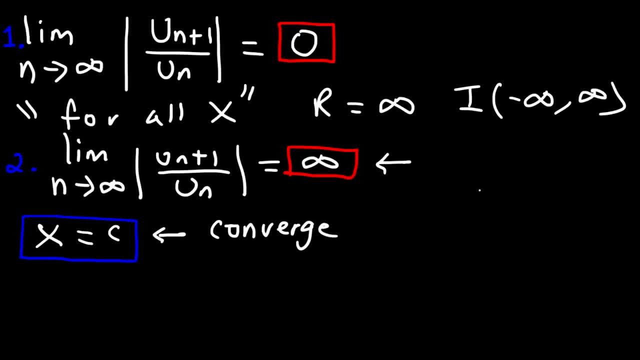 And because it only converges at one finite number. the radius of convergence is 0.. And the interval of convergence is only 1.. There's only one number, it's not a range of numbers. So the interval of convergence is just: the x equals c value or c itself. 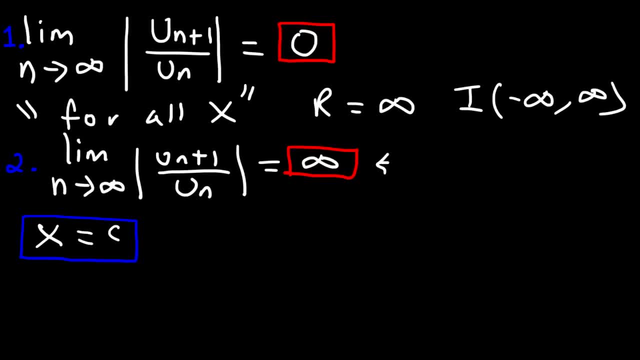 that is not equal to c, you're going to get infinity, And so the series will diverge for all other x values. But for this particular x value, where x is equal to c, it's going to converge, And because it only converges at one finite number, the radius of convergence. 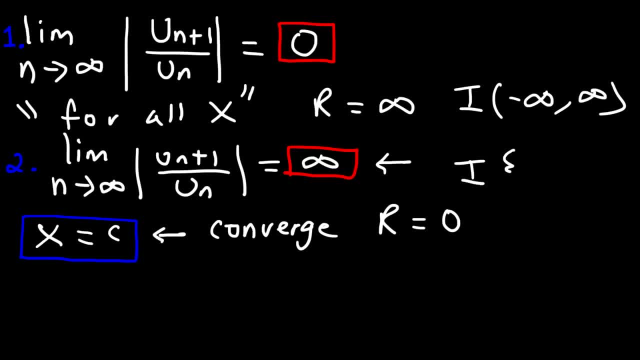 is zero And the interval of convergence is only one number, It's not a range of numbers. So the interval of convergence is just one number And the interval of convergence is zero. And the interval of convergence is only one number, It's not a range of numbers. 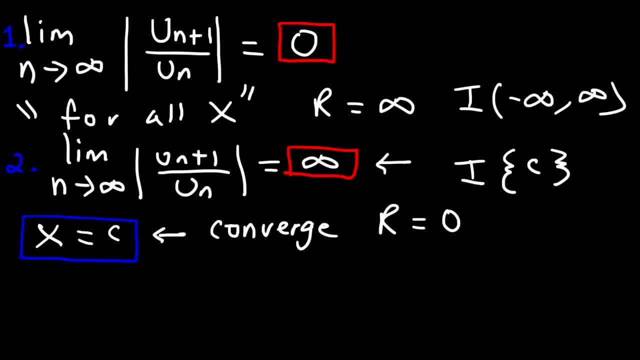 It's just the x equals c value or c itself. So let me separate the first situation from the second. Let's move on to the third situation. So for the third scenario, if we use the ratio test, we're going to get an expression. 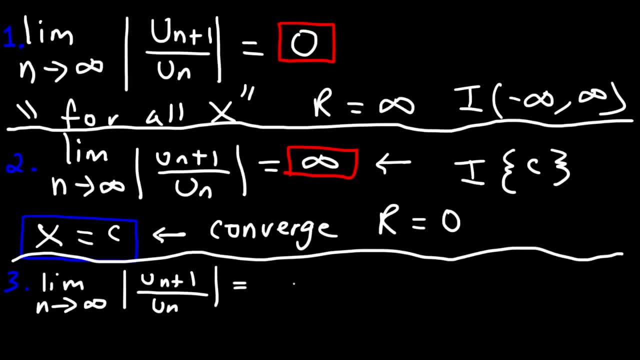 In terms of x. Typically it's going to look something like this: One over r. absolute value, x minus c, which is less than one. So it's going to vary, but c could be four, c could be zero, So you may just see an absolute value of x. r could be anything It could. 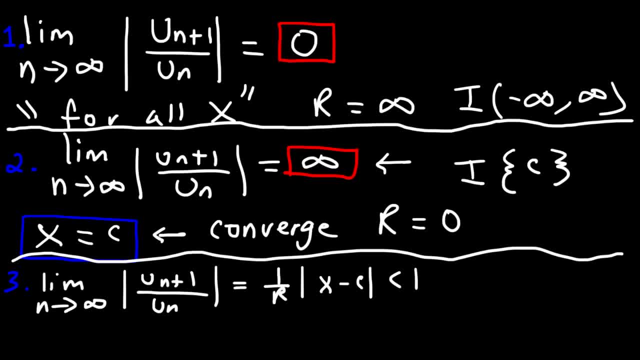 be one half, It could be two, But usually in this format. And once you get to this point, you want to multiply both sides by r And keep in mind you want to set it less than one Because you'll get this, but you need to introduce this inequality Because it only 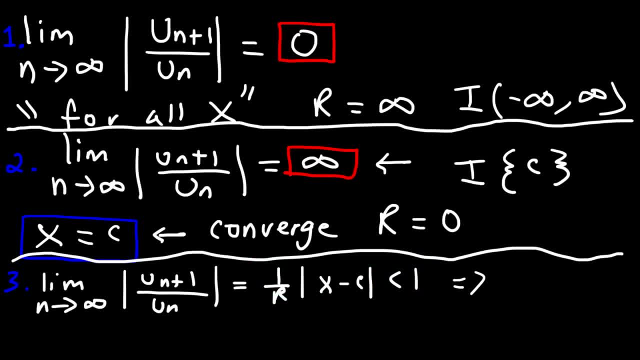 converges when a ratio test gives you a value less than one. So this is something that you have to add, The less than one part, And then, once you multiply both sides by r for this expression, you're going to get x minus c is less than r. So whatever number you see, 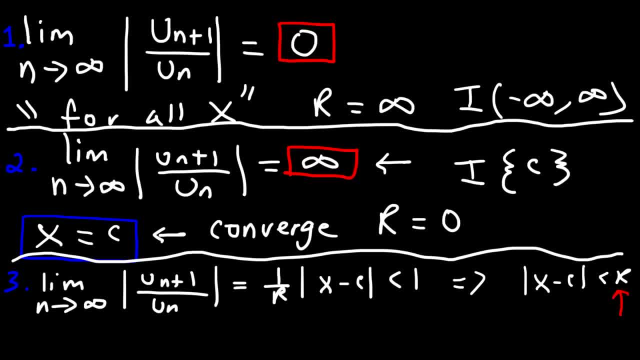 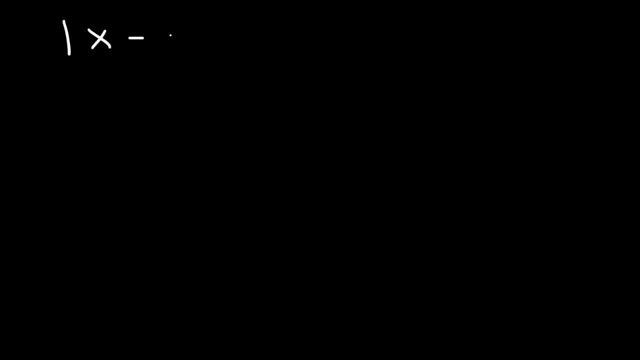 at this point, that is your radius of convergence. Now, because of space, I'm going to clear the board, So let's start with this. So this is where the series converges. Now, whenever the absolute value of x minus c is greater than r, then at that point, in. 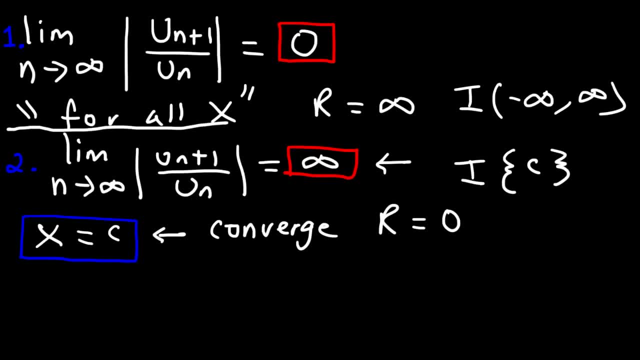 So let me separate the first situation from the second. Let's move on to the third situation. So for the third scenario, if we use the ratio test, Okay, We're going to get an expression in terms of x. Typically it's going to look something like this: 1 over r. absolute value, x minus c. 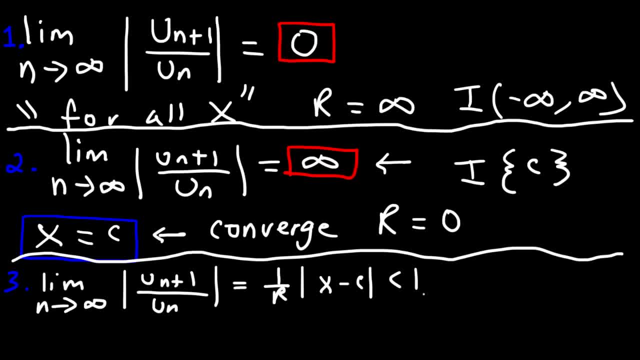 which is less than 1.. So it's going to vary, but c could be 4,, c could be 0, so you may just see an absolute value of x. r could be anything, it could be 1, half, it could be 2, but usually in this format. 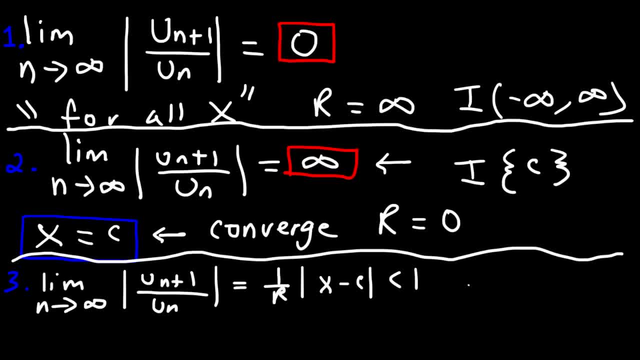 And once you get to this point, you want to multiply both sides by r And keep in mind, you want to set it less than 1, because you'll get this. but you need to introduce this inequality because it only converges when a ratio test gives you a value. 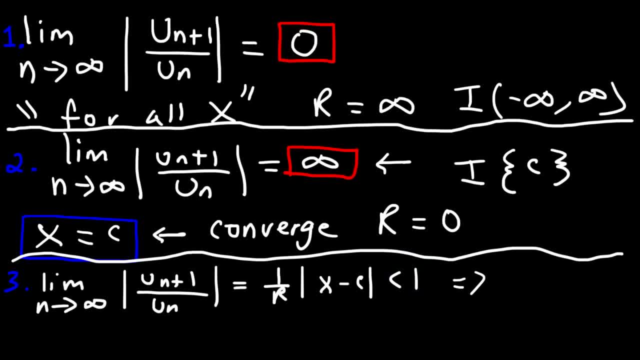 less than 1.. So this is something that you have to add, the less than 1 part, And then, once you multiply both sides by r for this expression, you're going to get x minus c is less than r. So whatever number you see at this point, you're going to get x minus c is less than. 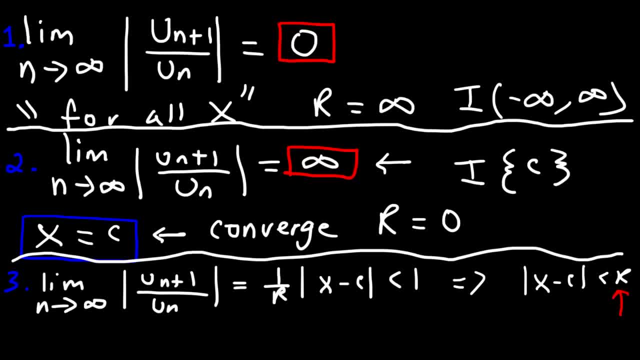 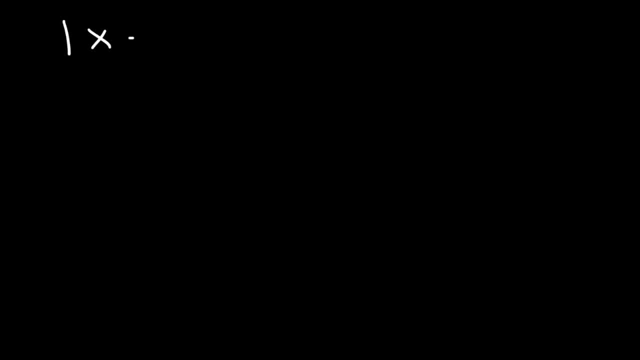 r, And at this point that is your radius of convergence. Now, because of space, I'm going to clear the board, So let's start with this. So this is where the series converges. Now, whenever the absolute value of x minus c is greater than r, then at that point the 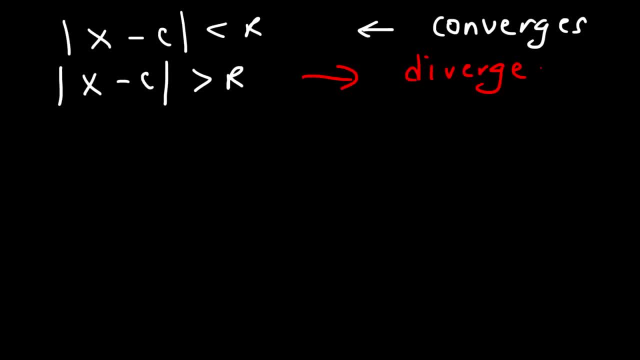 series. it diverges, But since we're looking for the radius of convergence, We're not going to use this, So we're just going to be focusing on this expression. Now. to get rid of the absolute value symbol, we could say that x minus c is less than r. 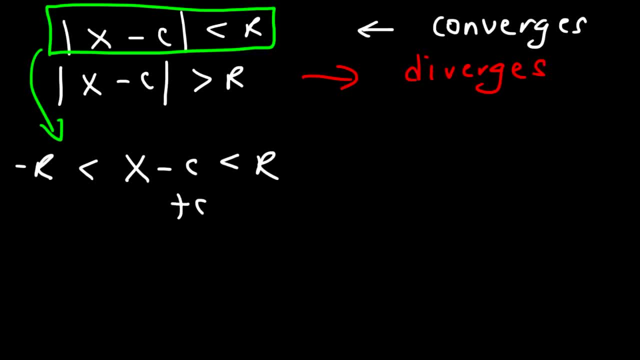 but greater than negative r. Now if you add c to both sides, you'll get that x is between negative r plus c and r plus c. So the interval of convergence becomes this: It's negative r plus c, comma r plus c. Now the last thing you need to do is check the endpoints. 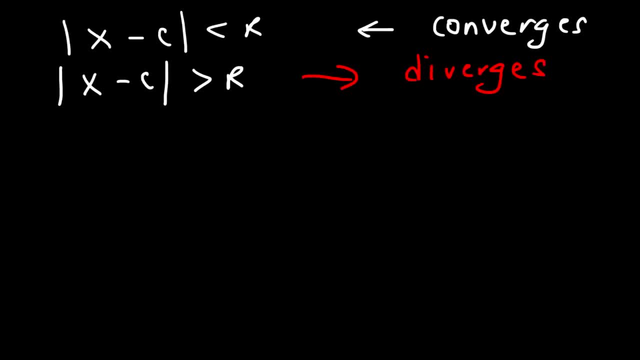 the series. it diverges, But since we're looking for the radius of convergence, we're not going to use this, So we're just going to be focusing on this. Można this expression now to get rid of the absolute value symbol, we could say that x minus c is less. 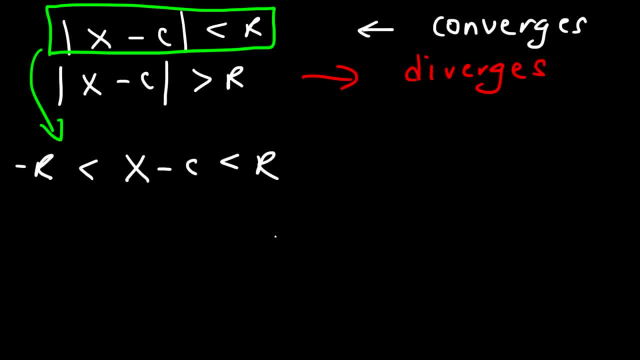 than r, but greater than negative r. now if you add c to both sides, you'll get that x is between negative r plus c and r plus c. so the interval of convergence becomes this: it's negative r plus c, comma r plus c. now the last thing you need to do is check the endpoints, because even though you 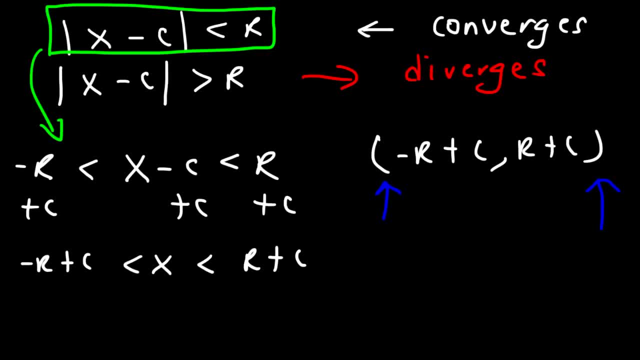 have parentheses here. sometimes you could have two brackets, two parentheses- a bracket and a parentheses or parentheses in the bracket. so there's four possibilities here and you have to check your endpoints, which i need to show you by example. but that's how you could find the interval of convergence. so now you know the three scenarios, so let's work on the. 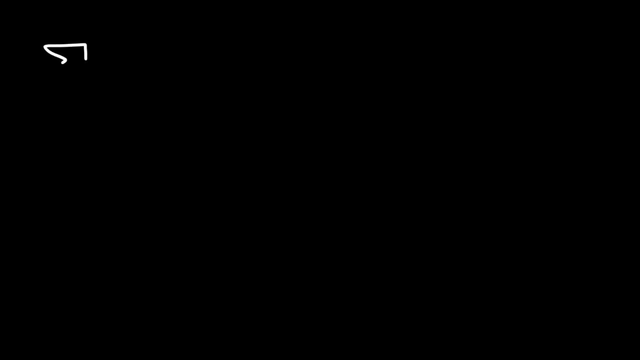 some practice problems. so let's say, if we have the power series from 0 to infinity, of x to the n over n factorial, go ahead and determine the radius and the interval of convergence for this power series. so let's start with the ratio, test the limit as n goes to infinity of 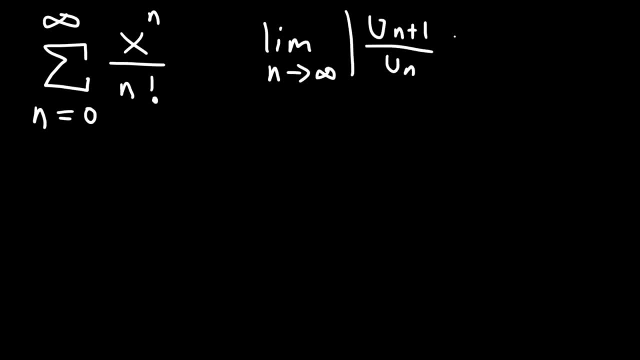 u sub n plus 1, divided by u sub n. we need to see where it's less than 1, where the series converges. so u sub n plus 1. all you got to do is, in this expression, replace n with n plus one, so it's. 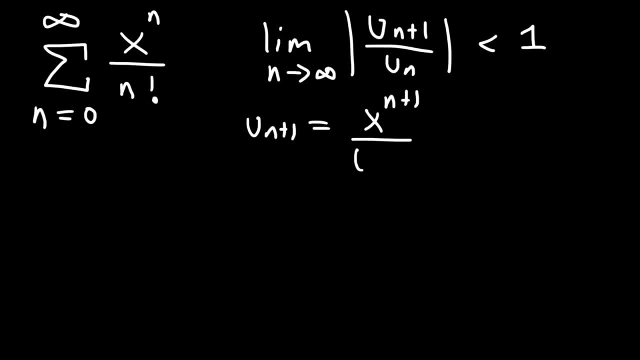 x to the n plus 1 divided by n plus 1 factorial. and you said: then that's just the original expression, x to the n over n factorial. so let's take the limit, as n goes to infinity, of u sub n plus 1, so that's this, and then divided by u sub n. 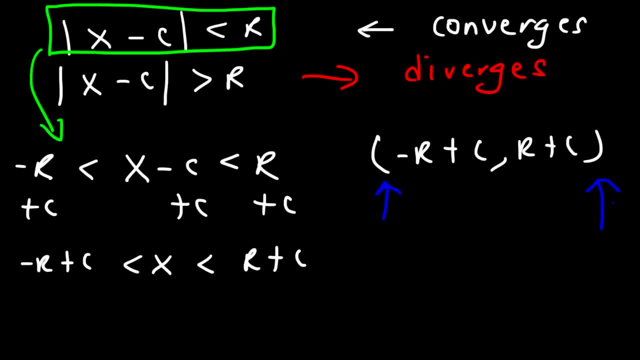 Because, even though you have parentheses here, sometimes you could have two brackets, two parentheses, a bracket and a parentheses or parentheses and a bracket. So there's four possibilities here and you have to check your endpoints, which I need to show you by example. 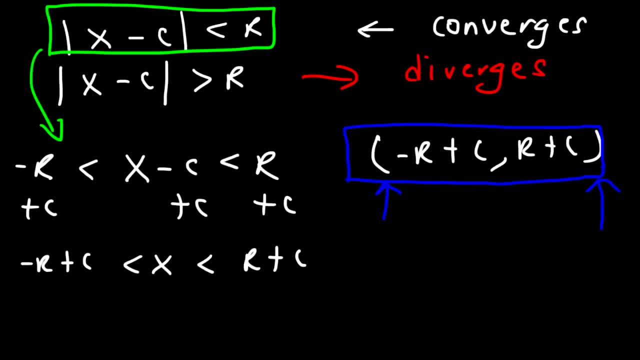 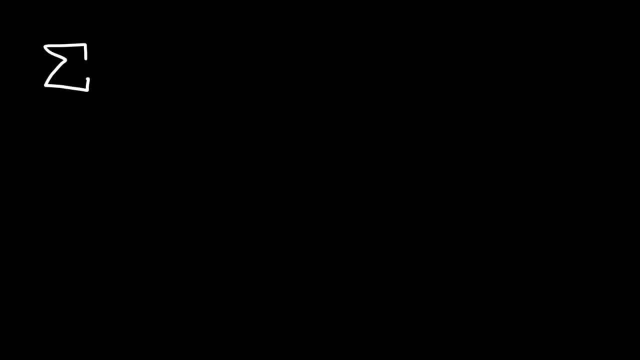 But that's how you could find the interval of convergence. So now you know the three scenarios. So let's work on some practice problems. So let's say, if we have the power series from zero to infinity, of x to the n over n, factorial, 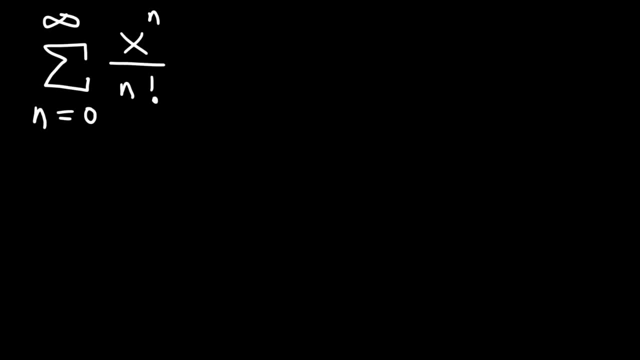 Go ahead and determine the radius and the interval of convergence for this power series. So let's start with the ratio test, The limit, as n goes to infinity, of u sub n plus one. Divide that by two. Divide that by u sub n. 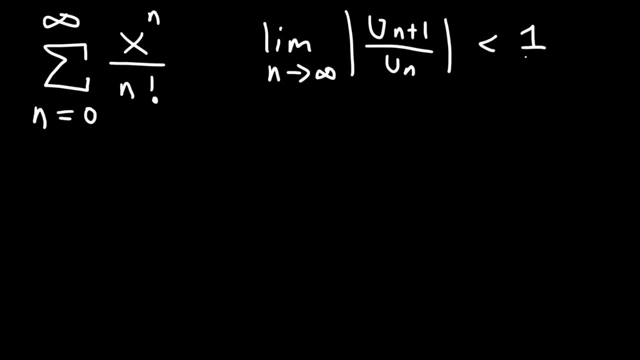 And we need to see where it's less than one, where the series converges. So u sub n plus one. All you got to do is, in this expression, replace n with n plus one, So it's x to the n plus one divided by n plus one. factorial. 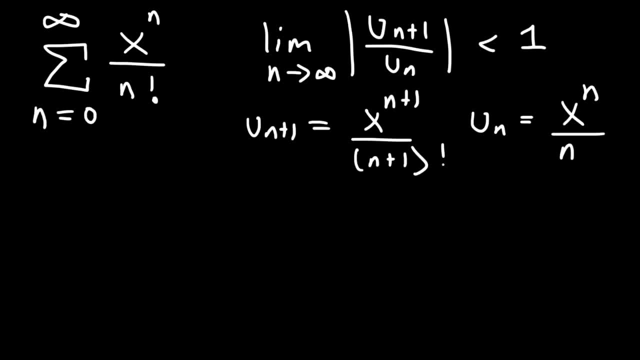 And u sub n. that's just the original expression: x to the n over n- factorial. So let's take the limit As n goes to infinity. So let's say that x goes to infinity, of x to the n plus one, And then in this case it can be n plus one. 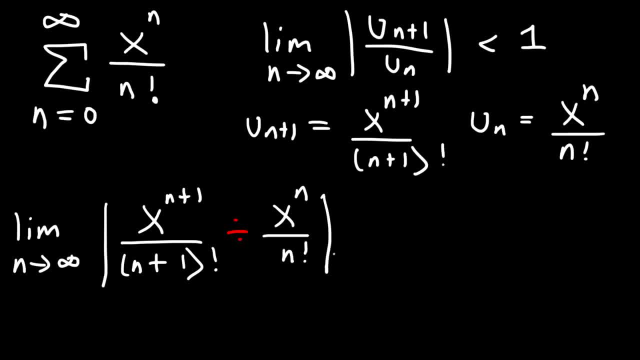 So that's this, And then divided by u sub n. So let's simplify the expression: x to the n plus one. we can say the same thing. we could say: that's x to the n times x to the first power, n plus 1. factorial is n plus 1. 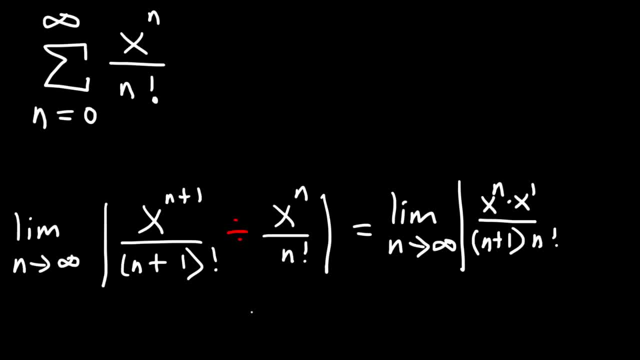 times n factorial And then, using the expression keep, change, flip. we're going to change division to multiplication and we're going to flip the second fraction, So it's n factorial over x to the n. So we can cancel an n factorial and we can also cancel x to the n, And so we're going to be left. 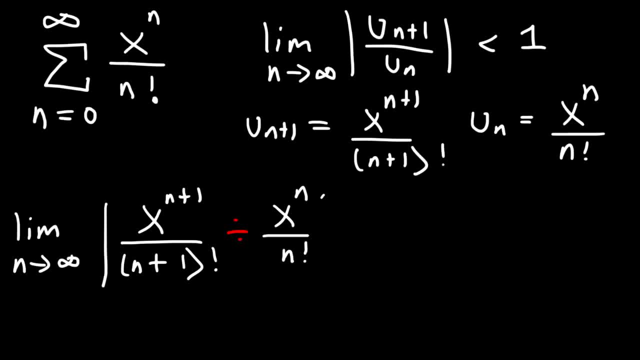 So let's simplify the expression X to the n plus 1, we can say that's x to the n times x to the first power. n plus 1 factorial is n plus 1 times n factorial, and then, using the expression, keep change. 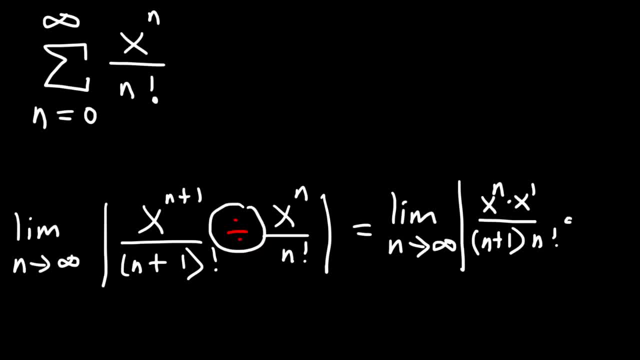 flip. We're going to change division to multiplication and we're going to flip the second fraction, So it's n factorial over x to the n, So we can cancel an n factorial and we can also cancel x to the n, And so we're going to be left over with. so just, I'm continuing from here, just keep. 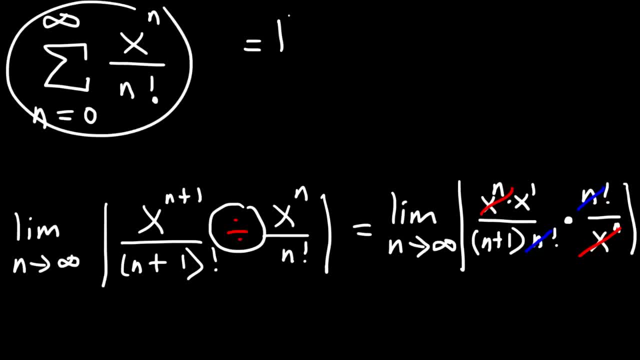 that in mind, I'm not saying this is equal to n. Okay, It's equal to this here. So this is equal to the limit, as n goes to infinity. and then we have absolute value: 1 over n plus 1 times the absolute value of x. 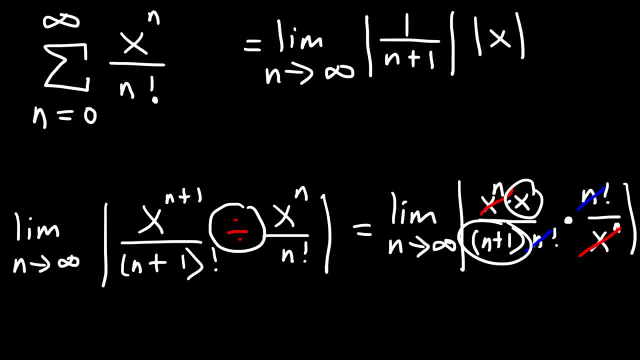 So basically separated x over n plus 1 into those two parts. Now, as n goes to infinity, what happens to 1 over n plus 1?? That's going to go to 0.. And 0 times x, That's going to go to 0.. 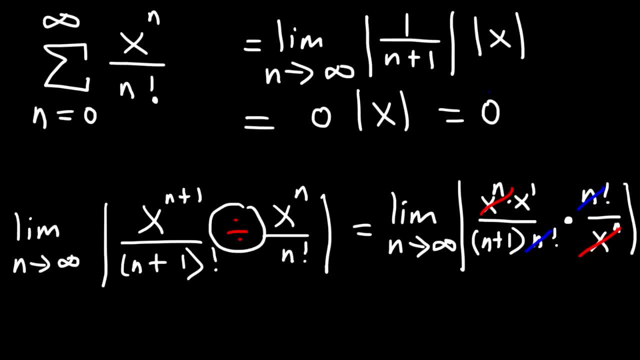 And 0 times x is 0. Now what do we say will happen if we get a limit of 0?? If the limit is equal to 0, which is always less than 1,, then that means that the series, it converges for all x values. 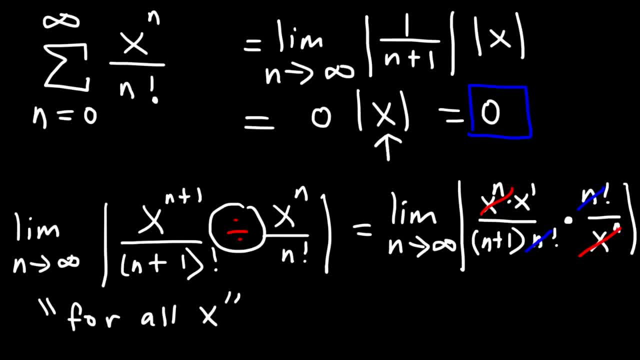 Regardless of what x is, x is a fixed number, by the way. So if you choose x to be 2 or 8 or 25 or negative 4, all of those numbers, all of those fixed values, Multiply by 0 is equal to 0. 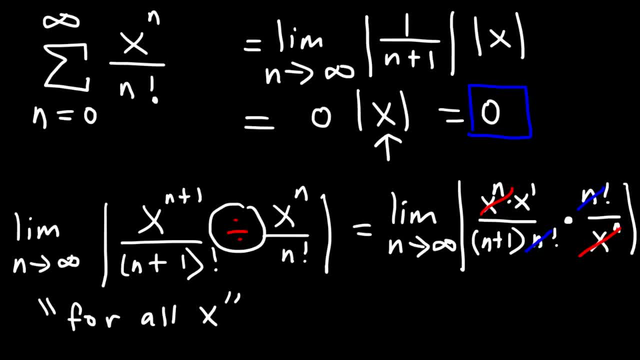 So for any x value that you choose, the series will converge. And so what does this mean? So, for this situation, I believe we define it to be what was it? scenario number 1, I think That was scenario number 1.. 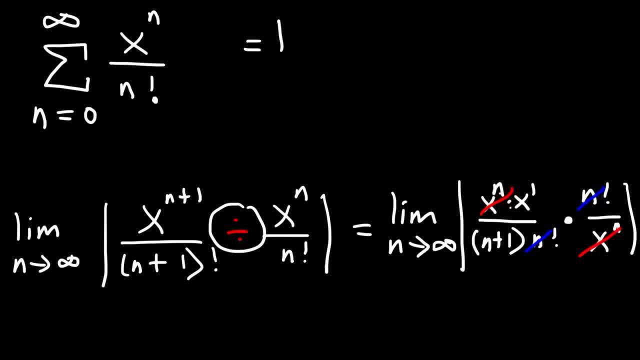 over with. so just I'm continuing from here. just keep that in mind. I'm not saying this is equal to this here. So this is equal to the limit, as n goes to infinity. And then we have afterwards absolute value, 1 over n, plus 1 times the absolute value of x. So basically separated x over n plus. 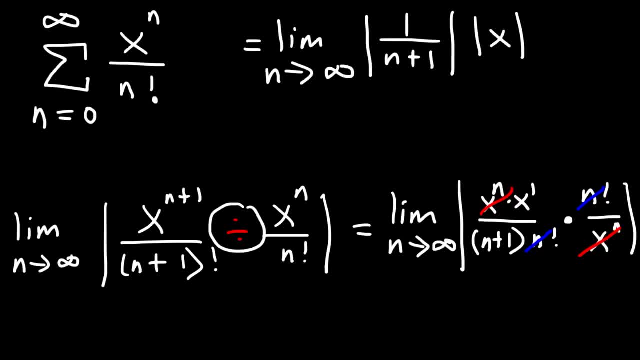 1 into those two parts. Now, as n goes to infinity, what happens to 1 over n plus 1?? That's going to go to 0, and 0 times x is 0. Now what do we say will happen if we get a limit of 0? If the limit 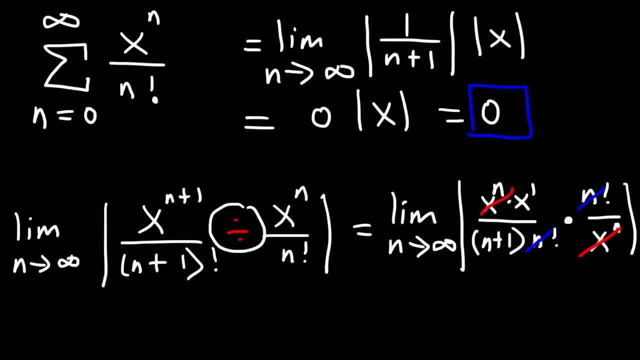 is equal to 0, which is always less than 1, then that means that the series, it converges for all x values, regardless of what x is. X is a fixed number, by the way. so if you choose x to be 2 or 8 or 25 or negative 4, all of those numbers, all of those fixed values, multiplied by 0 is equal to 0. 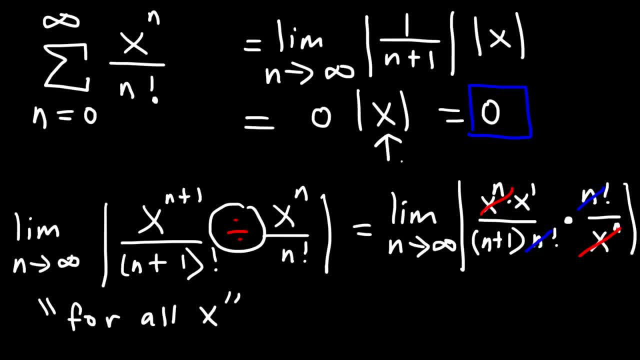 So for any x value that you choose, the series will converge. And so what does this mean? So, for this situation- I believe we define it to be- what was the scenario number one? I think That was scenario number one. and so when a limit equals 0, 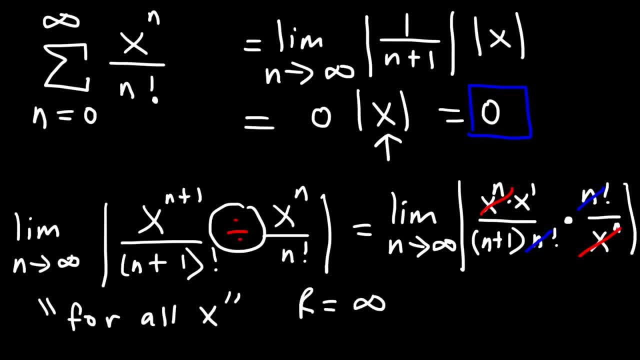 the radius of convergence is infinity and the interval of convergence is negative- infinity to infinity- because x could be anything and the series will converge. X could be a thousand, it will still converge, And so this is the first step we're going to do. So this is the first step we're going to do. 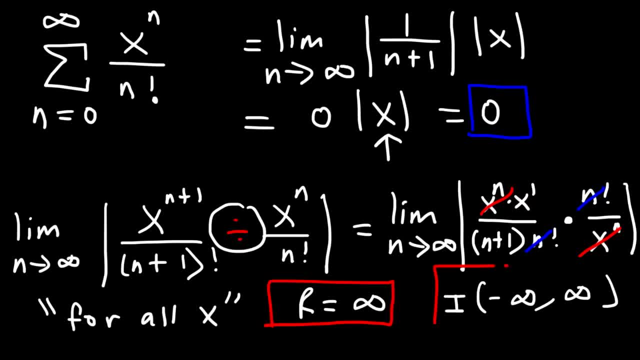 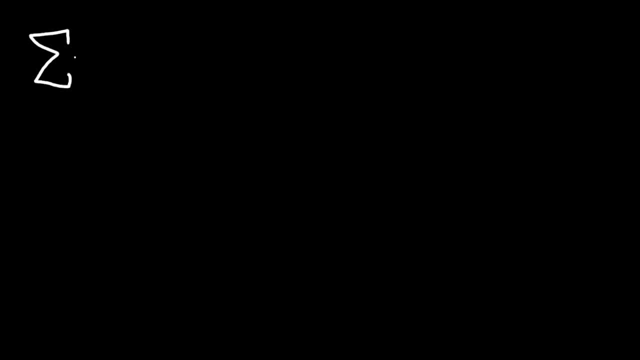 is the answer. anytime you get a limit that's equal to 0.. That's all you need to write. Now let's work on another example. This time we're going to have the series of n- factorial times x to the n. Feel free to pause the video if you want to try it. So let's start with. 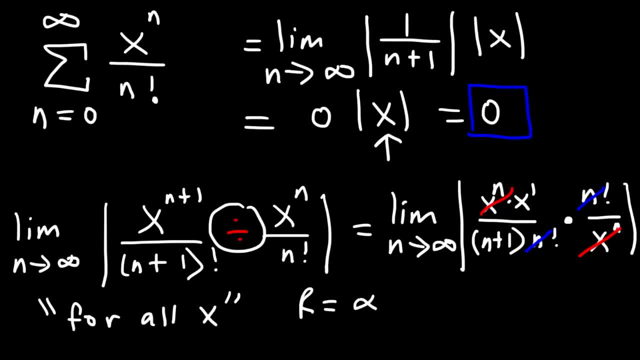 And so when a limit equals 0, the radius of convergence is infinity and the interval of convergence is infinity. And so the radius of convergence is negative infinity to infinity, because x could be anything And the series will converge. x could be 1,000. 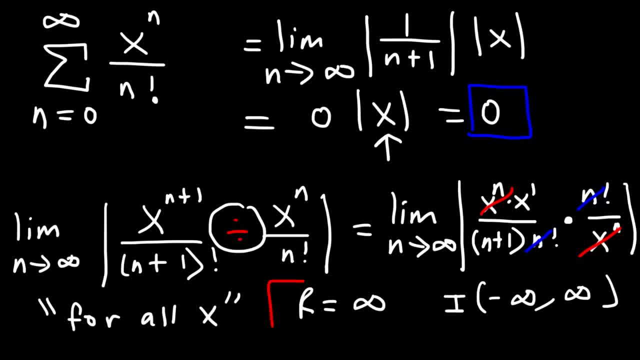 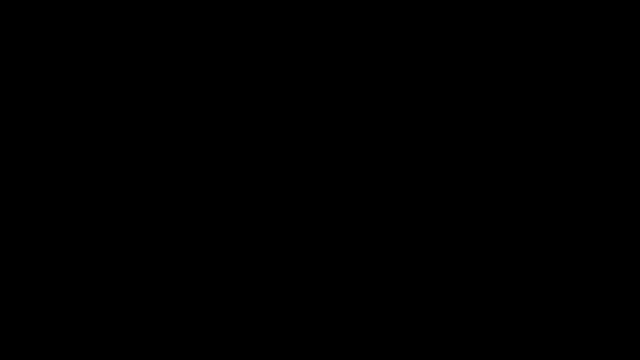 It will still converge, And so this is the answer: any time you get a limit that's equal to 0.. That's all you need to write. Now let's work on another example. This time we're going to have the series of n- factorial times, x to the n. 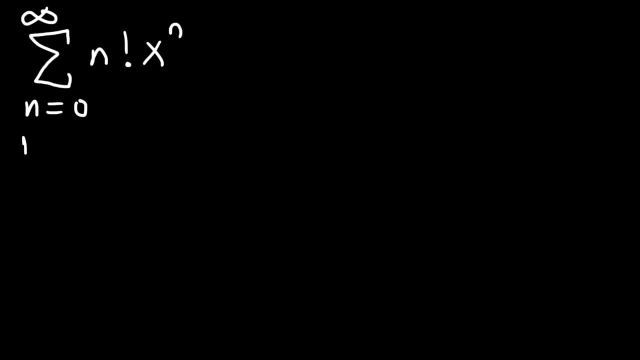 Feel free to pause the video if you want to try it. So let's start with the ratio test Now. u to the n plus 1, that's going to be n plus 1, factorial times x to the n plus 1.. And then we're going to divide it by u to the n, which is the original expression that. 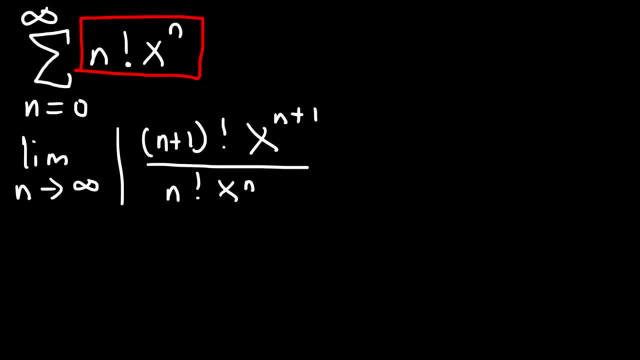 we see here. So that's u to the n. So now let's simplify. So now we have the limit as n goes to infinity, and then n plus 1 factorial, that's n plus 1 times n factorial, and x to the n plus 1, that's x to the n times x to the first. 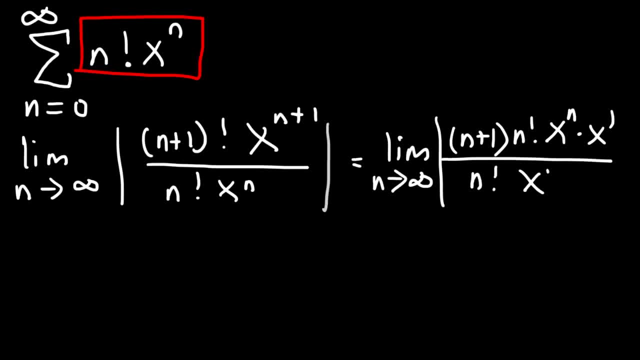 power divided by these two. So now we can cancel x to the n And we can cancel n factorial, And then I'm going to separate n plus 1 and x. So what I now have is that the limit as n goes to infinity of n plus 1, my absolute. 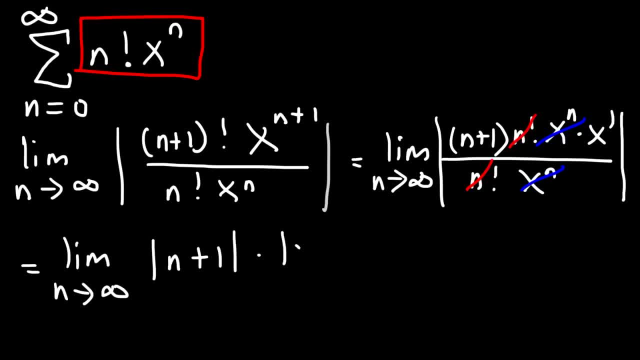 value doesn't need to be so big- and then times the absolute value of x, So you can move this to the front because it's not affected by n. So you can say that The absolute value of x times the limit, as n goes to infinity, of n plus 1.. 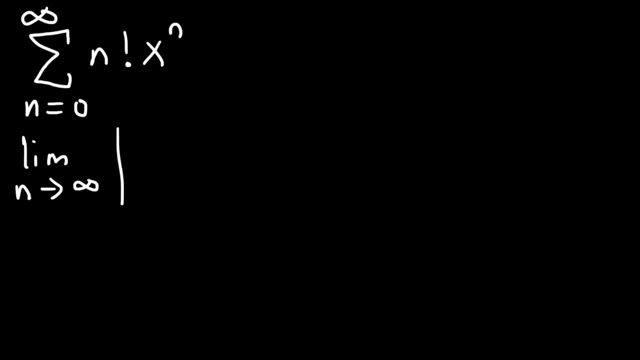 the ratio test Now: u to the n plus 1, that's going to be n plus 1, factorial times x to the n plus 1.. And then we're going to divide it by u to the n, which is the original expression. 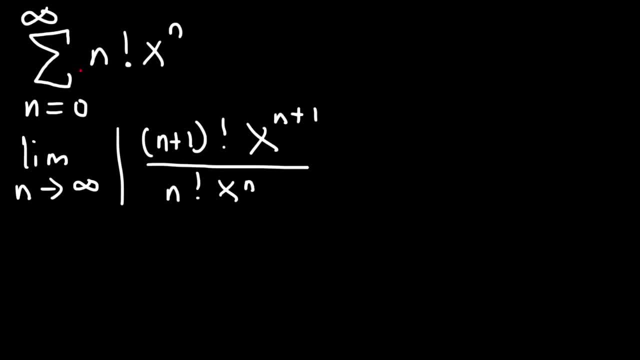 that we see here. So that's u to the n. So now let's simplify. So now we have the limit as 0.. As n goes to infinity, And then n plus 1 factorial, that's n plus 1 times n factorial, And x to 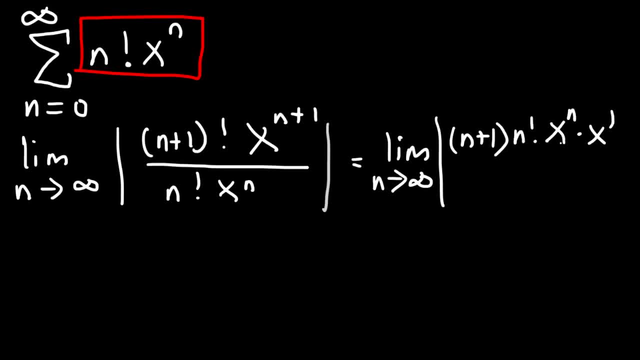 the n plus 1, that's x to the n times x to the first power Divided by these two. So now we can cancel x to the n And we can cancel n factorial, And then I'm going to separate n plus 1 and x. 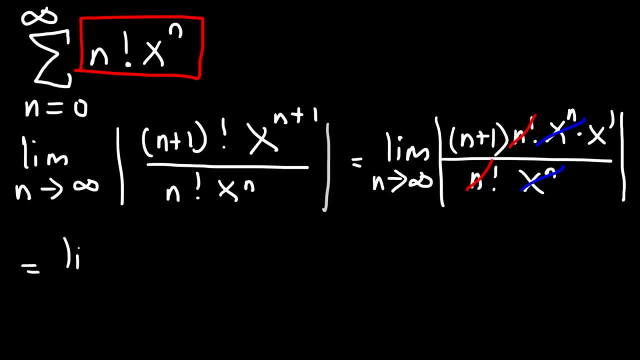 So what I now have is that the limit, as n goes to infinity, of n plus 1, my absolute value doesn't need to be so big- and then times the absolute value of x, So you can move this to the front because it's not affected by n. So you can say that this is the absolute. 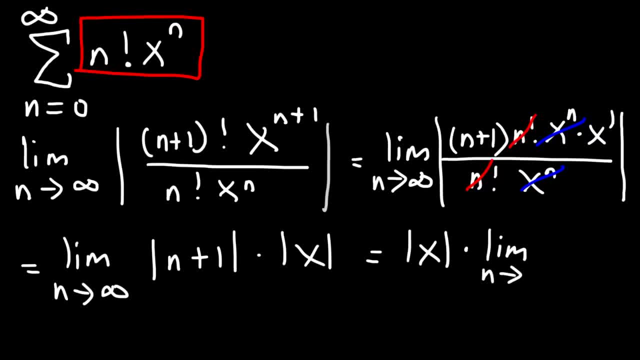 value of x times the limit, as n goes to infinity of n plus 1.. And then you can move this to plus 1.. And n is always positive, so we really don't need the absolute value symbol there. But as n goes to infinity, what happens to n plus 1?? n plus 1 also goes to infinity. 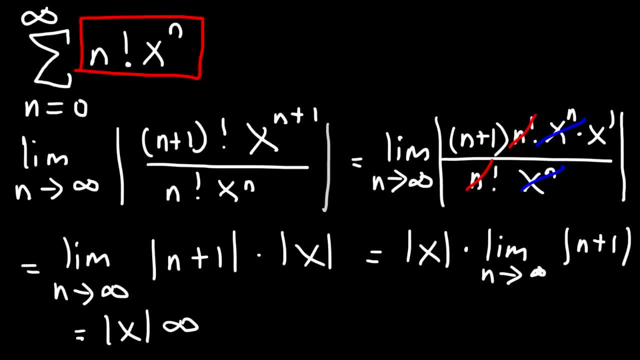 Now, what does this mean? The absolute value of x times infinity. That means that the limit goes to infinity. And what do we know when the limit goes to infinity? This is the second scenario. That means that the radius of convergence is 0, and the interval of convergence? 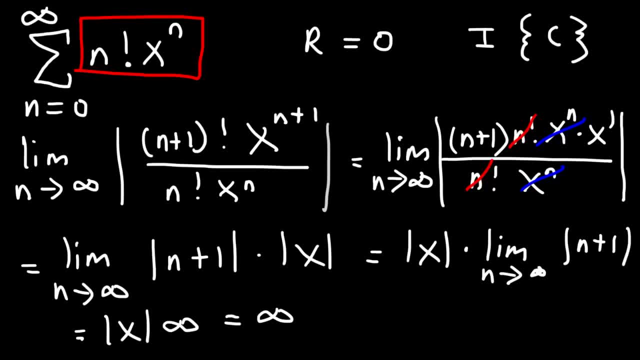 is our c value. So what is c? So at what number is the function centered at? There's no x minus c to the n, It's x minus 0 to the n, which is x to the n. So we could say that it's centered at 0.. 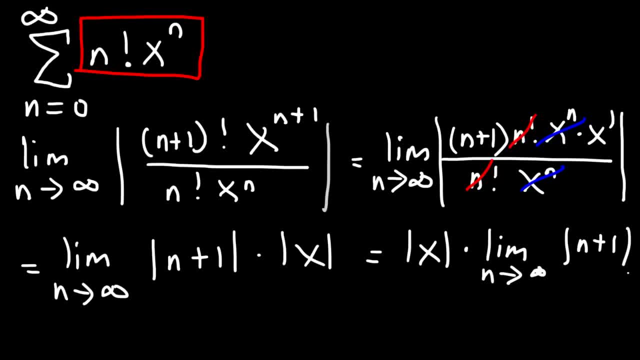 And n is always positive, so we really don't need the absolute value symbol there. But as n goes to infinity, what happens to n plus 1? N plus 1 also goes to infinity. Now what does this mean? The absolute value of x times infinity. 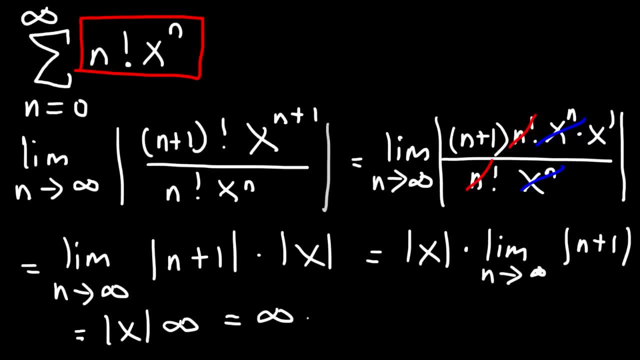 That means that the limit goes to infinity. And what do we know when the limit goes to infinity? This is the second scenario. That means that the radius of convergence is 0. And the interval of convergence is our c value. So what is c? 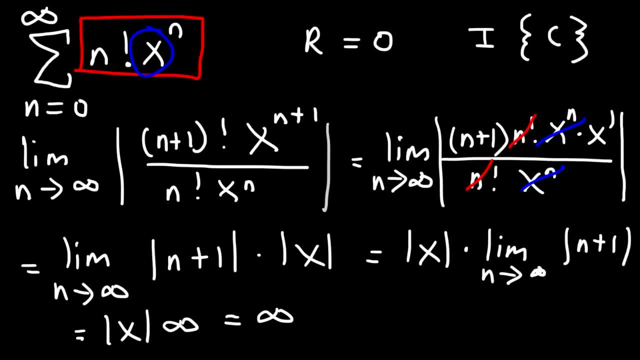 So at what number is the function centered at? There's no x minus c to the n. It's x minus 0 to the n, which is x to the n. So we can say that We can say that it's centered at 0.. 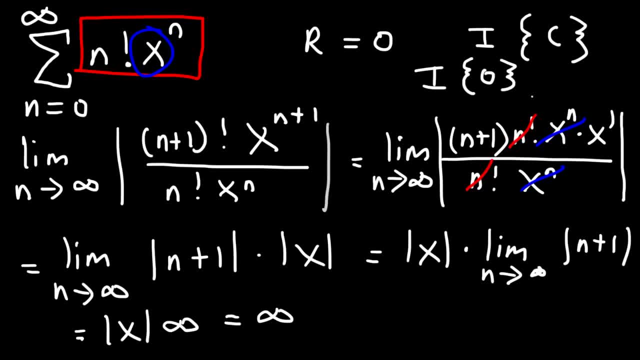 So when x is 0, it's going to converge. Now let's understand why. So if x is 0, we're going to have the limit as n approaches infinity. So if x is 0, we're going to have the limit as n approaches infinity. 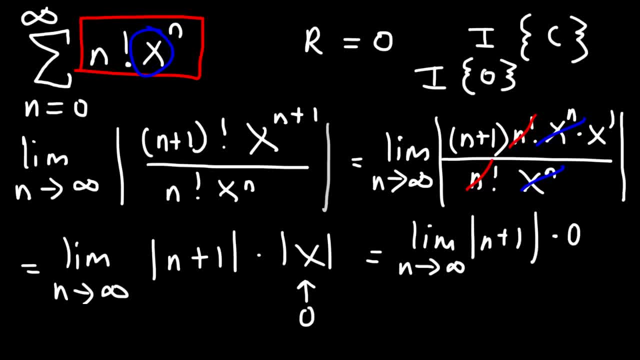 So if x is 0, we're going to have the limit, as n approaches infinity: n plus 1 times 0.. n plus 1 times 0 is 0. So then the whole limit will equal 0 if x is 0.. 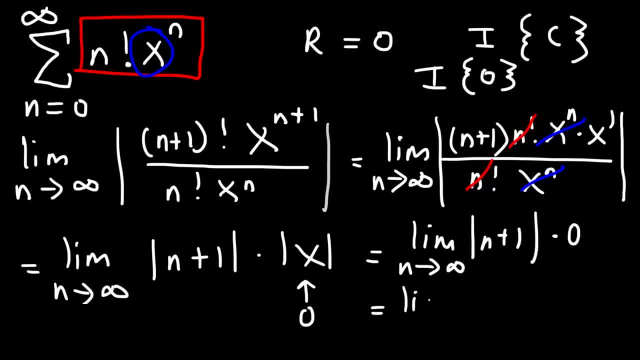 Now, if x is anything else but 0, let's say if x is a half, One, half times the limit, as n goes to infinity, of n plus 1.. Well, this is going to go to infinity. And if you multiply that by a half, 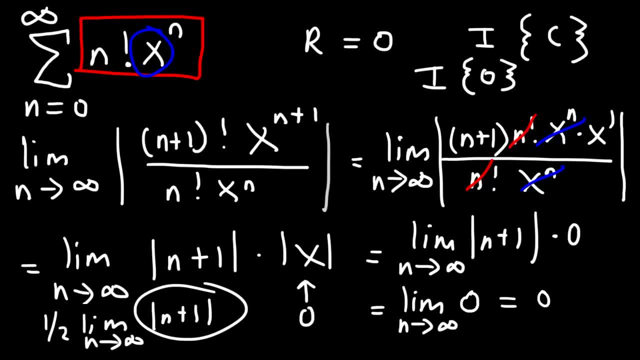 Then what's going to happen then? the whole thing is still going to be infinity. Half of infinity is infinity. So if x is any other value than 0, the limit will go to infinity, and so it's going to diverge. 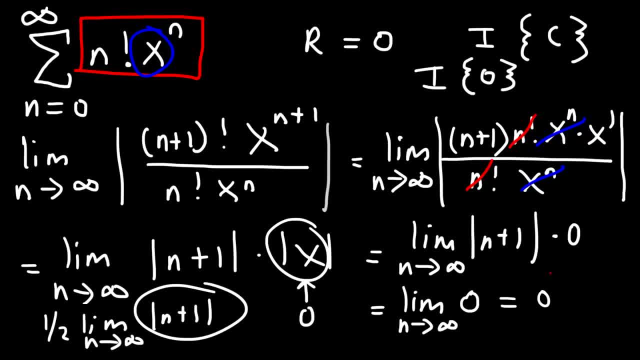 But when x is 0, then the limit goes to 0. And by the ratio test that's less than 1. It converges. So anytime you do the ratio test. if you get infinity as your output, that means that it's only going to converge. 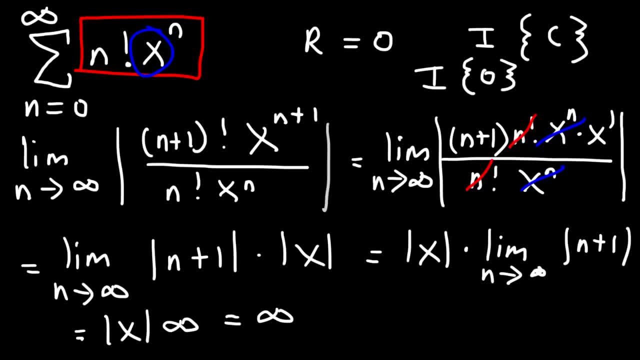 So what does this mean? The function is centered at 0.. So what does this mean? The function is centered at 0.. So when x is 0, it's going to converge. Now let's understand why. So if x is 0, we're going to have the limit as n approaches infinity: n plus 1 times 0.. 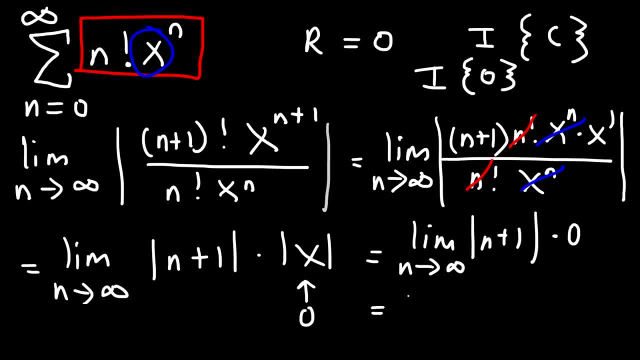 n plus 1 times 0 is going to converge. So then the whole limit will equal 0 if x is 0.. Now, if x is anything else but 0, let's say if x is a half, One, half times the limit, as n goes to infinity of n plus 1, well, this is going to go to infinity. 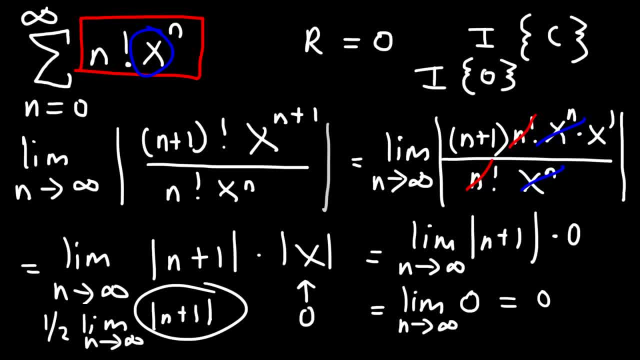 And if you multiply that by a half, then the whole thing is still going to be infinity. Half of infinity is infinity. So if x is any other value than 0, the limit will go to infinity, And so it's going to diverge. 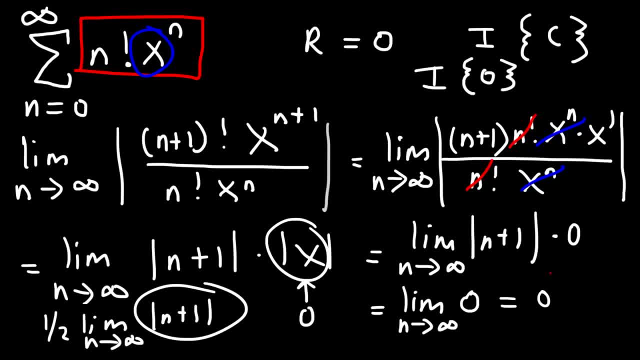 But when x is 0, then the limit goes to 0. And by the ratio test that's less than 1.. It converges So anytime you do the ratio test. if you get infinity as your output, that means that it's only going to converge when x is equal to c. 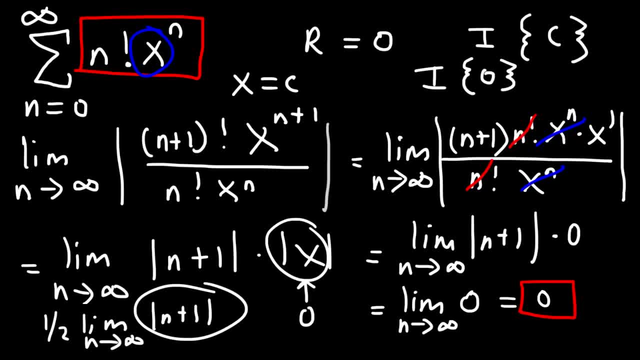 In this case, your c value is 0. So it converges when x is equal to 0, because the limit will go to 0. And so your answer for this situation is: the radius of convergence will be 0. And your interval of convergence is your c value. 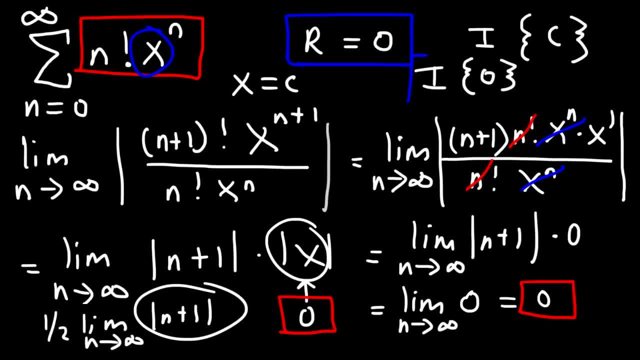 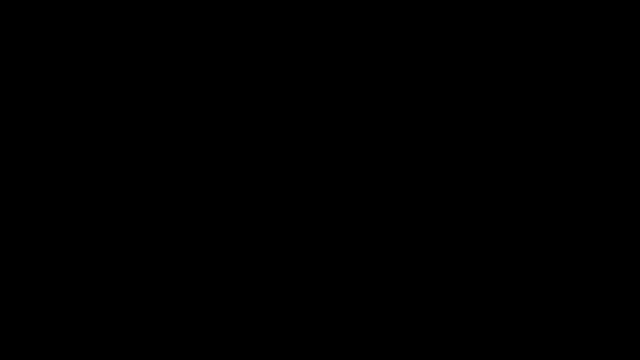 It's when x is equal to c. So in this case your interval of convergence is simply 0 because c is 0.. Now let's try another similar But a different example. So consider the series from 1 to infinity of n factorial times 2x minus 1 raised to the n factorial. 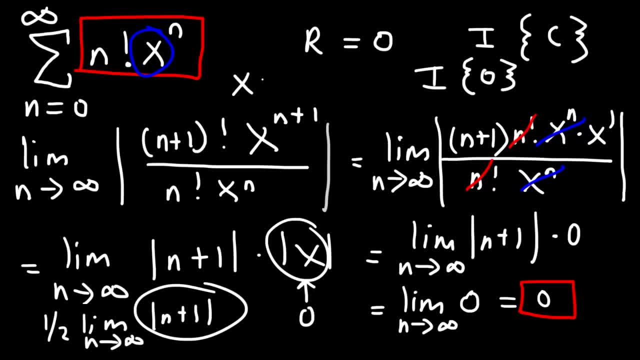 when x is equal to c. In this case, your c value is 0, so it converges when x is equal to 0, because the limit will go to 0. And so your answer for this situation is: the radius of convergence will be 0,. 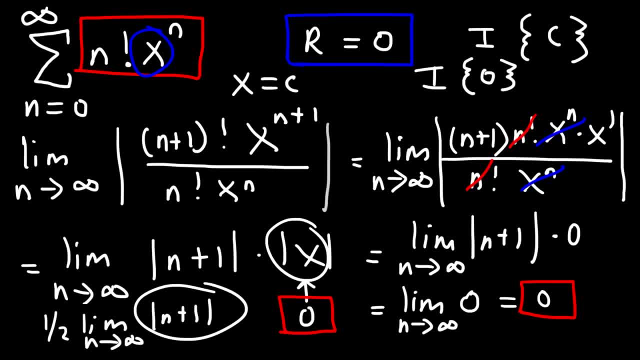 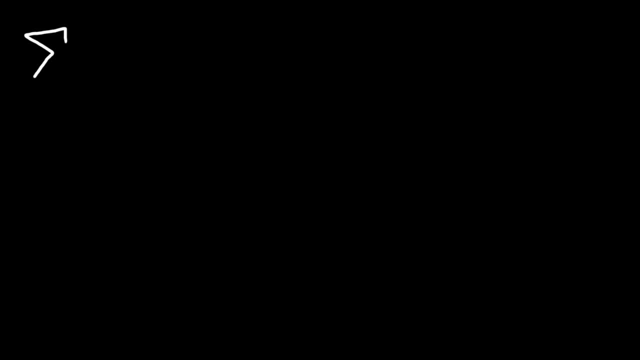 and your interval of convergence is your c value. It's when x is equal to c. So in this case, your interval of convergence is simply 0, because c is 0.. Now let's try another similar but different example. So consider the series from 1 to infinity. 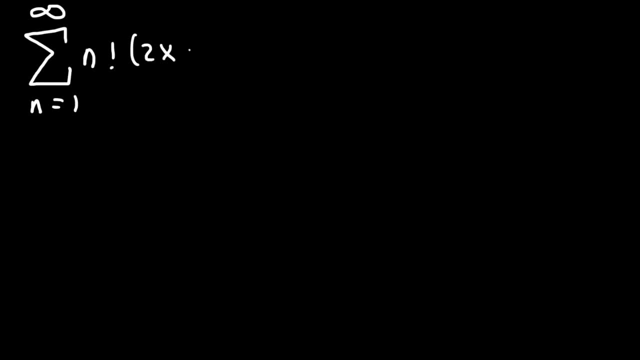 of n factorial times 2x minus 1, raised to the n factorial. So go ahead and determine the radius of convergence and the interval of convergence. So, as always, we're going to start with the ratio test. So u to the n plus 1,. 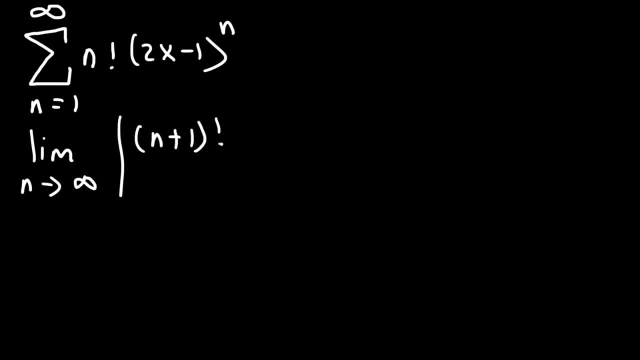 that's going to be n plus 1 factorial times 2x minus 1 to the n, plus 1 factorial divided by n. factorial times 2x minus 1 to the n. So that's our u sub n. So this is u sub n plus 1,. 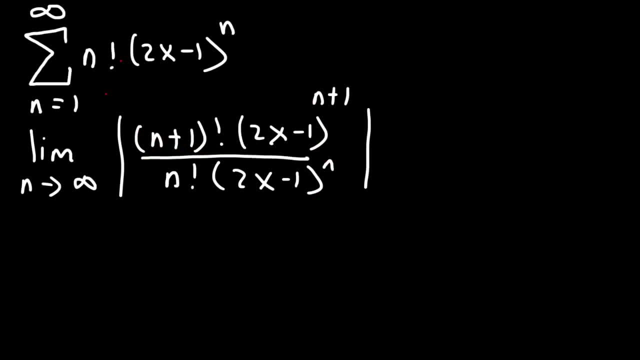 and this is the original u sub n expression that we see here. So go ahead and simplify it. So n plus 1 factorial, we can write that as n plus 1 times n factorial And 2x minus 1 to the n plus 1,. 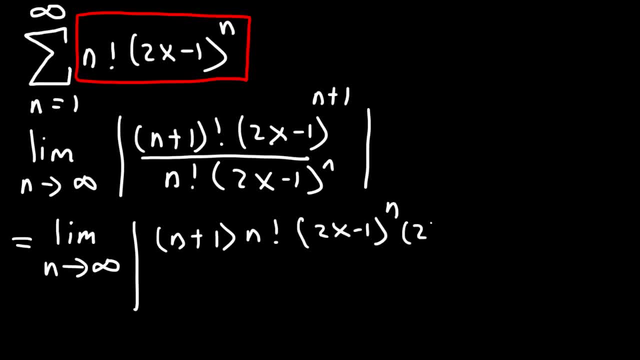 that's 2x minus 1 to the n times 2x minus 1 to the first power, And so we're going to simplify it, So we could cancel 2x minus 1 to the n and n factorial. And so now, 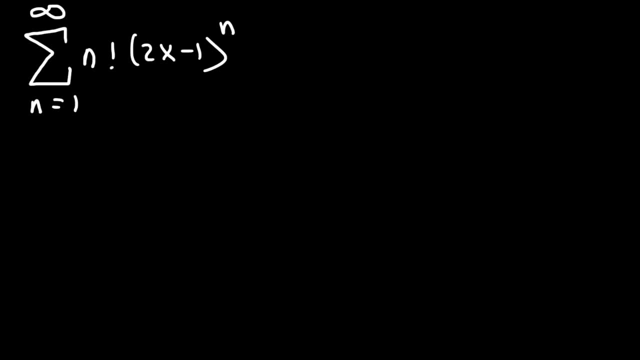 So go ahead and determine the radius of convergence and the interval of convergence. So, as always, we're going to start with the ratio test. So u to the n plus 1, that's going to be n plus 1 factorial Times. 2x minus 1 to the n plus 1 factorial 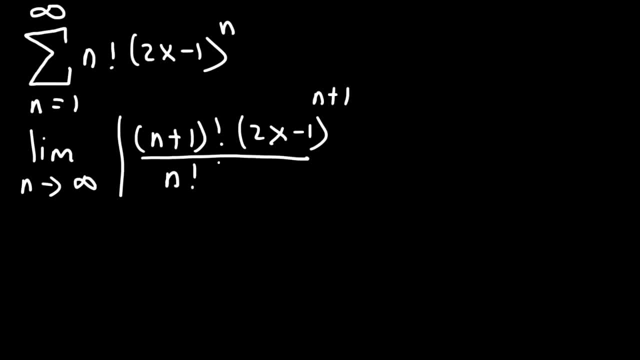 Divided by n factorial times, 2x minus 1 to the n. So that's our u sub n. So this is u sub n plus 1.. And this is the original u sub n expression that we see here. So go ahead and simplify it. 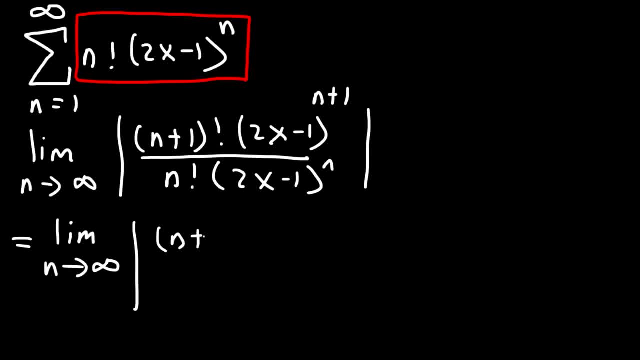 So n plus 1 factorial. we can write that as n plus 1 times n factorial And 2x minus 1 to the n plus 1, that's 2x minus 1 to the n times 2x minus 1 to the first power. 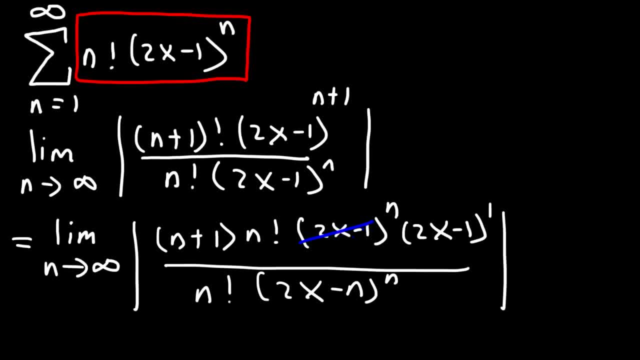 And so we could cancel 2x minus 1 to the n and n factorial. And so now what we have left over is the limit, as n goes to infinity, And then we have n plus 1 and also 2x minus 1.. 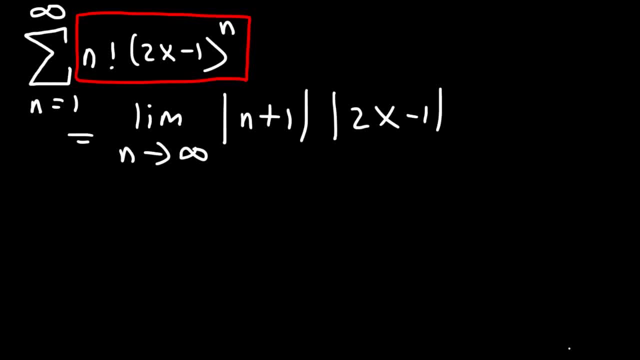 So what happens when n goes to infinity? n plus 1 also goes to infinity. So we're going to have infinity times 2x minus 1.. Now where is the power series centered at? What is our c value? To find our c value, we need to set the inside equal to 0.. 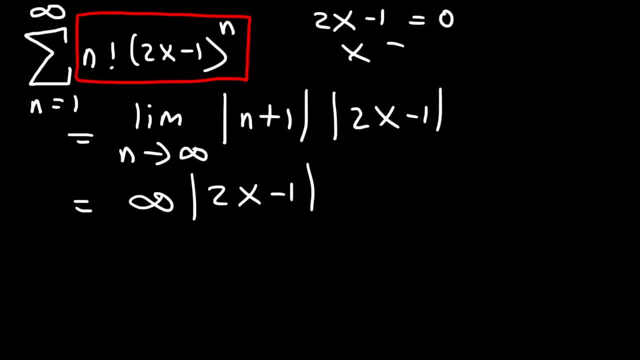 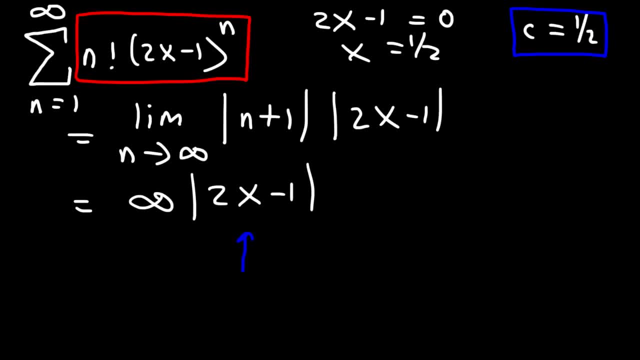 Let's say if x is 5.. If we plug it in here, 2 times 5 minus 1, that's 9.. 9 times infinity is infinity. So whenever x- let's say if x- does not equal 1, half infinity times, whatever that value is is going to be infinity. 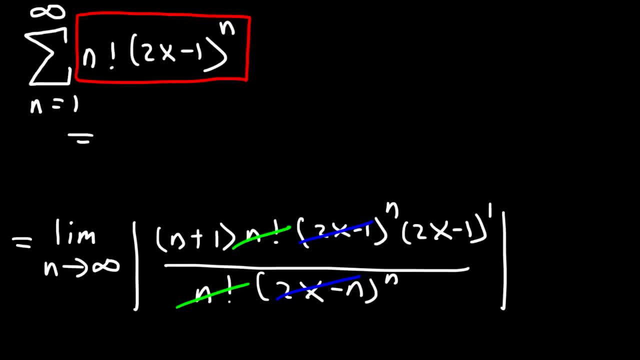 what we have left over is the limit, as n goes to infinity, and then we have n plus 1 and also 2x minus 1.. So we're going to cancel. so what happens when n goes to infinity, n plus 1 also goes to infinity. 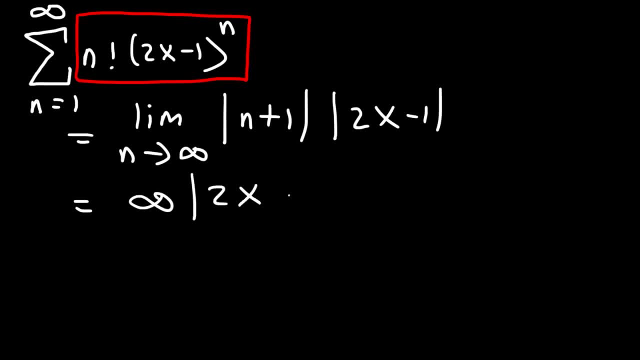 So we're going to have infinity times 2x minus 1.. Now where is the power series centered at? What is our c value? To find our c value, we need to set the inside equal to 0. So if you set 2x minus 1 equal to 0,. 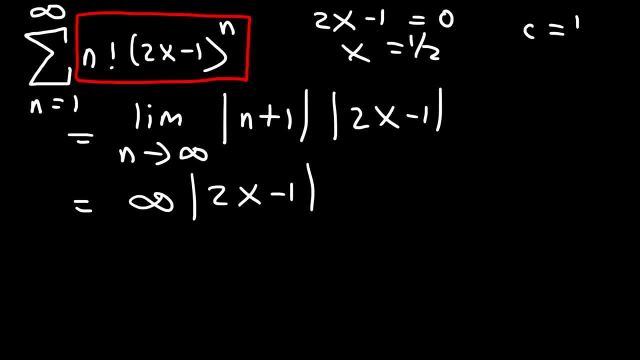 x is 1 half, And so c is 1 half. Now let's think about what we have. If x is anything but 1 half, it's going to diverge. Let's say, if x is 5. If we plug it in here, 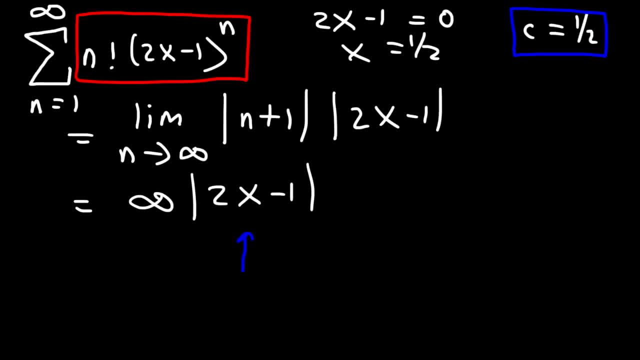 2 times 5 minus 1, that's 9.. 9 times infinity is infinity. So whenever x, let's say if x- does not equal 1, half infinity times, whatever that value is is going to be infinity, And so the series is going to diverge. 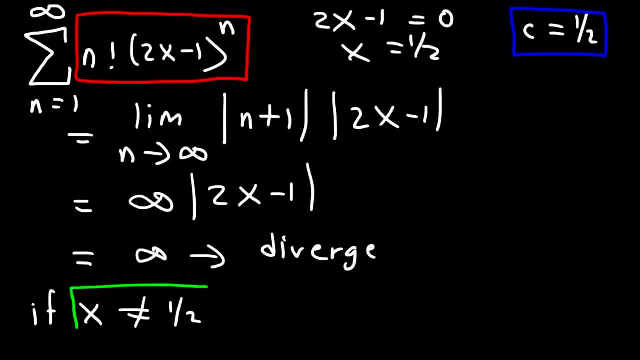 whenever x is anything but 1 half. What happens when x is 1 half? Well, if you plug in 1 half into this expression, we know we're going to get 0.. 2 times 1 half is 1 minus 1 is 0.. 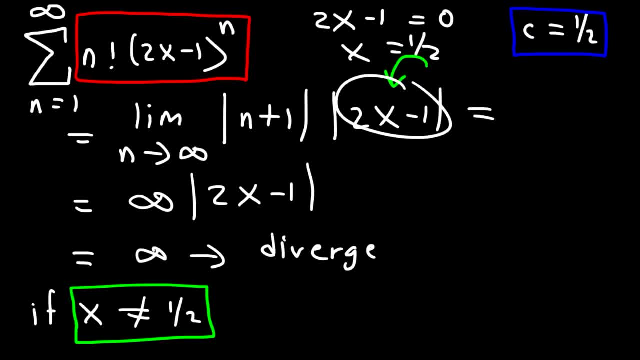 And so 0 times n plus 1 is 0. That's, the whole limit is going to go to 0, which means that the power series converges. So anytime you get infinity as a result, it's only going to converge. 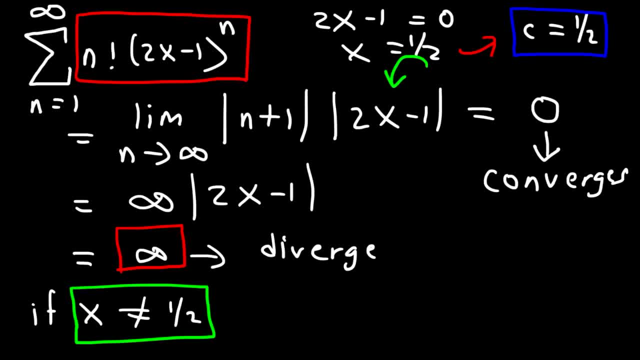 when x is equal to c. That is where the power series is centered at. So for this problem, the radius of convergence is 0, because there's only one number where this series converges, one x value. So the interval of convergence 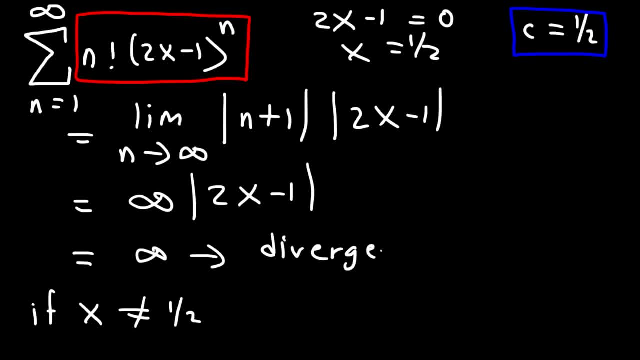 And so the series is going to diverge Whenever x is anything but 1 half. But what happens when x is a half? Well, if you plug in 1 half into this expression, we know we're going to get 0.. 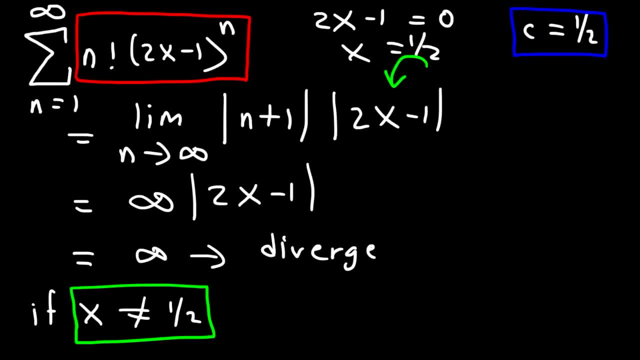 2 times a half is 1 minus 1 is 0. And so 0 times n plus 1 is 0. Thus the whole limit is going to go to 0, which means that the power series converges So anytime you get infinity as a result. 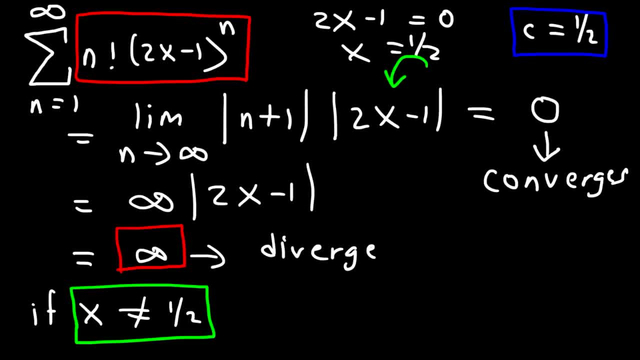 it's only going to converge when x is equal to c. That is where the power series is centered at. So for this problem, the radius of convergence is 0. Because there's only one number where this series converges, one x value. 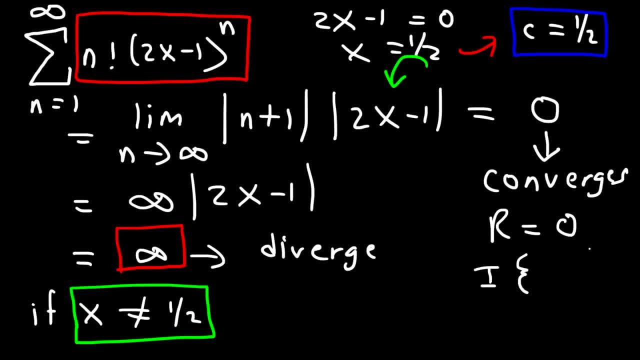 So the interval of convergence is x equals c, which is just 1 half. So it's not always 0. It depends on. It depends on where the power series is centered at. So this is the answer for this problem. So anytime you get infinity, the radius of convergence is 0.. 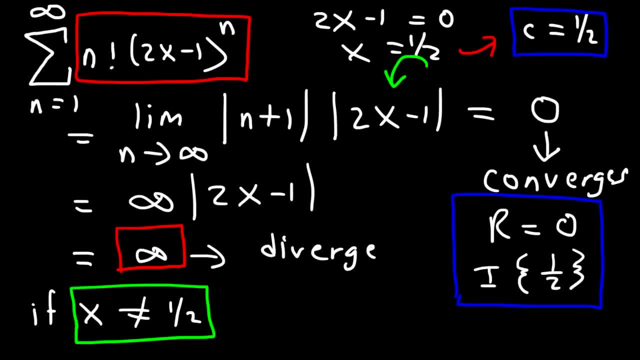 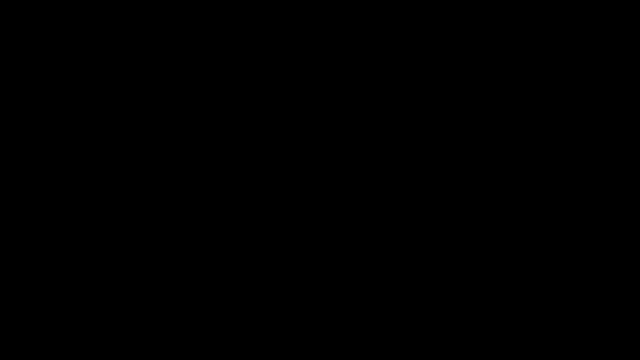 And the interval of convergence is where the power series is centered at, That's where x equals c. So you just put in your c value. Now let's work on another example problem. So let's say we have the power series from 0 to infinity. 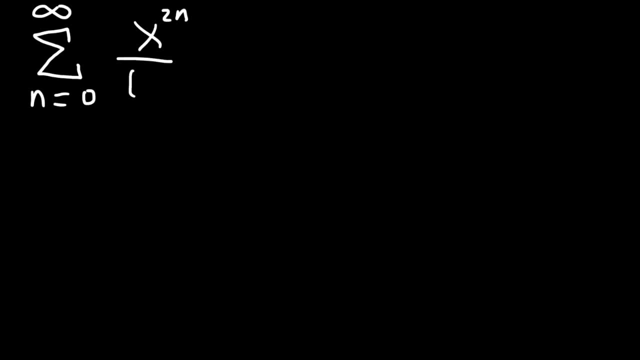 of x raised to 2n. divided by 2n, That's going to be x to the 2 times n plus 1.. So we're going to multiply 2n factorial by 2n factorial. So go ahead and work on this problem. 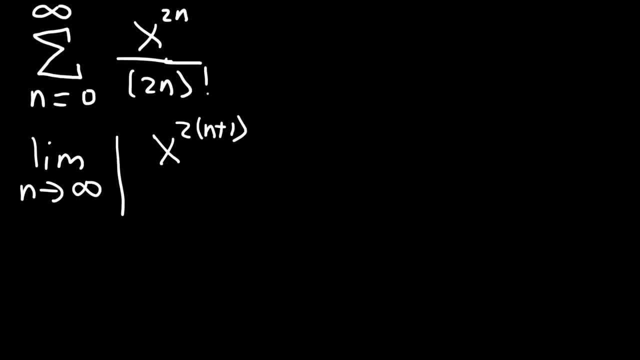 As always, let's start with the ratio test. So u sub n plus 1, that's going to be x to the 2 times n plus 1.. So replace n with n plus 1.. And then 2n factorial is going to become 2 times n plus 1 factorial. 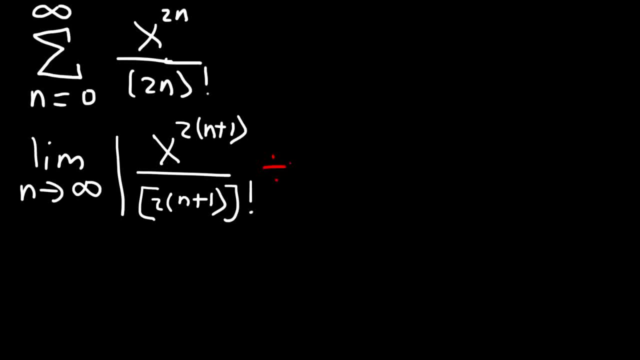 And then we're going to divide it by u sub n. So u sub n is just x to the 2n over 2n factorial. So right now what we have is x to the 2n plus 2.. And on the bottom we also have 2n plus 2 factorial. 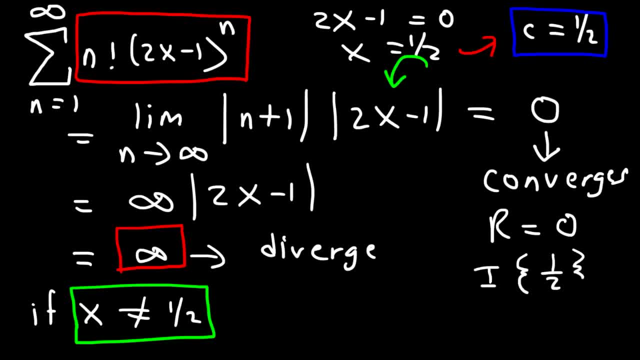 is x equals c, which is just 1 half. So it's not always 0. It depends on where the power series is centered at. So this is the answer for this problem. So anytime you get infinity, the radius of convergence is 0,. 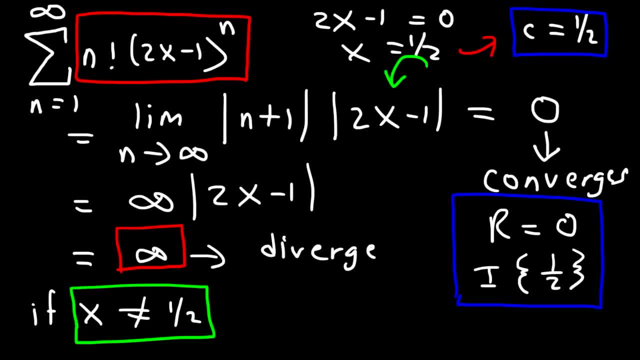 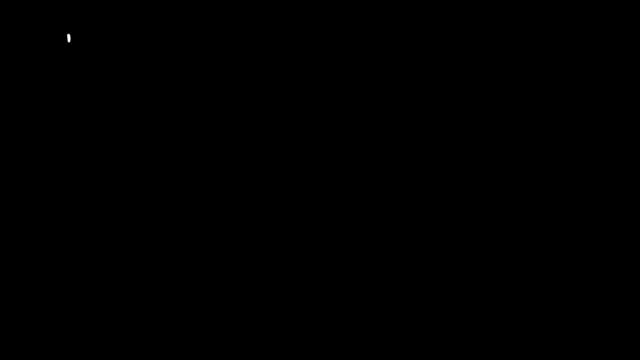 and the interval of convergence is where the power series is centered at, That's where x equals c. So you just put in your c value. Now let's work on another example problem. So let's say we have the power series from 0 to infinity. 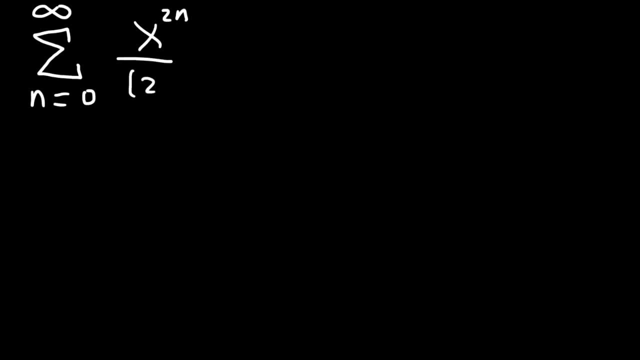 of x raised to 2n divided by 2n factorial. So go ahead and work on this problem. As always, let's start with the ratio test. So u sub n plus 1, that's going to be x to the 2 times n plus 1.. 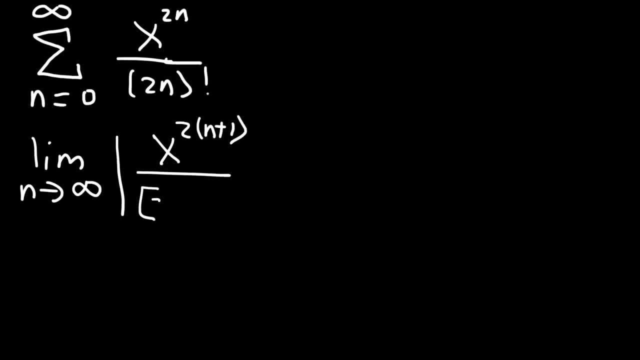 So replace n with n plus 1, and then 2n factorial is going to become 2 times n plus 1 factorial, And then we're going to divide it by u sub n. So u sub n is just x to the 2n over 2n factorial. 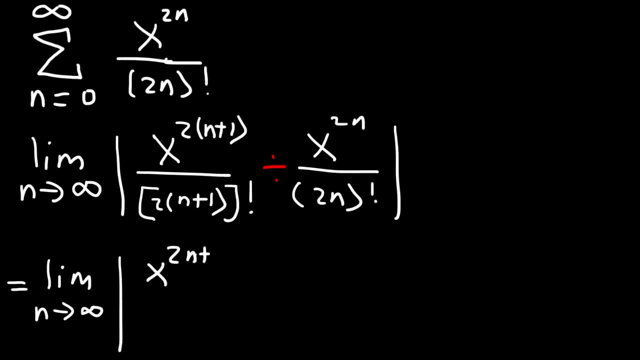 So right now what we have is x to the 2n plus 2.. And on the bottom we also have 2n plus 2 factorial, And then we're going to multiply it by the reciprocal of the other fraction. So this is going to be 2n factorial over x to the 2n. 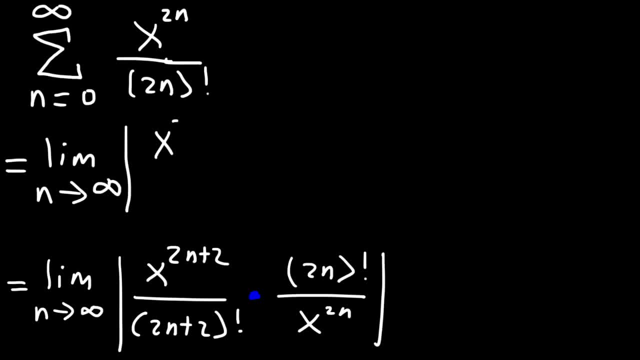 Now x to the 2n plus 2, we can say well x to the 2n plus 2.. We can say well x to the 2n plus 2.. We can separate that into x to the 2n times x squared. 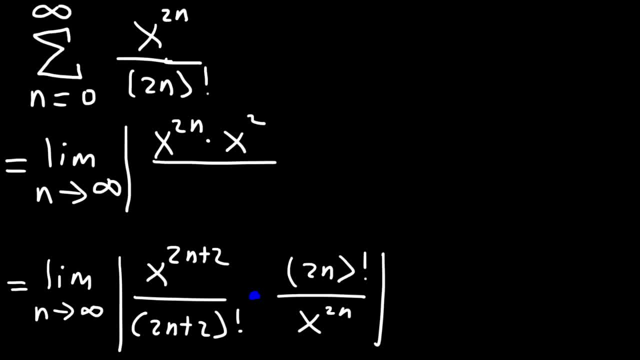 2n plus 2 factorial. So let's say we have 8 factorial, That's 8 times 7 times 6, and if you want to, you can stop at 5 factorial. So you have to keep subtracting 1 to get the next number. 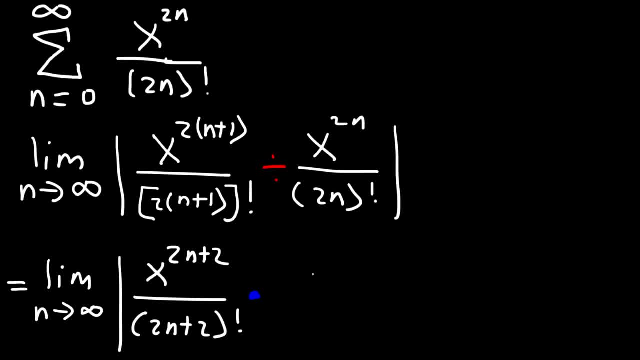 And then we're going to multiply by the reciprocal of the other fraction. So this is going to be 2n factorial over x to the 2n, Now x to the 2n plus 2. We can separate that into x to the 2n times x squared. 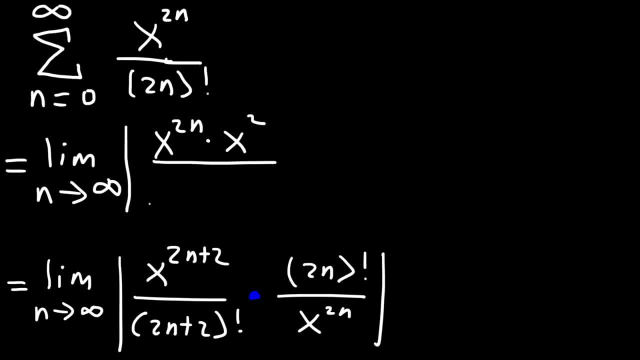 2n plus 2 factorial. So we're going to multiply by the reciprocal of the other fraction: 2n plus 2 factorial. So let's say, if you have 8 factorial, That's 8 times 7 times 6.. 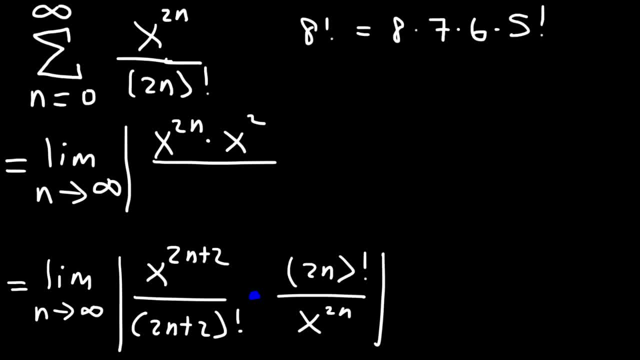 And if you want to, you can stop at 5 factorial. So you have to keep subtracting 1 to get the next number. So if we start with the first number- 2n plus 2,, to get to the next number we need to take 2n plus 2 and subtract it by 1.. 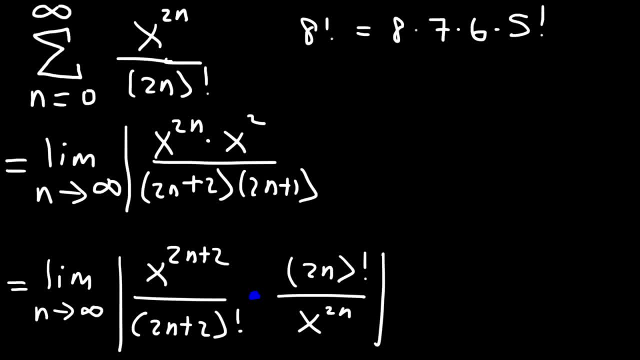 So it's going to be 2n plus 1.. And then if we subtract 2n plus 1 by 1, then we'll get 2n. We want to stop here because we can cancel it with the 2n factorial on top. 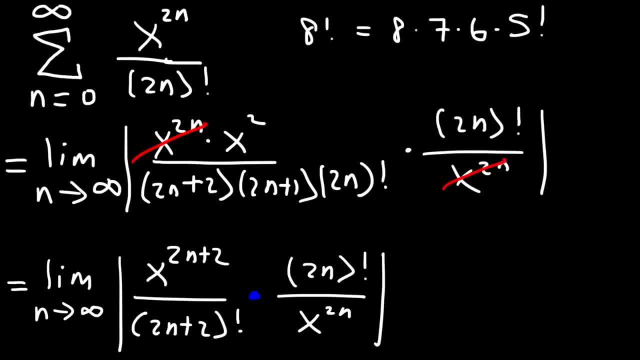 So now we can cancel x to the 2n and 2n factorial. So what we now have is the limit as n goes to infinity And then. And then we have: Since n is positive, I don't need an absolute value expression anymore. 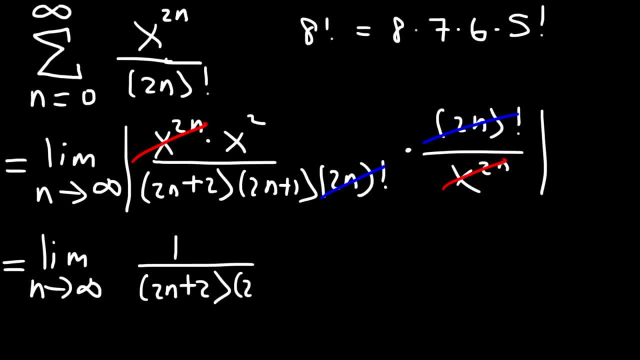 So this is going to be 2n plus 2, times 2n minus 1.. And then times x squared, which is also always positive. So what happens to this expression when n becomes very large, when it goes to infinity? As n goes to infinity, that fraction goes to 0.. 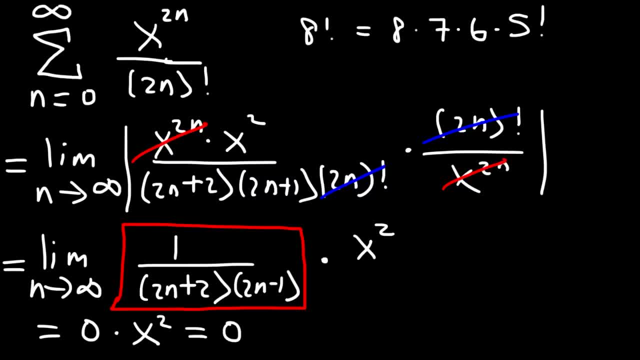 And so it's going to be 0 times x squared, which is 0 for all x. So, regardless of what x is, if it's 20, 1000, negative 50,, if you multiply by 0, it's going to be 0.. 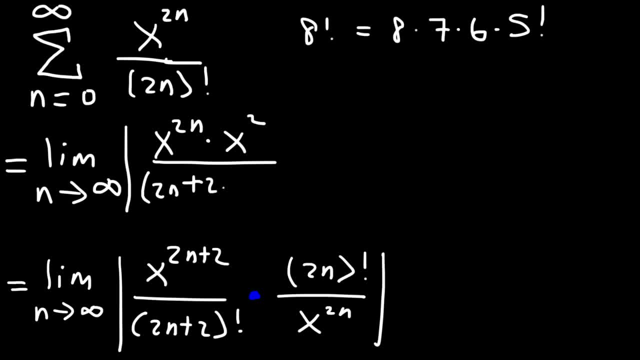 So if we start with the first number- 2n plus 2,, to get to the next number we need to take 2n plus 2 and subtract it by 1.. So it's going to be 2n plus 1.. 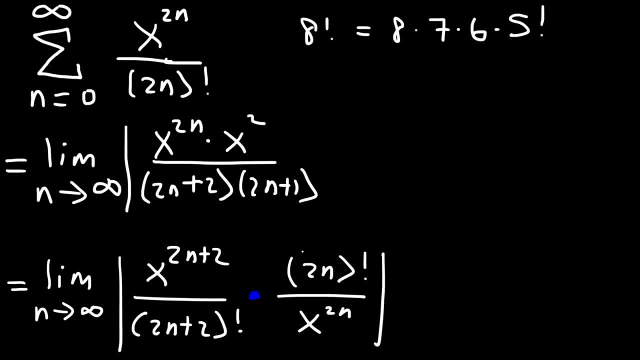 So that's 4 factorial. So we want to do the first equation. If we get the first equation, then we need to take 2n plus 2 and subtract it by 1.. And then if we subtract 2n plus 1 by 1, then we'll get 2n. 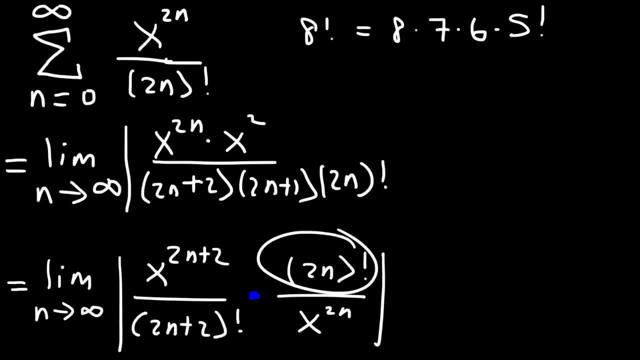 We want to stop here, because we can cancel it with the 2n factorial on top. So now we can cancel x to the 2n and 2n factorial. So what we now have is the limit, as n goes to infinity. And then we have: since n is positive, I don't need an absolute value expression anymore. 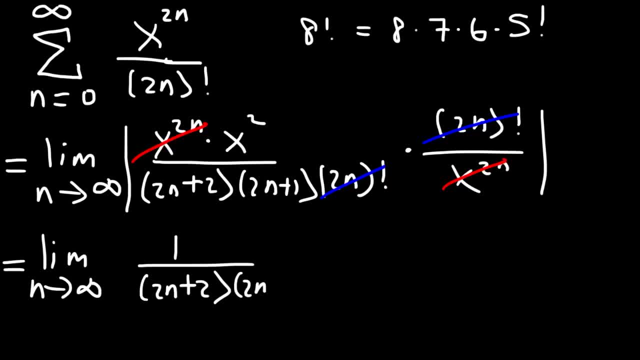 So this is going to be 2n plus 2, times 2n minus 1, and then times x squared, which is also always positive. So what happens if we subtract 2n? What happens to this expression when n becomes very large, when it goes to infinity? 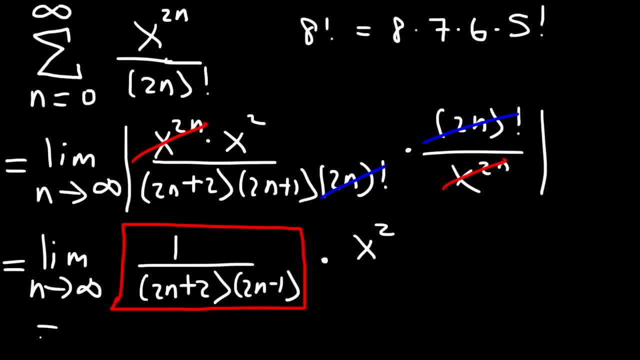 As n goes to infinity, that fraction goes to 0. And so it's going to be 0 times x squared, which is 0 for all x. So, regardless of what x is, if it's 20, 1,000, negative 50,, if you multiply it by 0, it's going to be 0.. 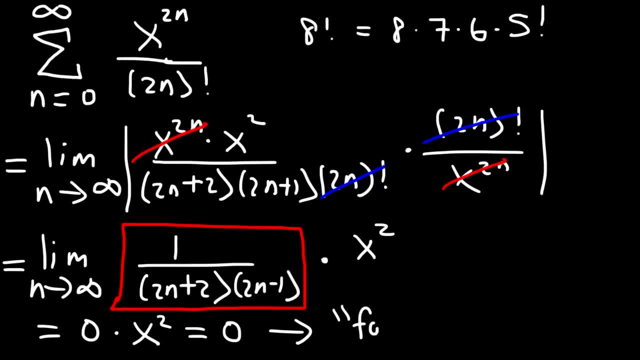 So this means that the series converges for all x values. So x is 0.. So x is 0. So any time you get an answer of 0 for the ratio test, that means that the radius of convergence is going to be infinity. 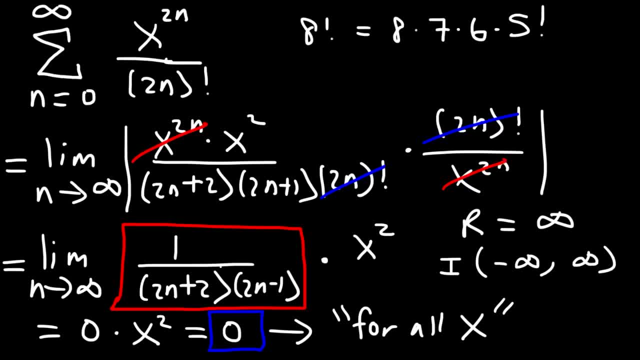 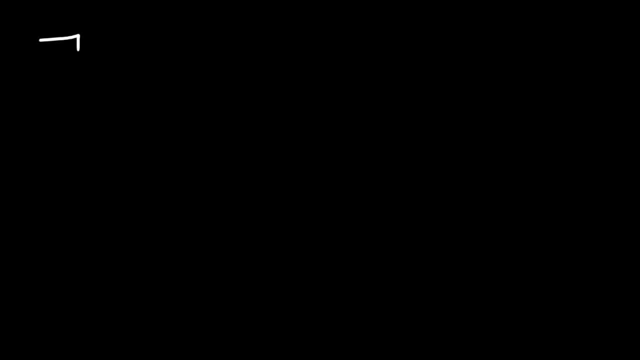 And the interval of convergence is negative: infinity to infinity. And so that's it for this problem. Now let's try another one. So consider the power series, the square root, n times x minus 1, raised to the n. Go ahead and try that one. 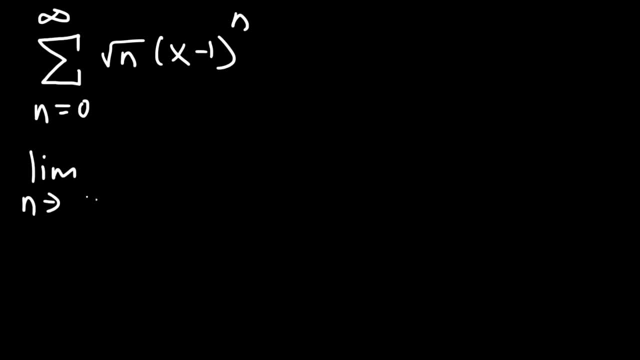 So once again, let's start with the ratio test. as always, u to the n plus 1, that's going to be the square root of n plus 1 times x minus 1, raised to the n plus 1, divided by the original expression u sub n. 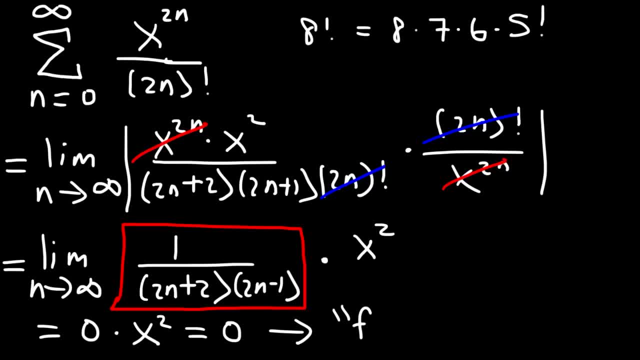 So this means that the series converges for all x values. So anytime you get an answer of 0 for the ratio test, that means that the radius of convergence is going to be infinity And the interval of convergence is going to be infinity. 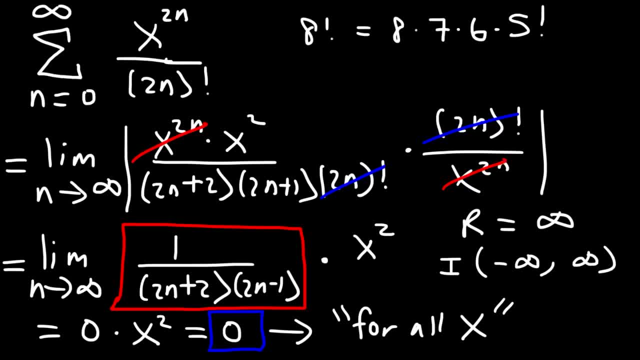 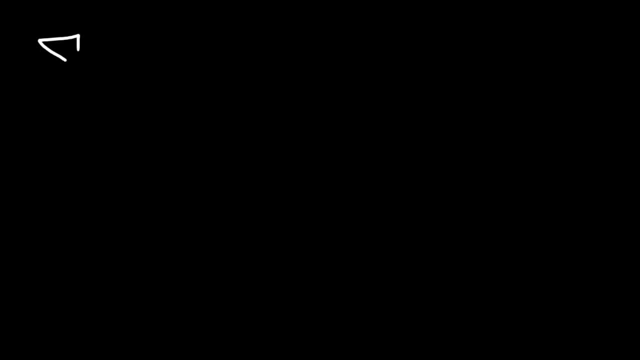 And the interval of convergence is negative: infinity to infinity. And so that's it for this problem. Now let's try another one. So consider the power series, the square root, n times x minus 1, raised to the n. Go ahead and try that one. 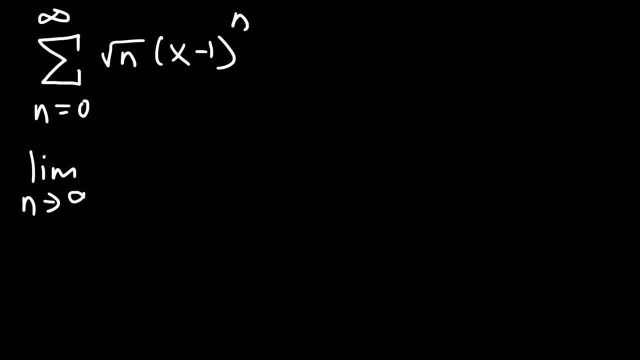 So once again, let's start with the ratio test. as always, u to the n plus 1, that's going to be the square root of n plus 1 times x minus 1, raised to the n plus 1, divided by the original expression u sub n. 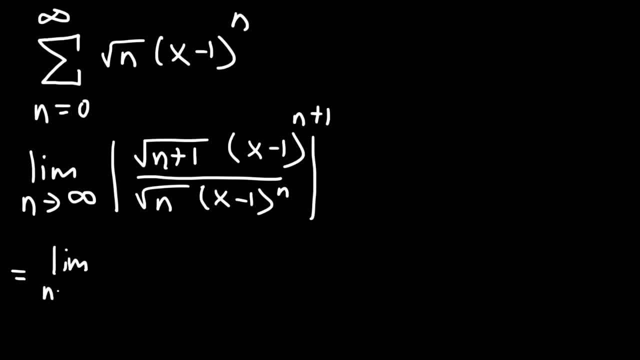 So this is equal to the limit, as n goes to infinity. Now, both of these expressions, they're inside the square root, so I can write it as one expression, The square root of n plus 1 over n. Now x minus 1 to the n plus 1, that's going to be x minus 1 to the n power times, x minus 1 to the first power. 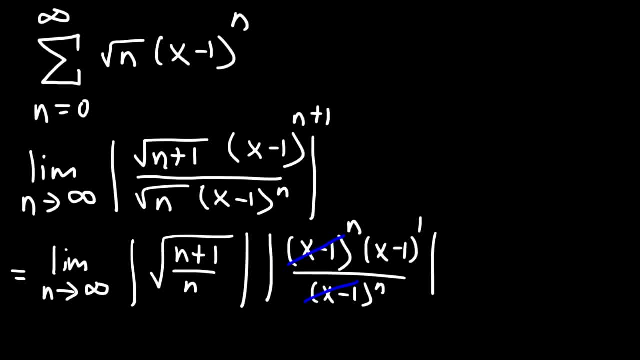 And so I can cancel these two. So what I have left over is the limit, as n goes to infinity. square root n plus 1 over the square root of n, or just I'm going to write it like this: and then times x minus 1.. 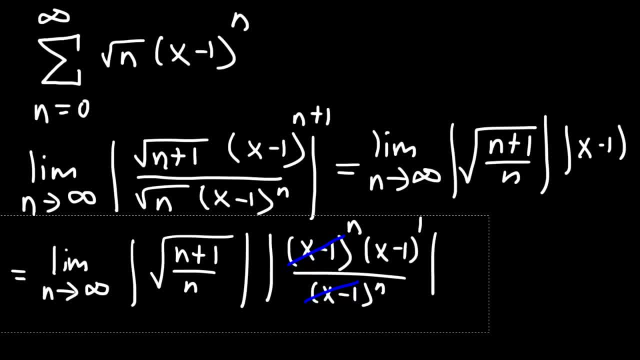 So what happens to n plus 1 over n when n goes to infinity, When n becomes very large, the 1 becomes insignificant. So you're going to get 1n over 1n, and so it's going to become 1.. 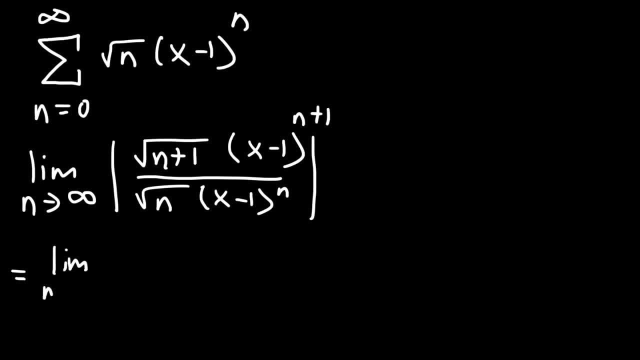 So this is equal to the limit, As n goes to infinity. now both of these expressions, they're inside the square root, So I can write it as one expression, the square root of n plus 1 over n. Now x minus 1 to the n plus 1, that's going to be x minus 1 to the n power times, x minus 1 to the first power. 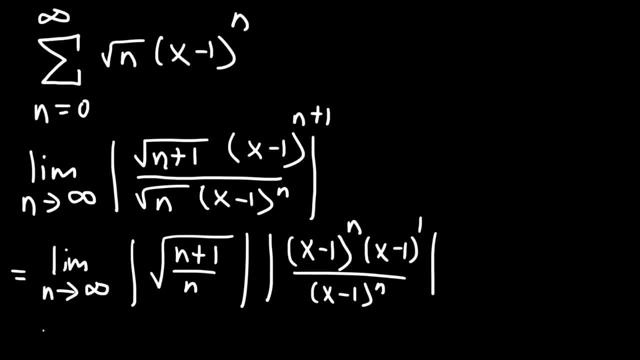 And so I can cancel these two. So what I have left over is the limit, as n goes to infinity. square root n plus 1 over the square root of n, or just I'm going to write it like this: and then times x minus 1.. 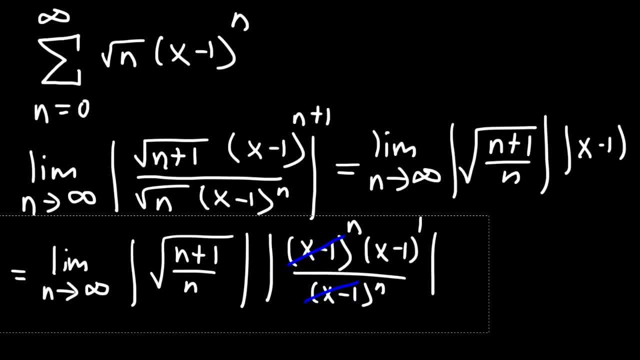 So what happens to n plus 1 over n when n goes to infinity, When n becomes very large, the 1 becomes insignificant. So you're going to get 1n over 1n, and so it's going to become 1.. 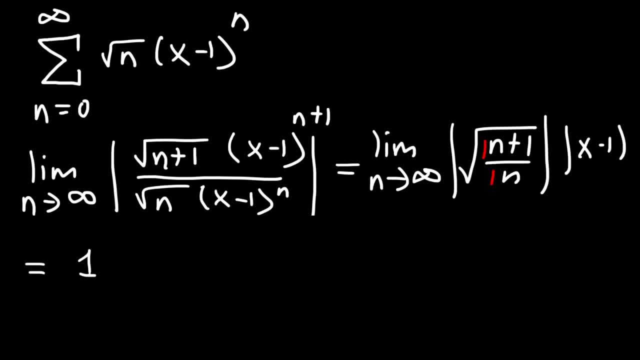 And the square root of 1 is 1.. So we're going to have 1 times x minus 1.. Now this is all still inside the absolute value expression. So we have the absolute value of x minus 1.. And whenever you have, let's say, an answer in terms of x after the ratio test. 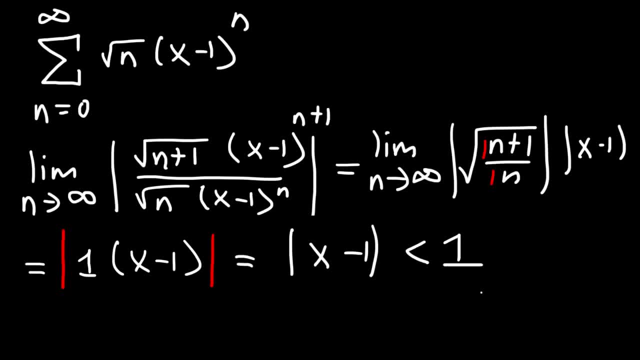 set that answer less than 1, because you want to find out for what values of x it converges. So we can rewrite this expression. We can get rid of the absolute value expression by saying that x minus 1 is less than 1,. 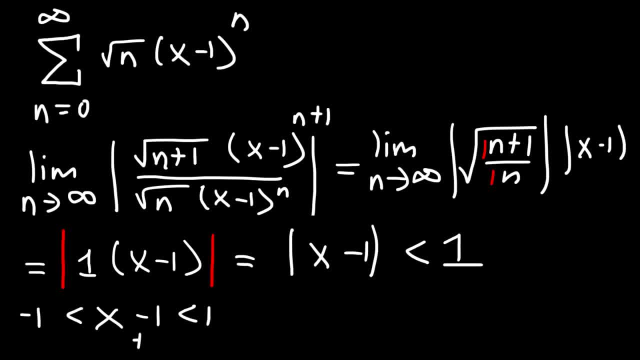 but greater than negative 1.. So now, if we add 1 to all three sides, we can see that x is less than 1 plus 1,, which is 2, but greater than negative 1 plus 1,, which is 0.. 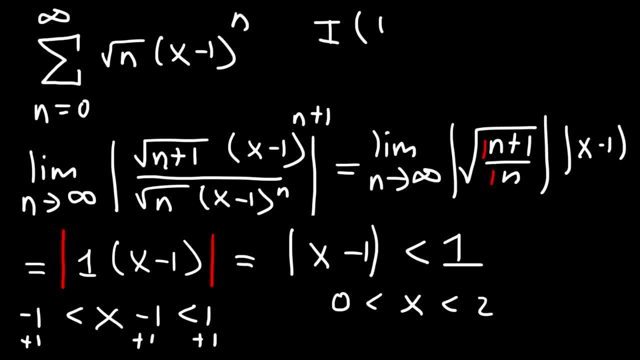 So, therefore, the interval of convergence is from 0 to 2, or at least it appears that way. We still need to check the endpoints, so we can adjust it shortly Now. what is the radius of convergence? If you recall once you have this form? 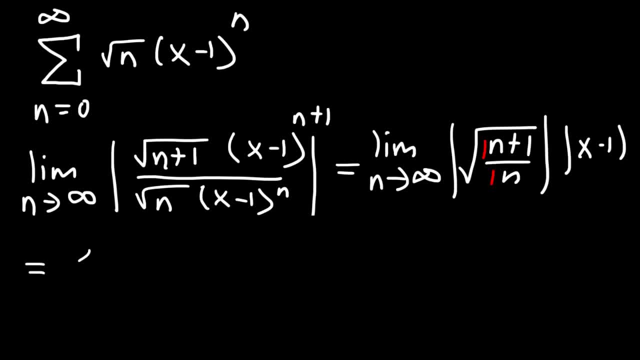 And the square root of 1 is 1.. So we're going to have 1 times x minus 1.. Now, this is all still inside the absolute value expression. So we have the absolute value of x minus 1.. And whenever you have, let's say, an answer in terms of x, 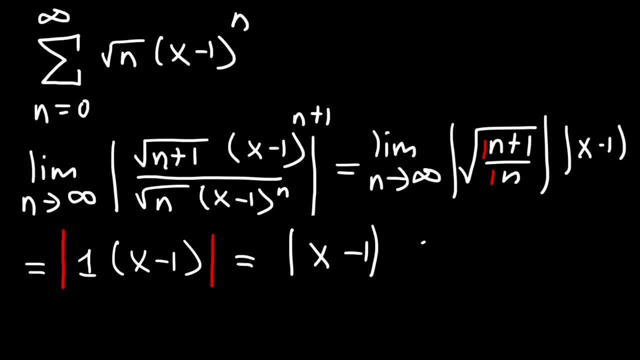 after the ratio test set that answer less than 1, because you want to find out for what values of x it converges. So we can rewrite this expression. we can get rid of the absolute value expression by saying that x minus 1 is less than 1,. 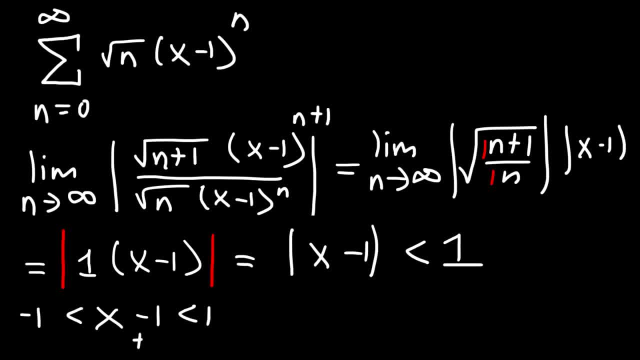 but greater than negative 1.. So now, if we add 1 to all three sides, we can see that x is less than 1 plus 1,, which is 2, but greater than negative 1 plus 1,, which is 0.. 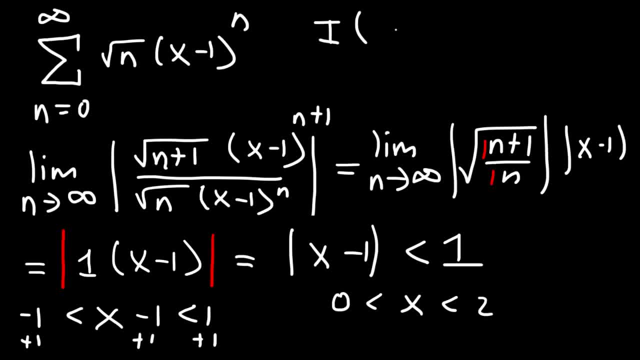 So, therefore, the interval of convergence is from 0 to 2, or at least it appears that way. We still need to check the endpoints, so we can adjust it shortly Now. what is the radius of convergence? If you recall once you have this form? 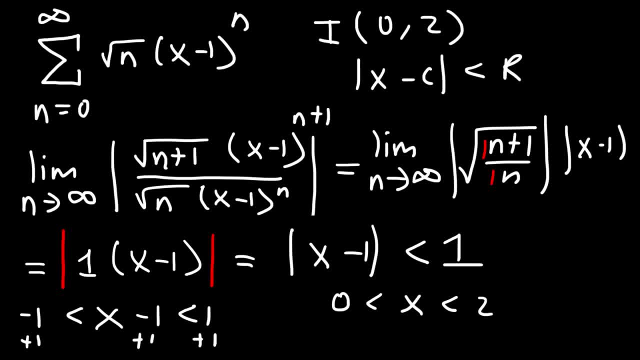 if there's no number in front of the absolute value, then whatever number you see here is the radius of convergence. In this case it's 1.. And you can see that we have x minus 1 or x minus c, so c is 1 for this example. 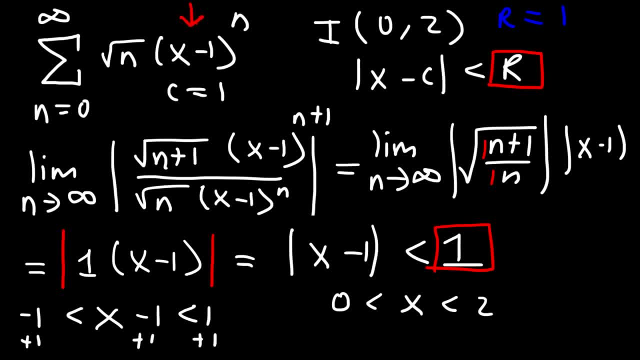 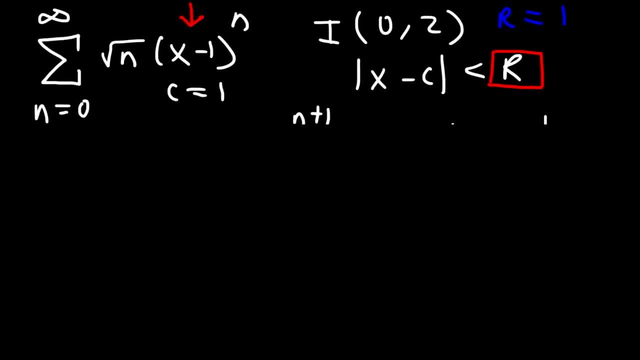 It's centered at 1.. And you can see it here too. That's x minus c. Now let's check the endpoints. So let's start with 0.. We're going to see if it converges when x is equal to 0.. 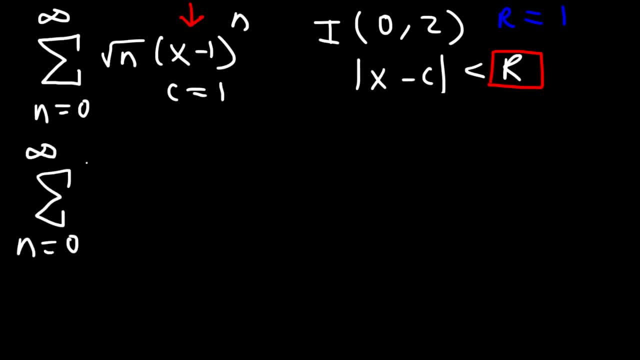 So, starting with the power series, replace x with 0.. So we're going to have the square root of n times 0 minus 1 to the n power, which is 1 to the n power or negative 1 to the n power. 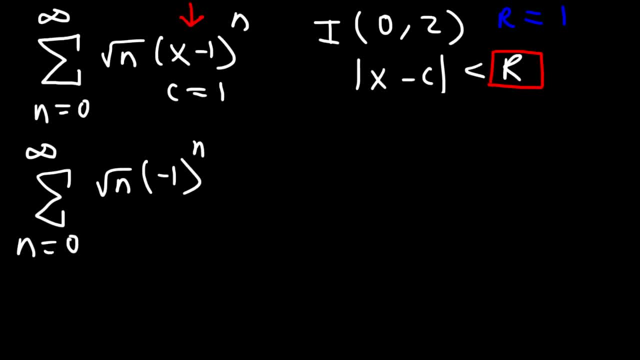 So does the series converge in this form? What would you say? Well, a simple way is to try the divergence test: The limit as n goes to infinity for the square root of n times negative 1 to the n power As n goes to infinity. 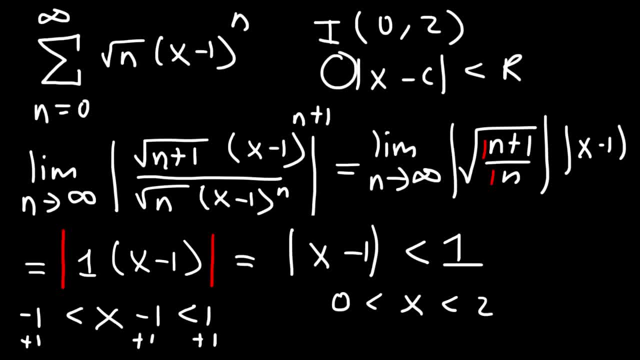 if there's no number in front of the absolute value, then whatever number you see here is the radius of convergence. In this case it's 1.. And you can see that we have x minus 1 or x minus c, So c is 1 for this example. 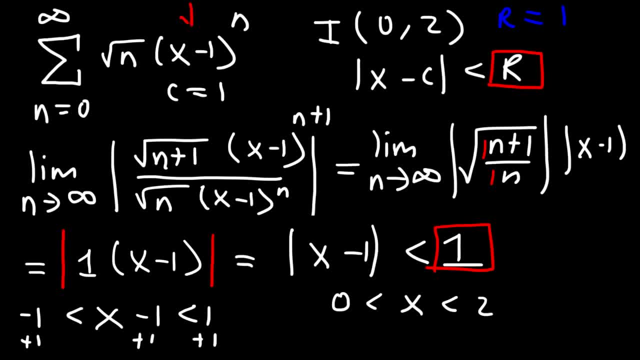 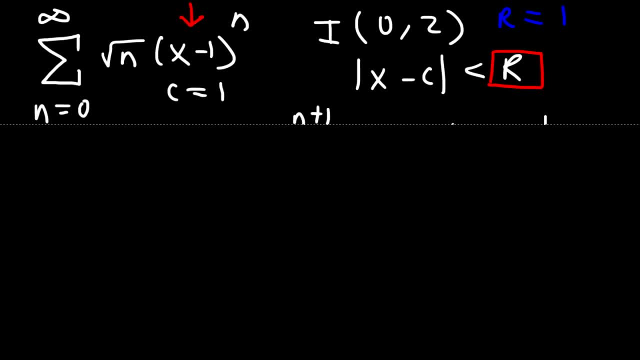 It's centered at 1.. And you can see it here too. That's x minus c. Now let's check the endpoints. So let's start with 0.. We're going to see if it converges when x is equal to 0.. 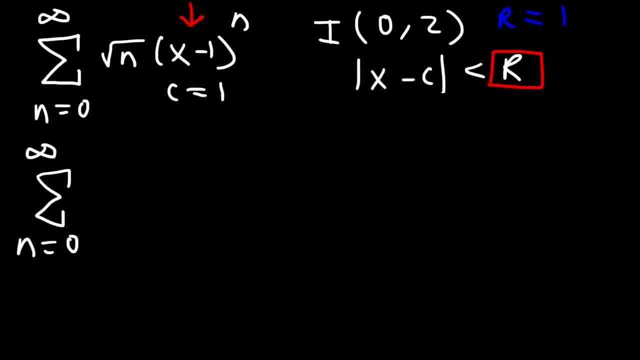 So, starting with the power series, replace x with 0.. So we're going to have the square root of n times 0 minus 1 to the n power or negative 1 to the n power. So does the series converge in this form? 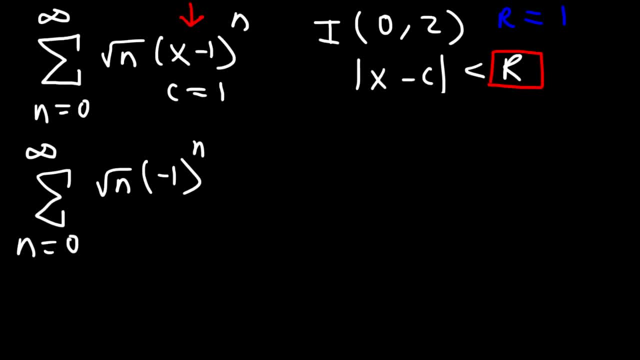 What would you say? Well, a simple way is to try the divergence test: The limit as n goes to infinity, for the square root of n, times negative 1 to the n power As n goes to infinity, the square root of n. what's going to happen to that? 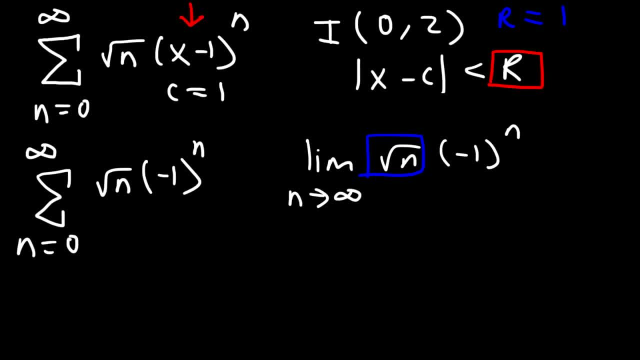 That's going to be the square root of infinity, which is basically infinity, And then the only difference is it's going to alternate in sine, It's going to switch from negative 1 to 1, so our answer is going to be: 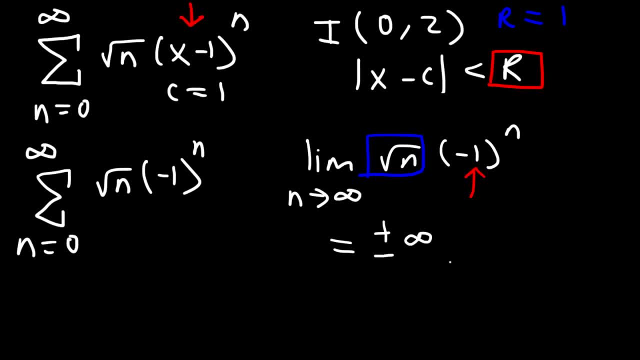 positive infinity, negative infinity and so forth. It's always going to alternate. So we could say that the limit doesn't exist because it doesn't equal one value. Sometimes it will equal positive infinity, Sometimes it will equal negative infinity. Now, if the limit doesn't exist, 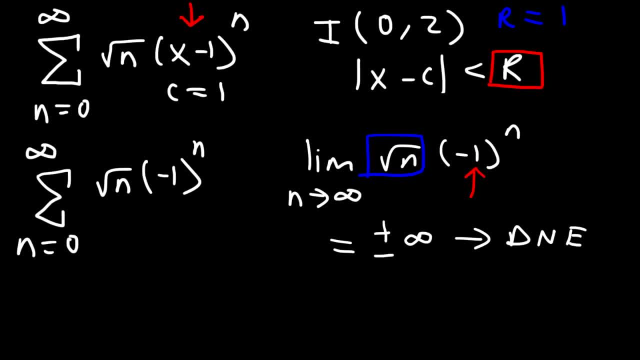 then we say that according to the divergence test, the limit diverges. So if it diverges, then it doesn't converge when x is equal to 0. So we're not going to include 0 as an endpoint, So we're going to leave it with parentheses. 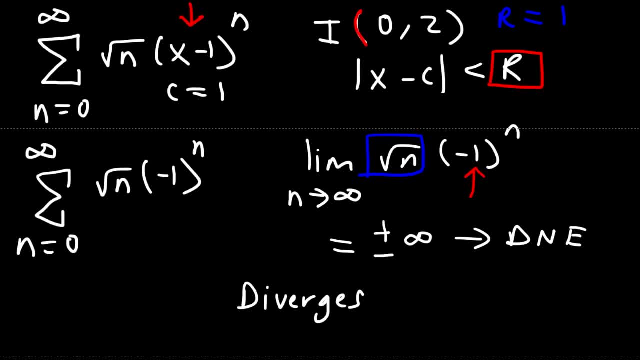 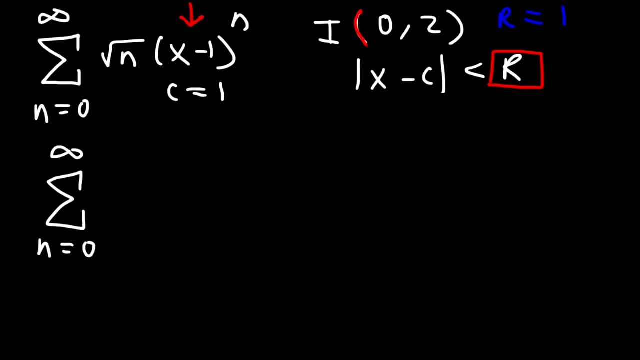 It doesn't include 0.. We're not going to use brackets. If it converged, then we would use a bracket at that endpoint. So now let's test the other endpoint, when x is 2.. So we're going to have the square root of n. 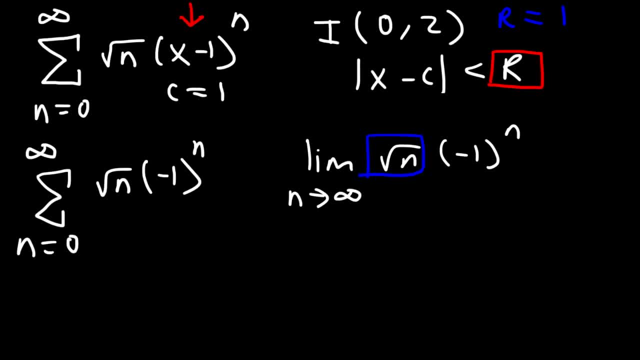 the square root of n. what's going to happen to that? That's going to be the square root of infinity, which is basically infinity, And then the only difference is it's going to alternate in sign, It's going to switch from negative 1 to 1,. 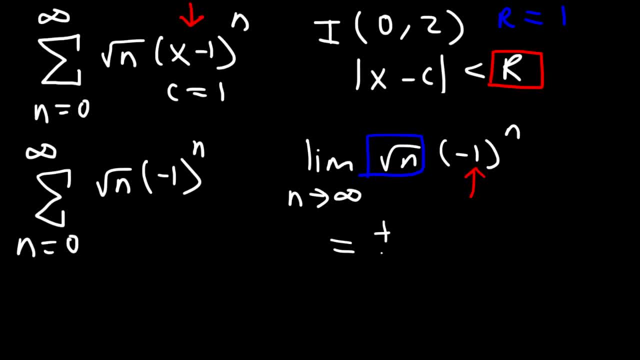 so our answer is going to be positive infinity, negative infinity and so forth. It's always going to alternate. So we could say that the limit doesn't exist because it doesn't equal one value. Sometimes it will equal positive infinity, sometimes it will equal negative infinity. 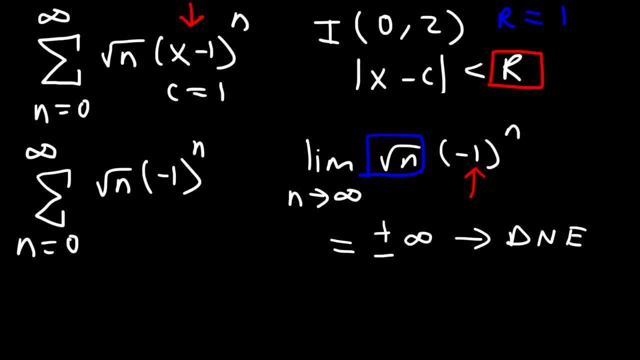 Now, if the limit doesn't exist, then we say that according to the divergence test, the limit diverges. So if it diverges, then it doesn't converge when x is equal to 0. So we're not going to include 0 as an endpoint. 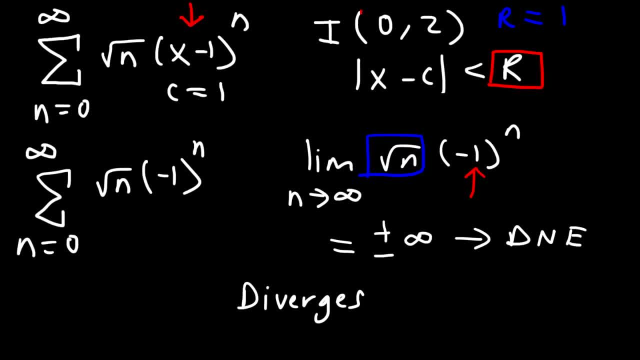 So we're going to leave it with parentheses. It doesn't include 0.. We're not going to use brackets. If it converged, then we would use a bracket at that endpoint. So now let's test the other endpoint, when x is 2.. 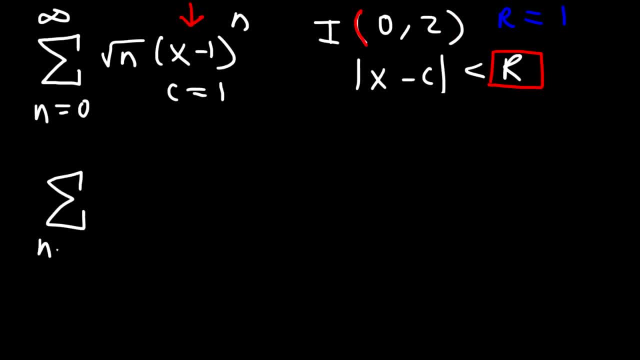 So we're going to have the square root of n times 2 minus 1 to the n power, which is 1 to the n and 1 to the n is just 1, so this is what we have Now using the divergence test. 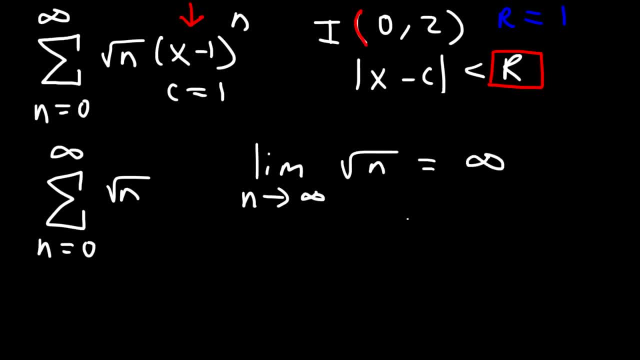 this is going to go to infinity, so it still diverges. So 2 should not be included in the interval of convergence. Now let's plot the interval of convergence for this problem. So it starts at 0, and it goes to 2.. 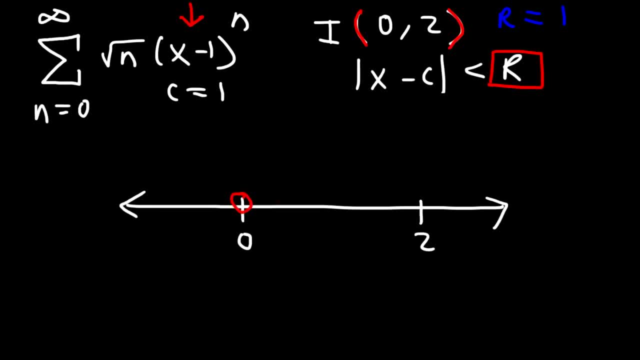 Now it doesn't include 0 or 2, so we're going to have an open circle at those points. So anywhere in this region where x is between 0 and 2, the power series will converge. Now the power series is centered at 1,. 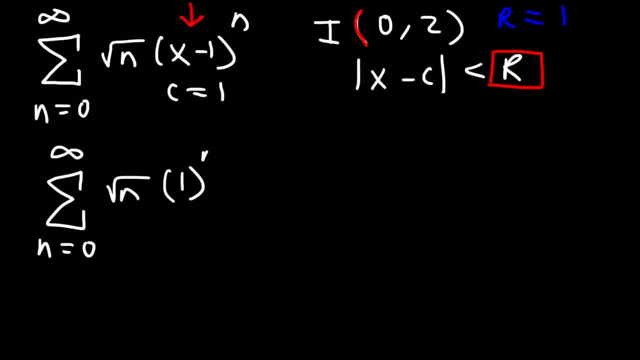 times 2 minus 1 to the n, power, which is 1 to the n and 1 to the n, is just 1, so this is what we have Now using the divergence test. this is going to go to infinity. 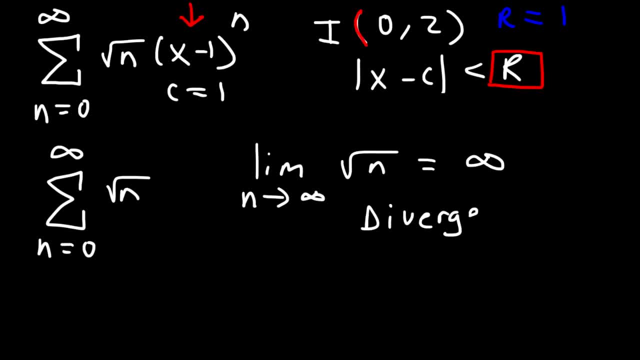 so it still diverges. So 2 should not be included in the interval of convergence. Now let's plot. Let's plot the interval of convergence for this problem. So it starts at 0, and it goes to 2.. Now it doesn't include 0 or 2,. 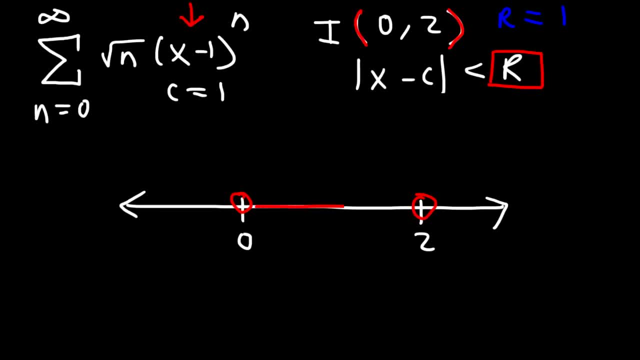 so we're going to have an open circle at those points. So anywhere in this region where x is between 0 and 2, the power series will converge. Now the power series is centered at 1,, so this is the c-value. 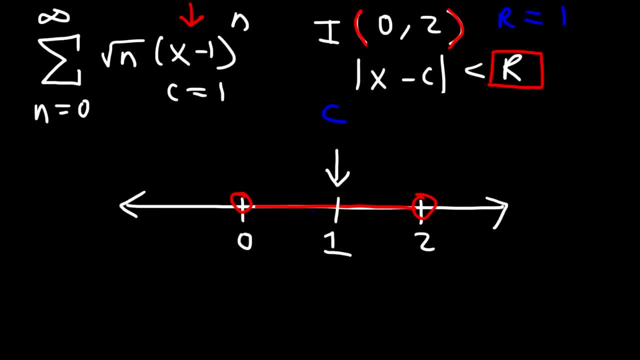 And the radius of convergence is basically the distance from the center to the end of the interval. So this distance is r, And so we can see why r is 1, because between 0 and 1, that distance is approximately 1.. 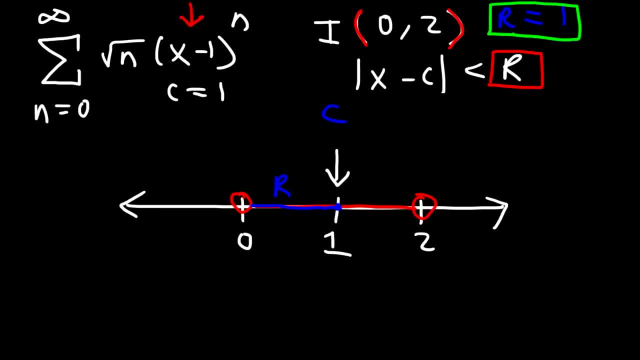 So r is typically 1 half of the length of the interval. So if it goes from 0 to 2,, then if you take the difference between 0 and 2, which is 2, divided by 2, that's your radius of convergence. 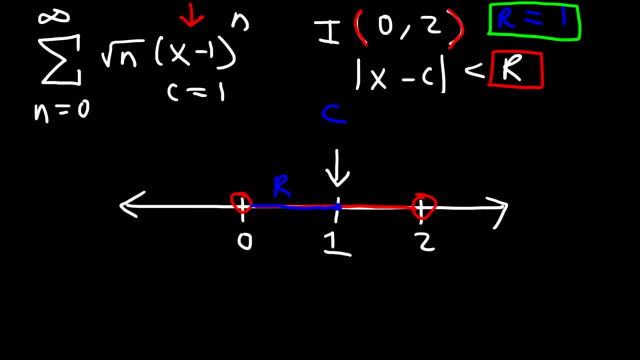 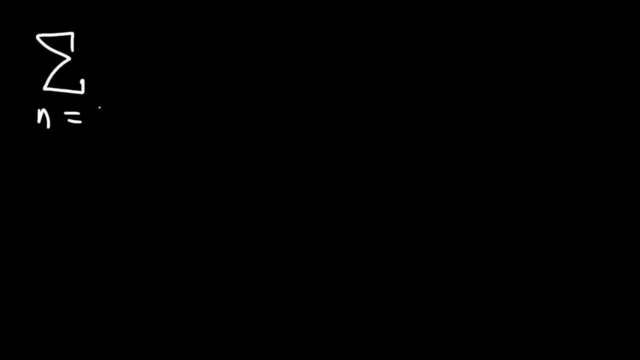 And so that's it for this problem. Hopefully this gives you a better understanding of it. Let's try this power series. Let's say it's x minus 3 to the n divided by n. So let's start with the ratio test. 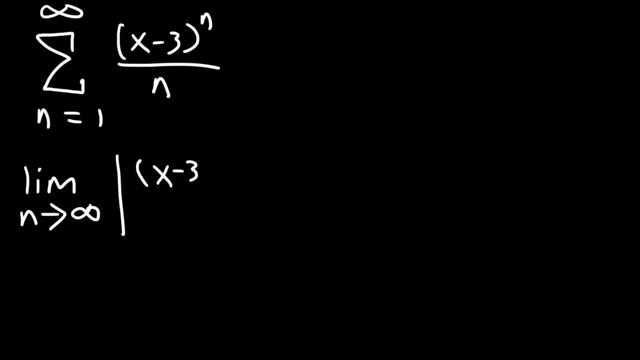 So u sub n plus 1, that's going to be x minus 3 raised to the n plus 1, divided by n plus 1.. And then we're going to divide that by u sub n, which is x minus 3 to the n over n. 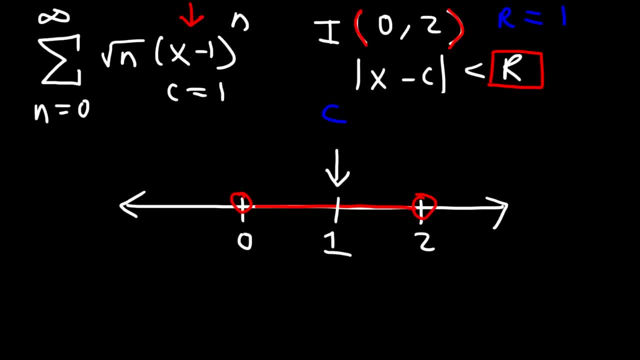 so this is the c-value, And the radius of convergence is basically the distance from the center to the end of the interval. So this distance is r, And so we can see why r is 1, because between 0 and 1,. 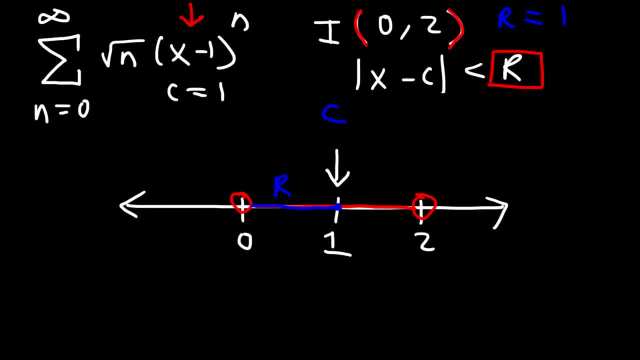 that distance is approximately 1.. So r is typically 1 half of the length of the interval. So if it goes from 0 to 2, then if you take the difference between 0 and 2, which is 2,, divide it by 2,. 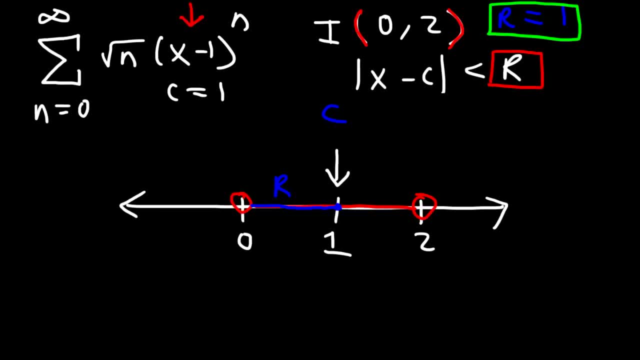 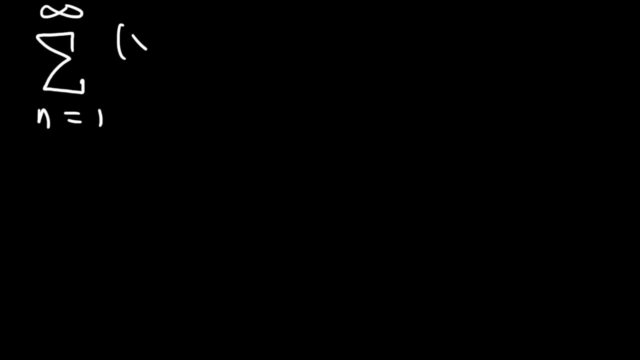 that's your radius of convergence, And so that's it for this problem. Hopefully this gives you a better understanding of it. Let's try this power series. Let's say it's x minus 3 to the n divided by n. So let's start with the ratio test. 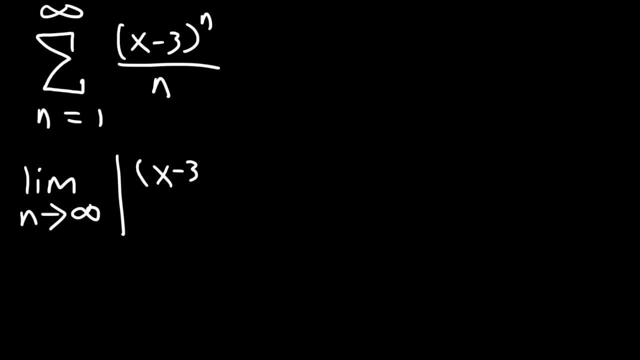 So u sub n plus 1, that's going to be x minus 3 raised to the n plus 1, divided by n plus 1.. And then we're going to divide that by u sub n, Which is x minus 3 to the n over n. 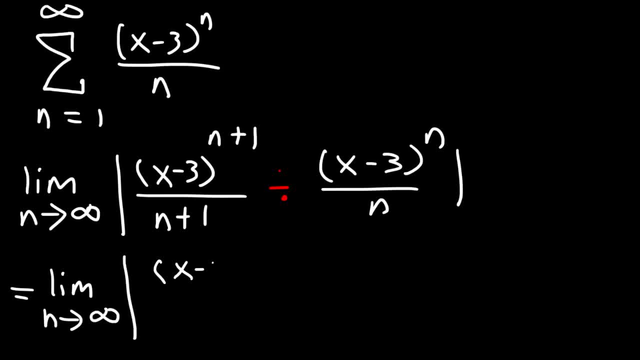 So then we can write x minus 3 to the n plus 1 as x minus 3 to the n times x minus 3 to the first power And n plus 1, that's not going to change, We're just going to leave that. 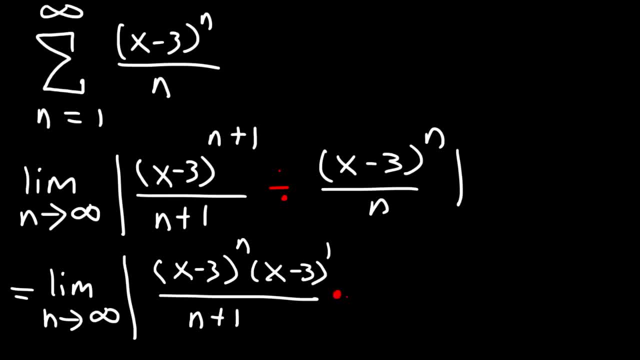 as n plus 1.. Now we're going to change division to multiplication and then flip the second fraction, So we have this. The only thing we can cancel right now is x minus 3 to the n power, And so we're left with the limit. 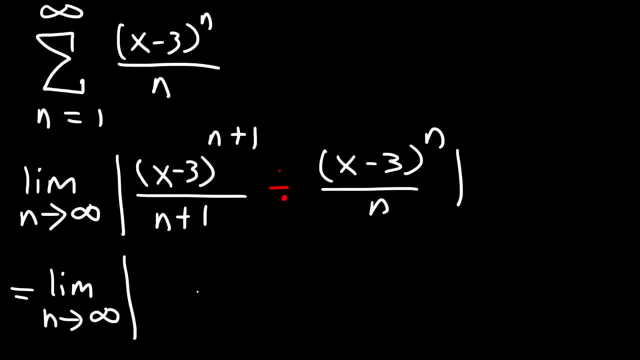 So then we can write x minus 3 to the n plus 1 as x minus 3 to the n times x minus 3 to the first power And n plus 1, that's not going to change, We're just going to leave that as n plus 1.. 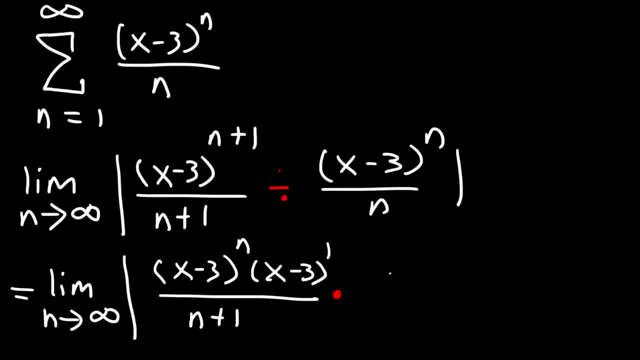 Now we're going to change division to multiplication and then flip the second fraction, So we have this. The only thing we can cancel right now is x minus 3 to the n power, And so we're left with the limit, as n goes to infinity, of the absolute value. 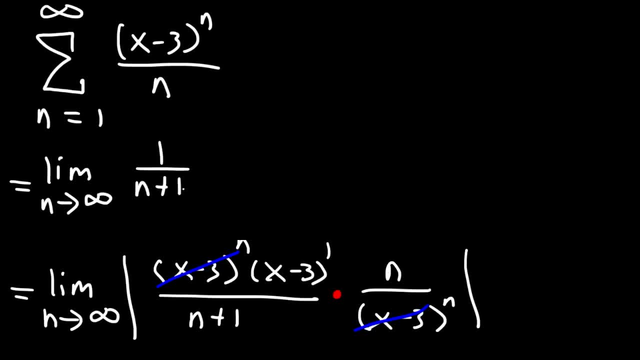 or we could just say: 1 over n plus 1 times the absolute value of x minus 3.. So as n goes to infinity. actually wait, I'm forgetting something. I can't forget this n, So let's put that on top. 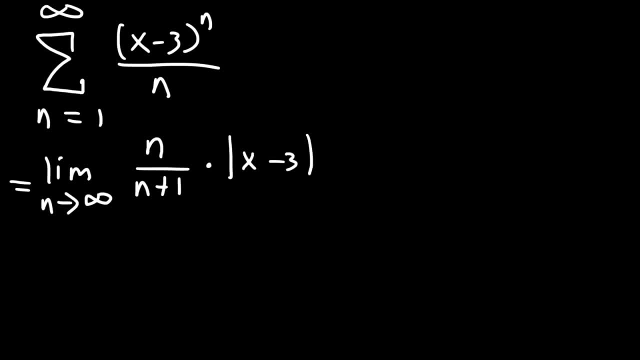 That would have been a very big mistake. So, as n goes to infinity, what happens to n over n plus 1?? The 1 is insignificant, so it becomes n over n, which becomes 1.. So this is 1 times the absolute value of x minus 3.. 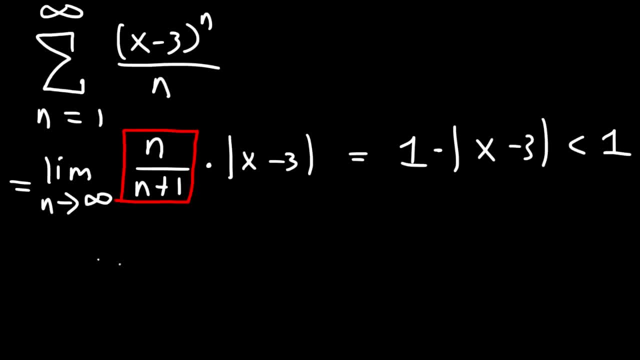 And so that's less than 1.. And so we can say that x minus 3 is between 1 and negative 1.. Now if we add 3 to both sides, then x is between 4 and 2.. And the midpoint of 2 and 4 is 3,. 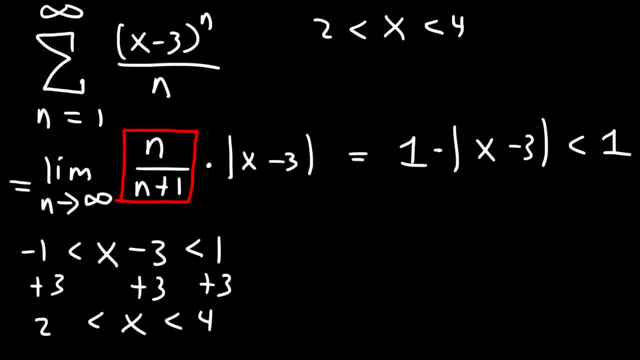 so we can see that it's centered at 3.. So c is 3.. Now, what is the radius of convergence? What is that? equal to Well, if you take the distance between the midpoint of the interval, which is 3,. 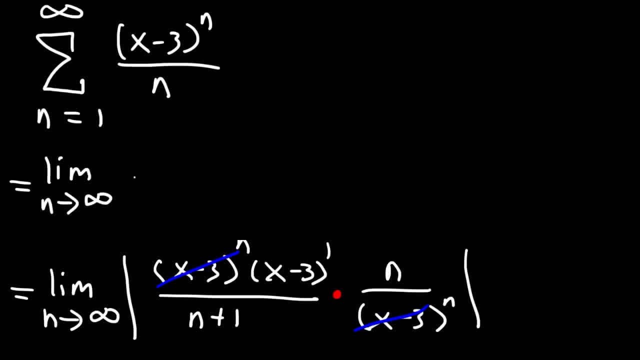 as n goes to infinity of the absolute value. or we could just say: 1 over n plus 1 times the absolute value of x minus 3.. So as n goes to infinity. actually, wait, I'm forgetting something. I can't forget this n. 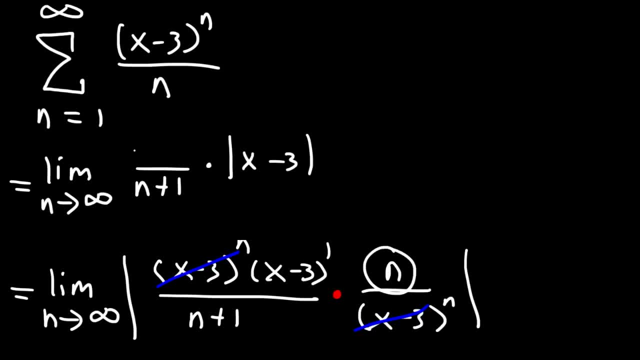 So let's put that on top. That would have been a very big mistake. So, as n goes to infinity, what happens? It happens to n over n plus 1.. The 1 is insignificant, so it becomes n over n, which becomes 1.. 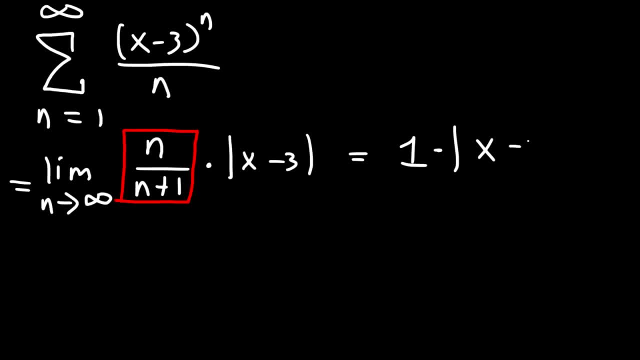 So this is 1 times the absolute value of x minus 3.. And so that's less than 1.. And so we could say that x minus 3 is between 1 and negative 1.. Now if we add 3 to both sides, 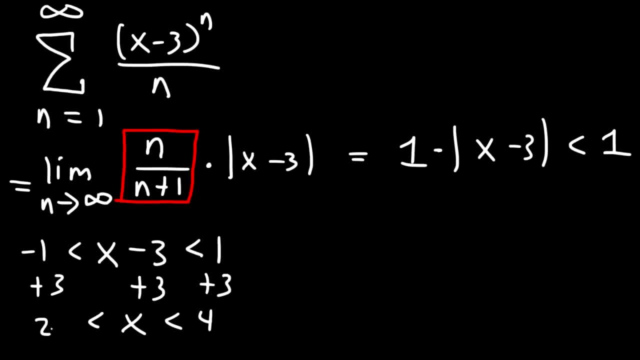 x is between 4 and 2.. And the midpoint of 2 and 4 is 3.. So we could see that it's centered at 3.. So c is 3.. Now, what is the radius of convergence? What is that equal to? 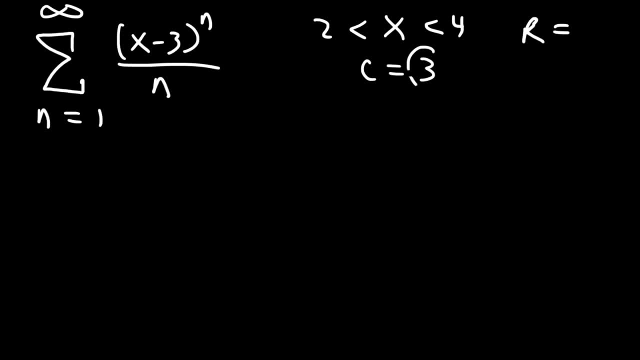 Well, if you take the distance between the midpoint of the interval, which is 3,, and one of the endpoints, the difference between 3 and 2 is 1.. So the radius of convergence is 1.. Or once we had it in this form. 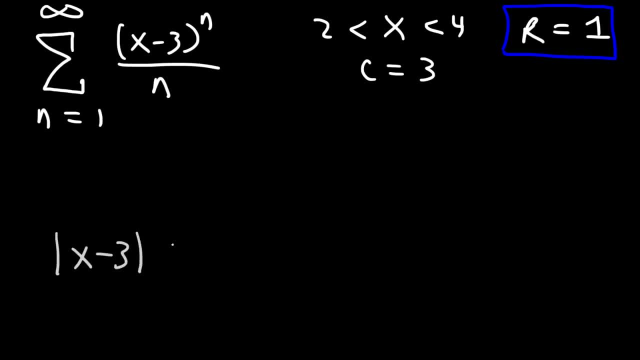 the absolute value of x minus 3 is less than 1.. We have it in the form of x minus c. the absolute value of that is less than r. So you can see, at this point r is 1.. So now we need to check. 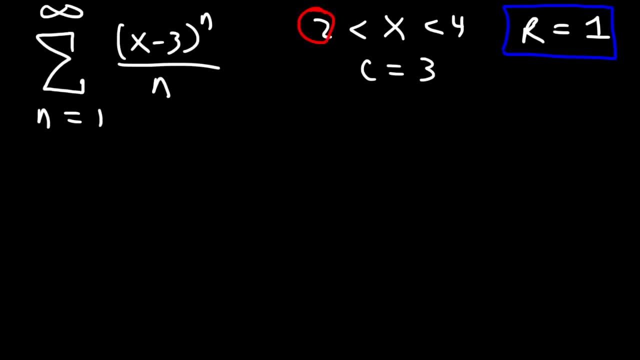 the endpoints. So let's start with 2.. So when x is 2, will the power series converge or will it diverge? So 2 minus 3, that's negative 1.. So we're going to have negative 1 to the n power. 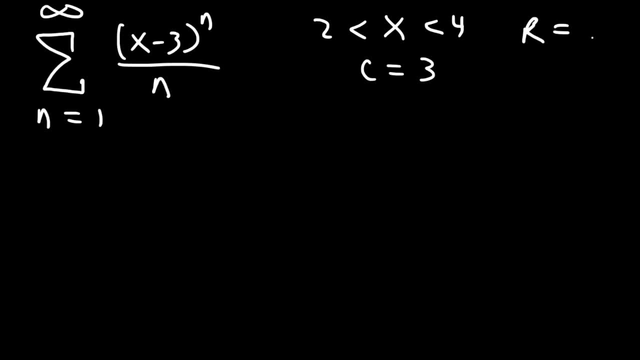 and one of the endpoints. the difference between 3 and 2 is 1.. So the radius of convergence is 1.. Or, once we had it in this form, the absolute value of x minus 3 is less than 1.. 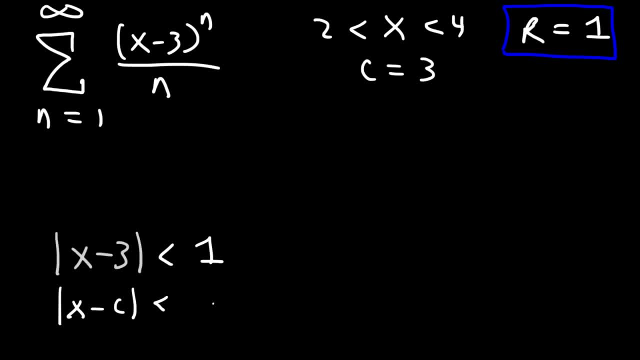 We have it in the form of x minus c. The absolute value of that is less than r. So you can see, at this point r is 1.. So now we need to check the endpoints, So let's start with 2.. 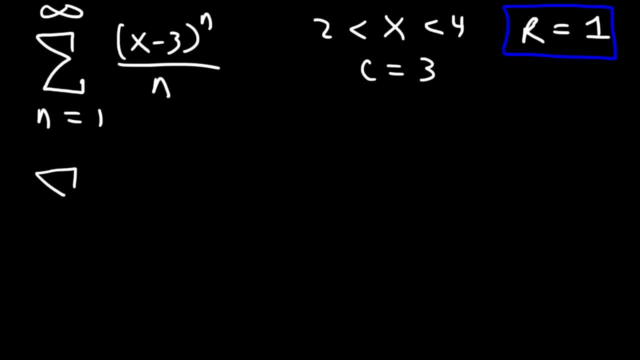 So when x is 2, will the power series converge or will it diverge? So 2 minus 3, that's negative 1.. So we're going to have negative 1 to the n power over n. So notice that this is the alternating harmonic series. 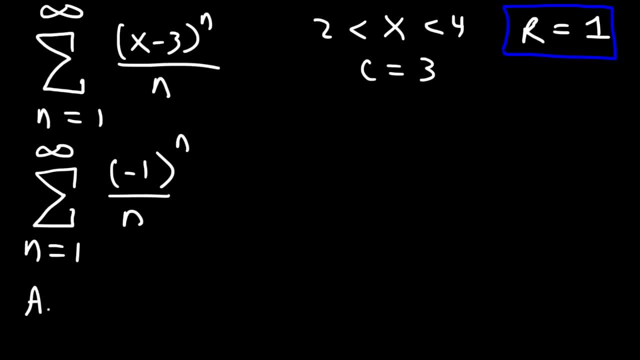 So we need to employ the alternating series test AST. So let's start with the divergence test. So we're going to take the limit, as n goes to infinity, of a sub n. a sub n is everything except the negative 1 to the n power. 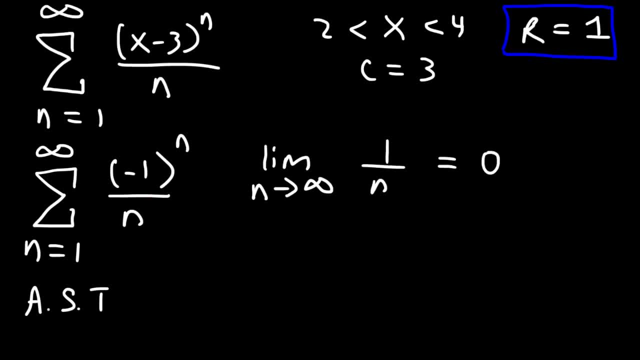 So we're just focused on 1 over n And that goes to 0. So it passes the divergence test. This tells us that it may converge or it may diverge. Now for the alternating series test, the second thing we need to show. 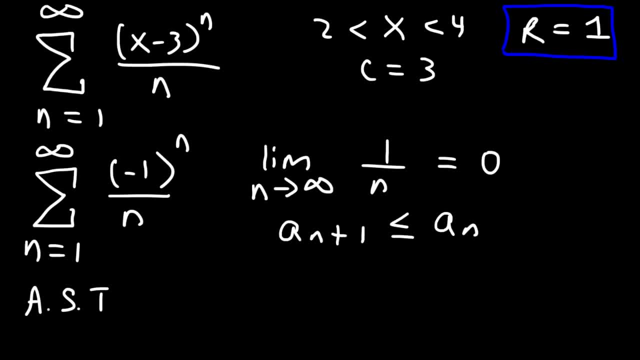 is that a sub n plus 1 is less than or equal to a sub n. So in this case, for the alternating series test, a sub n is 1 over n. So just keep that in mind. It's you take out the negative 1 to the n power. 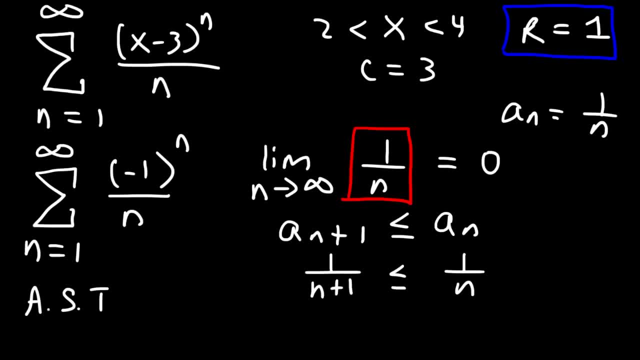 Now a sub n plus 1, that's 1 over n plus 1.. 1 over n is always greater than 1 over n plus 1.. So the two conditions of the alternating series test has been met, So we can say that the series converges. 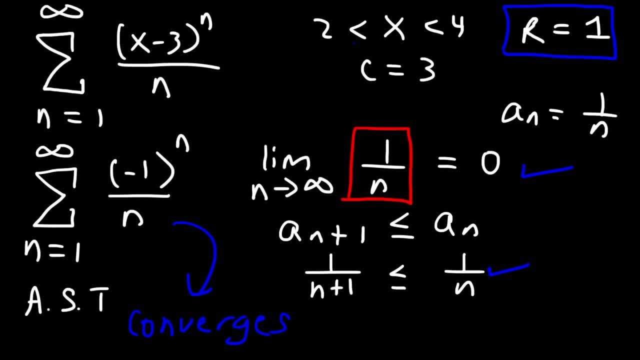 by the alternating series test. So we can say that x is equal to or greater than 2.. So 2 is equal to or greater than 2.. So 2 is equal to or greater than 2.. That says that x is included. 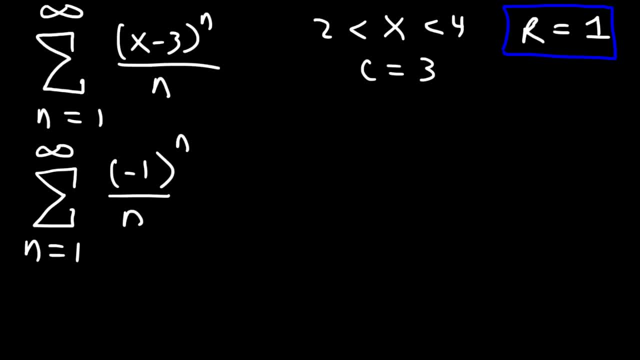 over n. So notice that this is the alternating harmonic series. So we need to employ the alternating series test AST. So let's start with the divergence test. So we're going to take the limit, as n goes to infinity of a sub n. 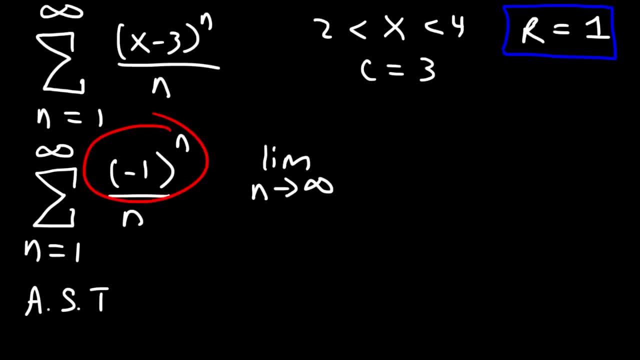 a sub n is everything except the negative 1 to the n power. So we'll just focus on 1 over n And that goes to 0.. So it passes the divergence test. This tells us that it may converge or it may diverge. 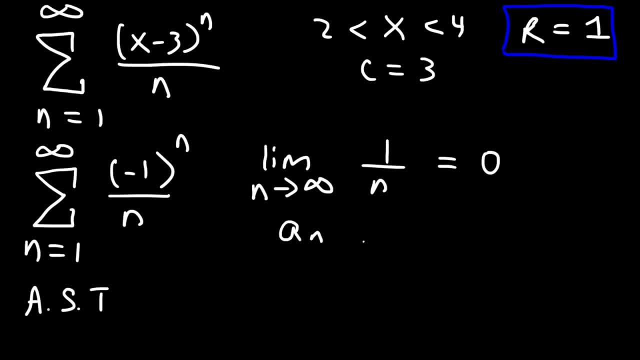 Now for the alternating series test. the second thing we need to show is that a sub n plus 1 is less than or equal to a sub n. So in this case, for the alternating series test, a sub n is 1 over n. 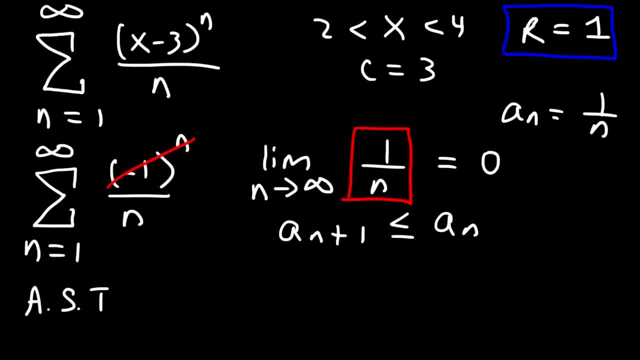 So just keep that in mind. You take out the negative 1 to the n power, Now a sub n plus 1, that's 1 over n plus 1.. 1 over n is always greater than 1 over n plus 1.. 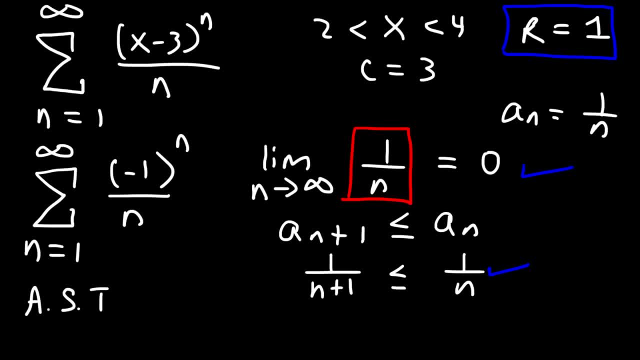 So the two conditions of the alternating series test has been met. So we can say that the series converges by the alternating series test. So we can say that x is equal to or greater than 2.. So 2 is included. Now we need to see if 4. 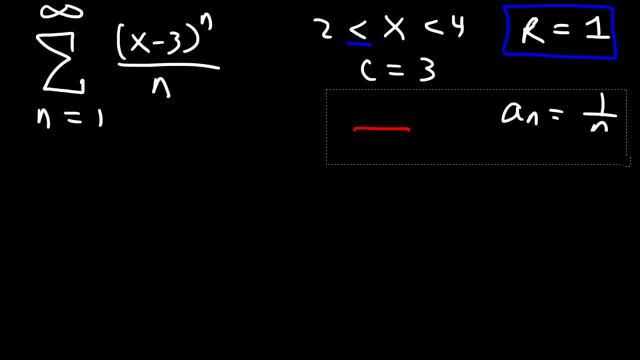 is going to be included in the interval of convergence. Now let's substitute x with 4.. So we're going to get the series 4 minus 3 to the n, which is 1 to the n, And 1 to the n is just 1.. 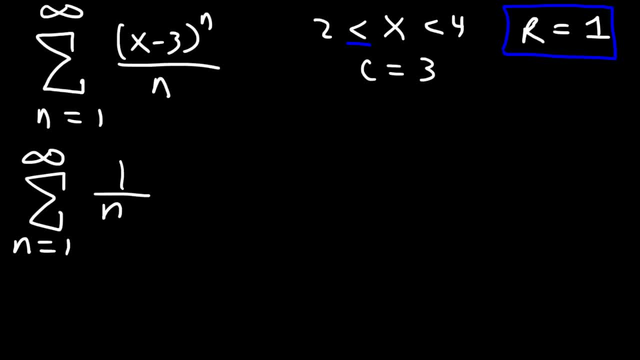 So we're going to have 1 over n. So this is the divergent harmonic series And based on the p-series test, you can see that p is equal to 1.. So if p is equal to 1, it's going to diverge. 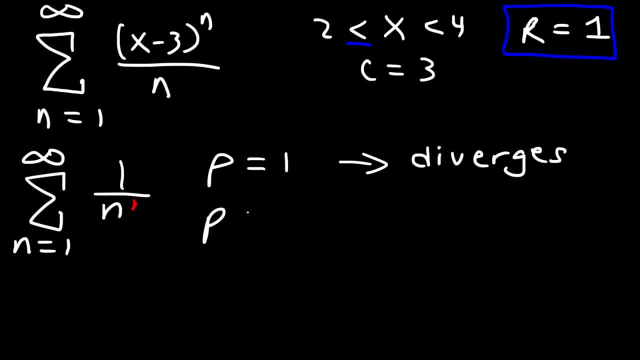 In order for the p-series to converge, p has to be greater than 1.. Then it will converge. If it's less than or equal to 1, it diverges. So, since p is exactly 1, this particular series diverges. 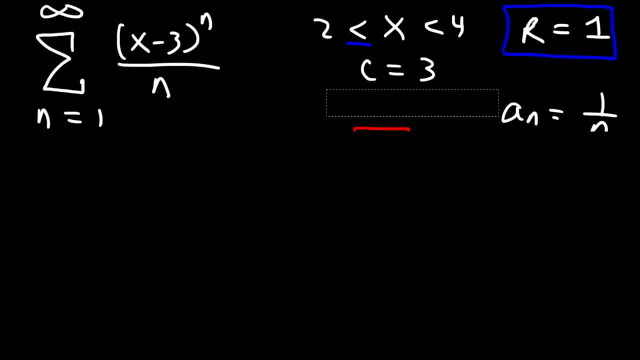 Now we need to see if 4 is going to be included in the interval of convergence. Now let's substitute x with 4.. So we're going to get the series 4 minus 3 to the n, which is 1 to the n. 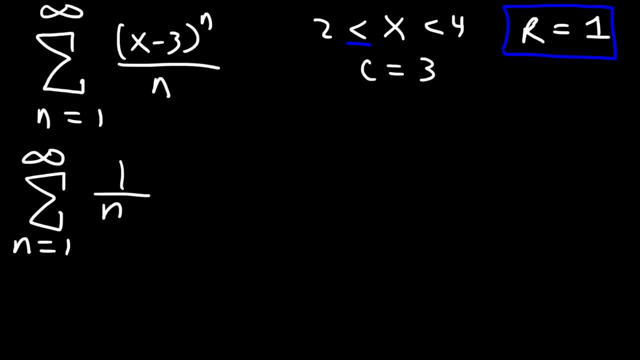 And 1 to the n is just 1.. So we're going to have 1 over n. So this is the Divergent Harmonic Series And based on a p-series test, you can see that p is equal to 1.. 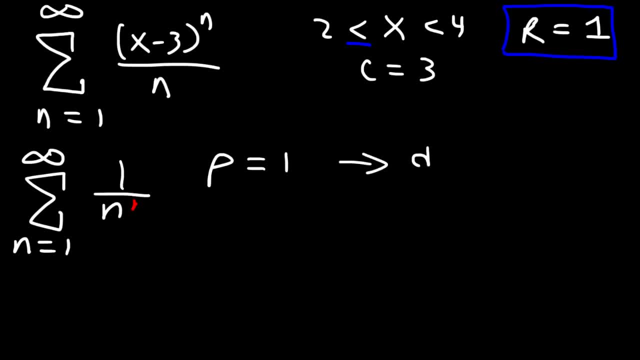 So if p is equal to 1, it's going to diverge. In order for the p-series to converge, p has to be greater than 1.. Then it will converge. If it's less than or equal to 1, it diverges. 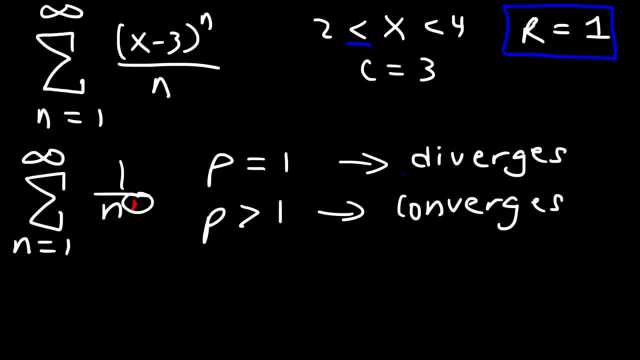 So since p is exactly 1, this particular series diverges. So 4 is not included. So we can write the interval of convergence like this: So it's going to be a bracket at 2 and a parenthesis at 4.. So, plotting it on a number line, we have the center at c and the endpoints are 2 and 4.. 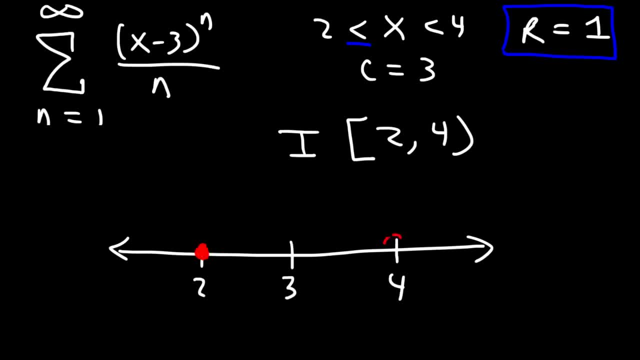 So we're going to have a closed circle at 2 and an open circle at 4.. And here we have a closed circle at 2 and an open circle at 4.. And here we have a closed circle at 2 and an open circle at 4.. 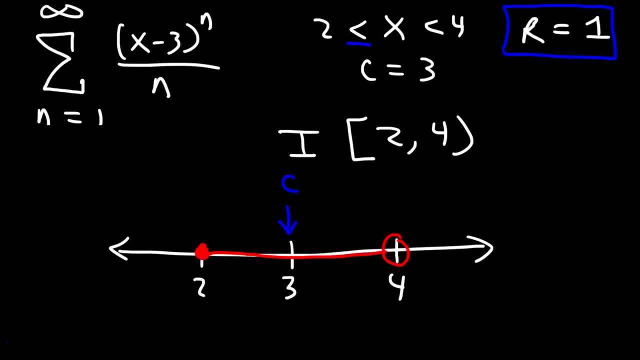 And here is our c-value. The power series is centered at 3.. And so this is the radius of convergence, which is 1.. And so that's it for this problem. So anywhere between 2 and 4,, if you plug it in, the series will converge. 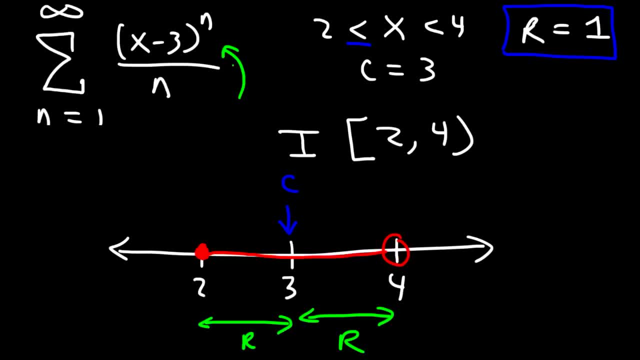 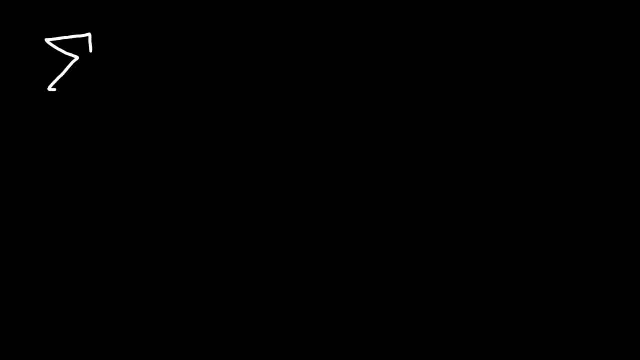 It doesn't converge at 4, but it converges at 2 and anywhere between 2 and up to 4, but not including 4.. So let's work on one more. Let's work on one more example problem: Consider the power series from 1 to infinity, of negative: 1 raised to the n, plus 1 times x minus 4 raised to the n, divided by n times 9 raised to the n. 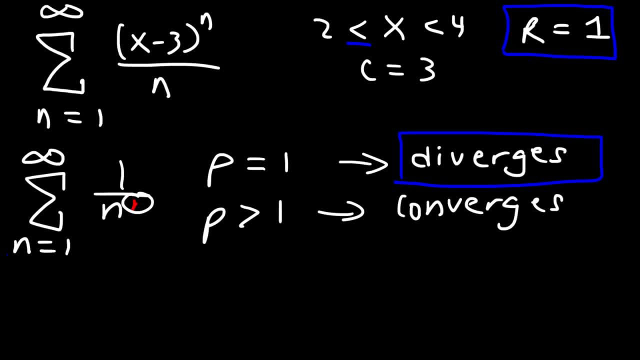 So 4 is not included. So we can write the interval of convergence like this: So it's going to be a bracket at 2 and a parenthesis at 4.. So, plotting it on a number line, we have this series center at c. 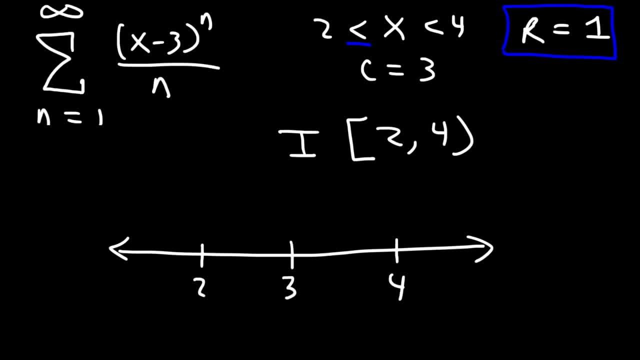 and the endpoints are 2 and 4.. So we're going to have a closed circle at 2 and an open circle at 4.. And here is our c value. The power series is centered at 3.. And so this is the radius. 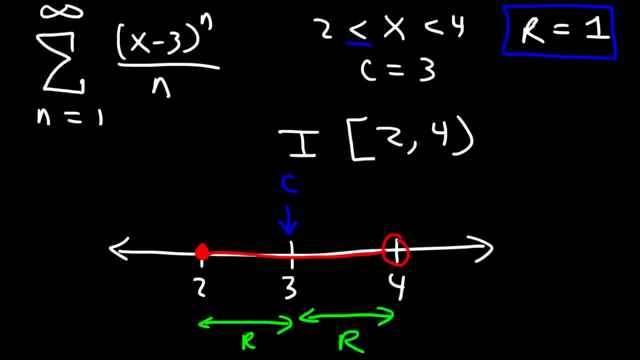 of convergence, which is 1.. And so that's it for this problem. So anywhere between 2 and 4,, if you plug it in, the series will converge. It doesn't converge at 4, but it converges at 2. 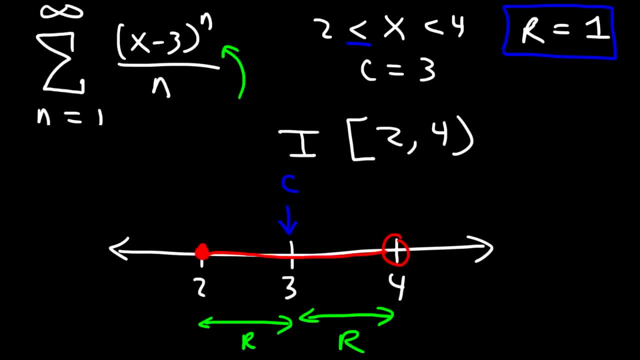 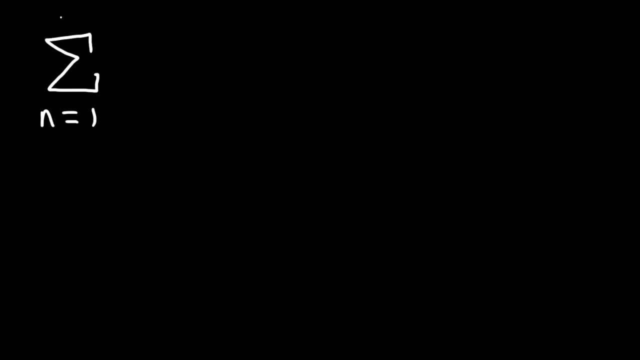 and anywhere between 2 and up to 4, but not including 4.. So let's work on one more example problem. Consider the power series from 1 to infinity of negative. 1 raised to the n plus 1 times x minus 4. 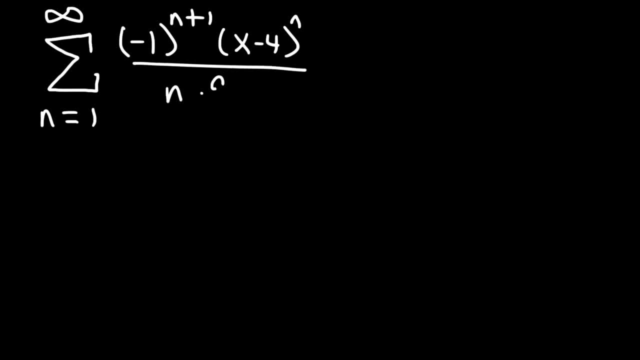 raised to the n, divided by n times 9 raised to the n. So go ahead and determine the radius and the interval of convergence for this power series. So let's start with the ratio test: u sub n plus 1.. That's going to be. 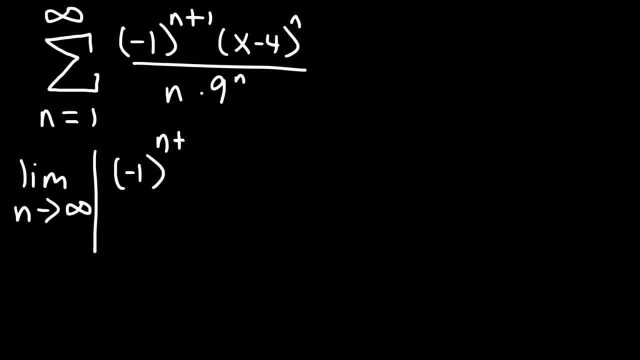 negative 1 to the n plus 1 plus 1.. So everywhere you see an n, replace it with n plus 1.. And then it's going to be divided by u sub n, the original expression: Negative 1 to the n plus 1.. 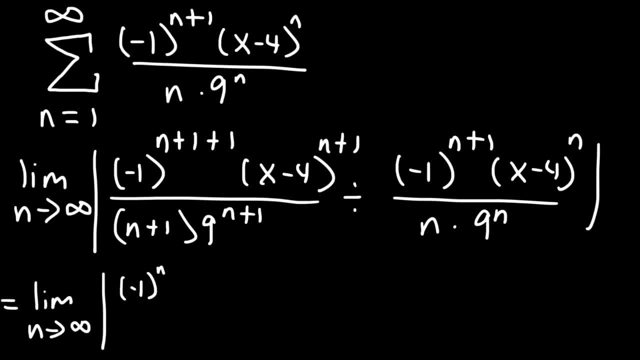 I'm going to separate it like this: Negative 1 to the n plus 1.. Well, this is n plus 2, really, I'm going to separate it as negative 1 to the n plus 1 times negative 1 to the first power. 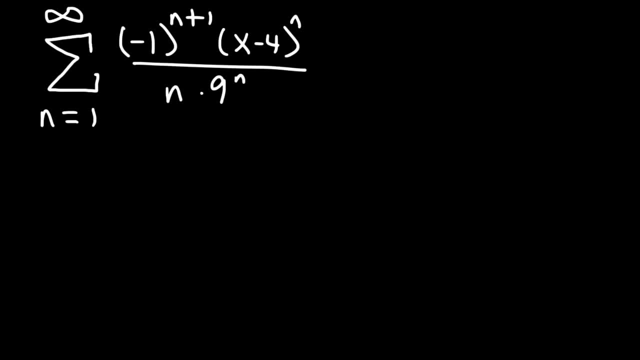 So go ahead and determine the radius and the interval of convergence for this power series. So let's start with the ratio test: u sub n plus 1.. That's going to be negative 1.. That's going to be negative 1 to the n plus 1 plus 1.. 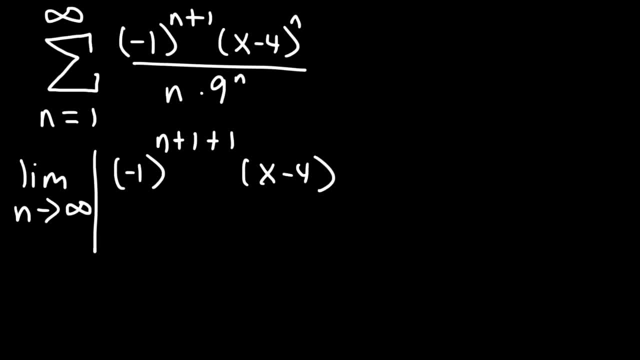 So everywhere you see an n, replace it with n plus 1.. And then it's going to be divided by u sub n, the original expression, Negative 1 to the n plus 1.. I'm going to separate it like this. 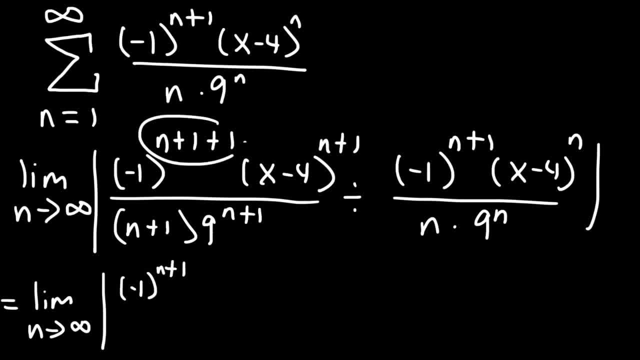 Negative 1 to the n plus 1.. Well, this is n plus 2, really, But I'm going to separate it as negative 1 to the n plus 1 times negative 1 to the first power, And then x minus 4 to the n plus 1.. 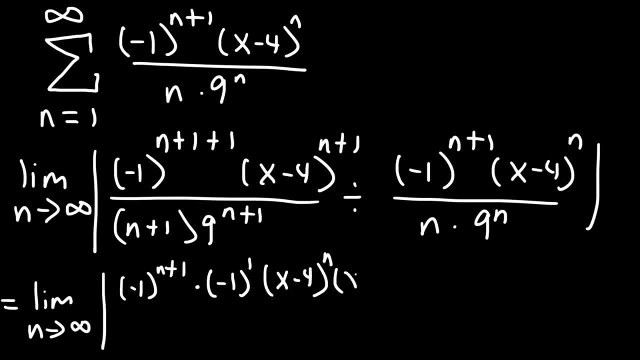 I'm going to write that as x minus 4 to the n times x minus 4 to the first power, n plus 1, I can't really change that. I'm just going to leave it the way it is: 9 to the n plus 1.. 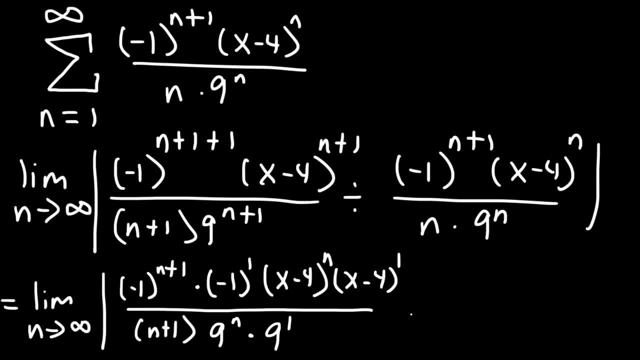 I can write that as 9 to the n times 9 to the 1. Then change division to multiplication And then flip the second fraction. Okay, so now let's simplify what we have. These two we can cancel. We can cancel x minus 4 to the n. 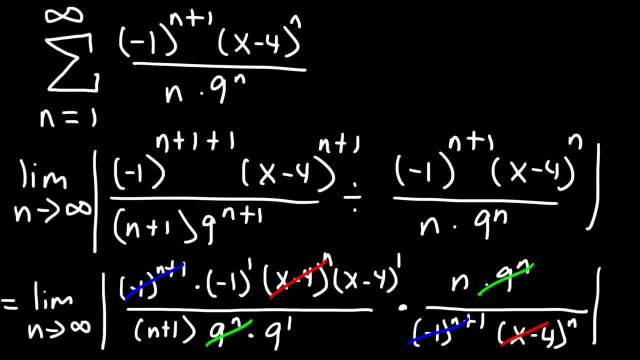 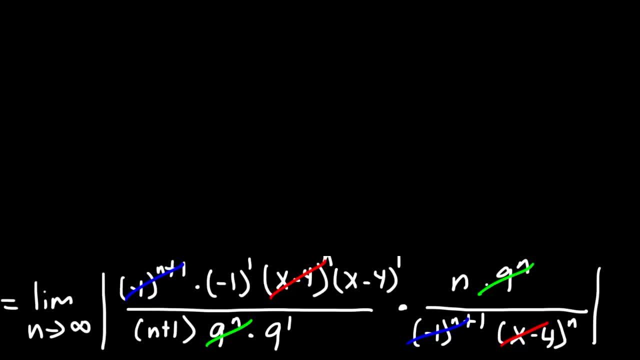 And also 9 to the n power. Now let's write these two together. So this is the limit, as n goes to infinity, n over n plus 1.. And then we have absolute value: Negative: 1 times x, x minus 4.. 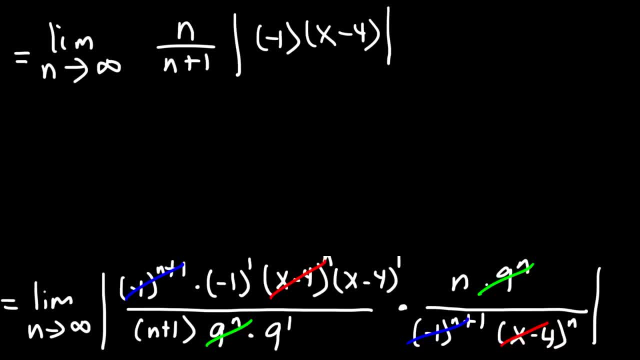 Now, as n goes to infinity, Oh, let's not forget about the 9 on the bottom. So let's put this over 9.. As n goes to infinity, what happens to n over n plus 1? This becomes 1.. 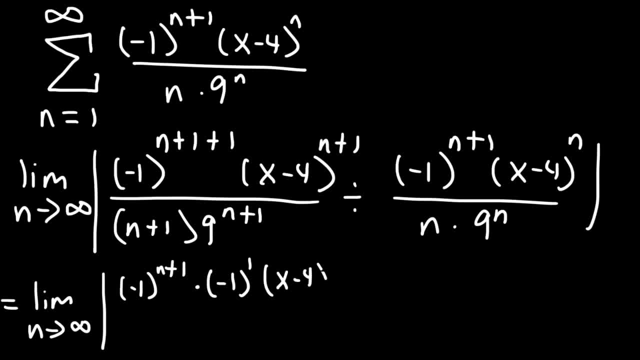 And then x minus 4 to the n plus 1.. I'm going to write that as x minus 4 to the n times x minus 4 to the first power, n plus 1.. I can't really change that, I'm just going to leave it. 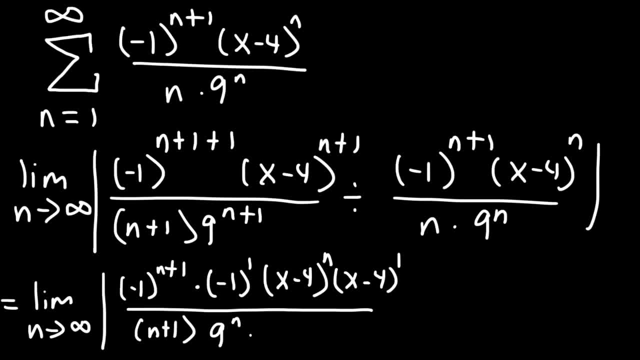 the way it is: 9 to the n plus 1.. I could write that as 9 to the n times 9 to the 1. Then change division to multiplication And then flip the second fraction. Okay, so now let's simplify. 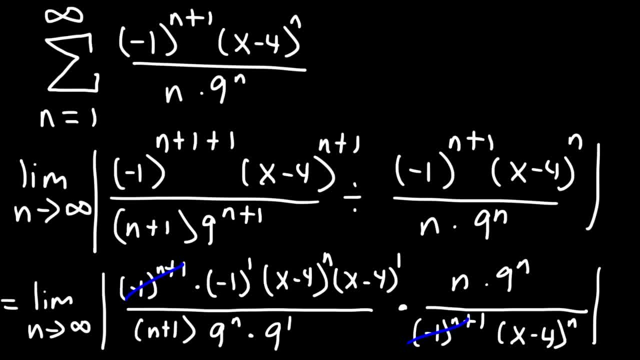 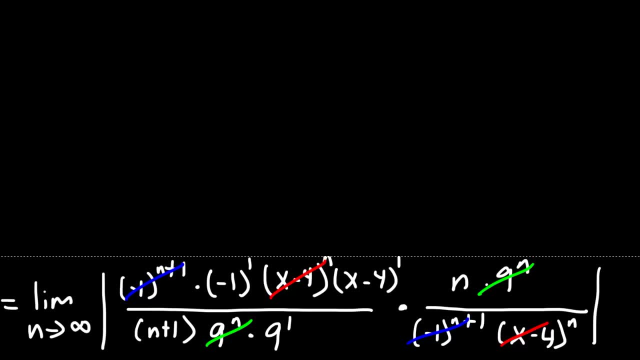 what we have. These two we can cancel. We can cancel x minus 4 to the n and also 9 to the n power. Now let's write these two together. So this is the limit as n goes to infinity, n over n plus 1.. 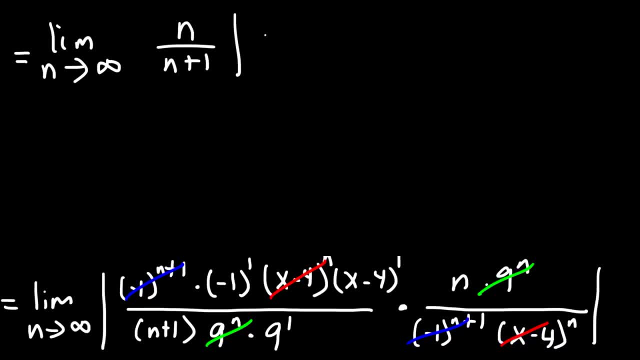 And then we have absolute value negative 1 times x minus 4.. Now, as n goes to infinity, let's not forget about the 9 on the bottom, So let's put this over 9.. As n goes to infinity, what happens to? 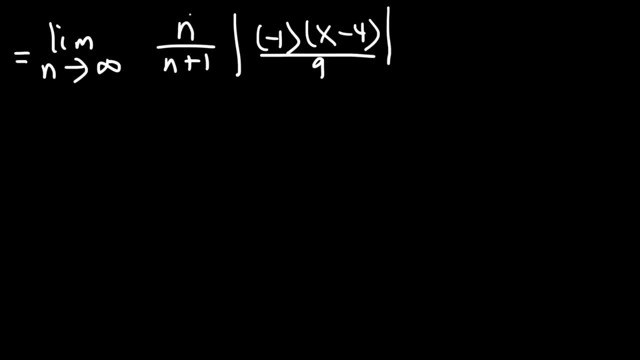 n over n plus 1? This becomes 1.. 1000 over 1001, that's about 1.. And then the absolute value of negative 1 over 9, we can take that out of the absolute value expression and write it as: 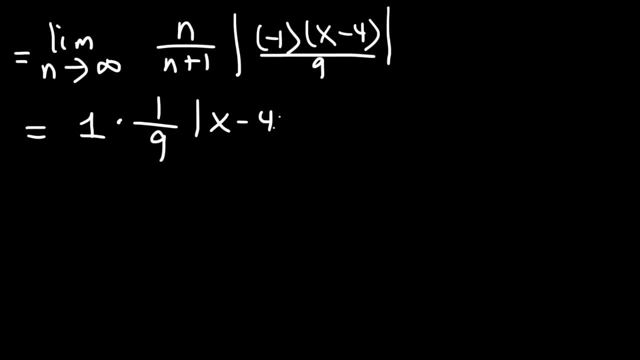 1 over 9.. So what we have now is 1 over 9 times the absolute value of x minus 4.. And this is going to converge when the ratio test is less than 1.. So now what we need to do is multiply both sides. 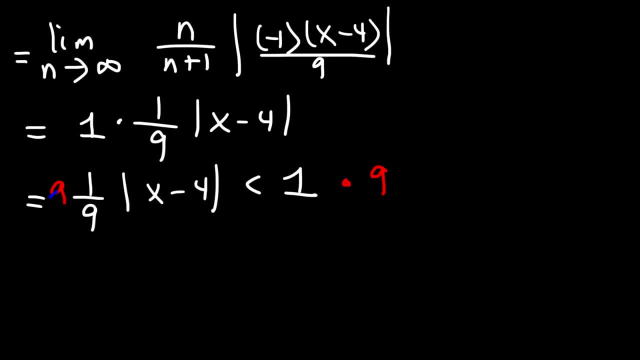 by 9.. And so these will cancel. And so now we have: x minus 4 is less than 9.. So notice that this is the form: x minus c is less than r, So therefore we can see that r is 9.. 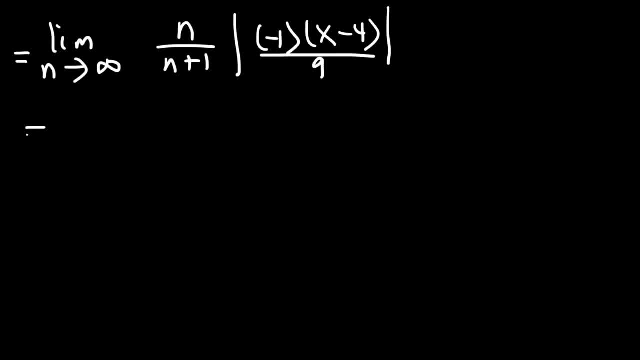 1,000 over 1,001, that's about 1.. And then the absolute value, The absolute value of negative, 1 over 9.. We can take that out of the absolute value expression and write it as 1 over 9.. 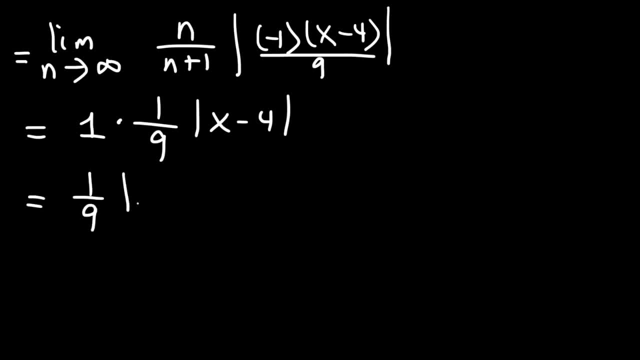 So what we have now is 1 over 9 times the absolute value of x minus 4.. And this is going to converge when the ratio test is less than 1.. So now what we need to do is multiply both sides by 9.. 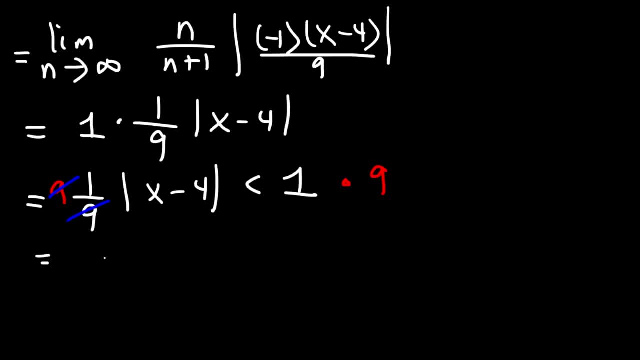 And so these will cancel. And so now we have x. x minus 4 is less than 9.. So notice that this is the form: x minus c is less than r, So therefore we can see that r is 9.. That's the radius of convergence. 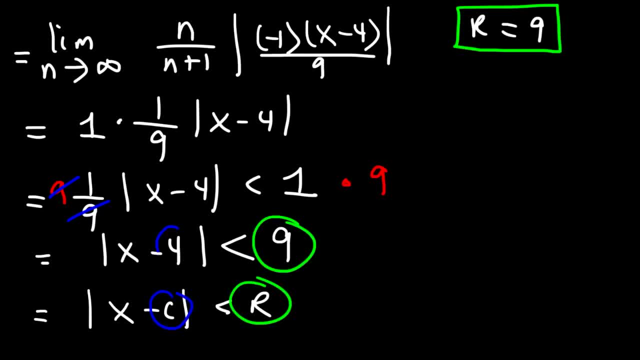 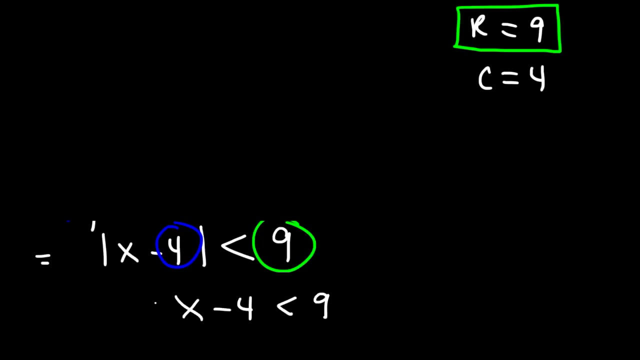 We can also see that c, the series, is centered at 4.. So c is 4.. So now let's determine the interval of convergence. So we can say that x minus 4 is less than 9, but greater than negative 9.. 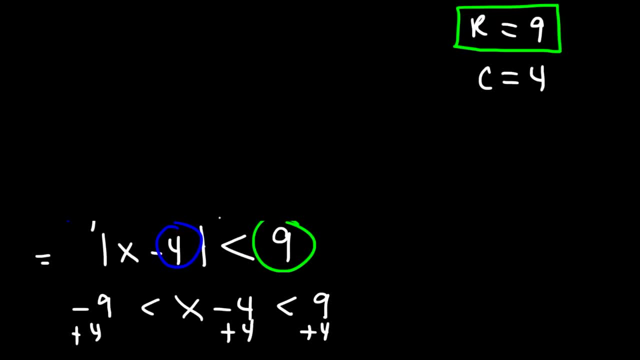 Now let's add 4 to both sides: 9 plus 4 is 13.. Negative: 9 plus 4 is negative: 5.. So this is what we now have. Now let's rewrite. Let's rewrite the original series, Which is negative: 1 to the n plus 1 times x, minus 4 to the n, divided by n times 9 to the n. 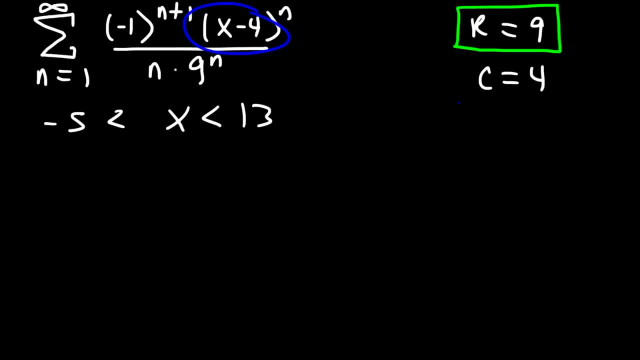 So just by looking at it you can see that the power series is centered at c equals 4 because of the x minus 4 in it. Now let's check the endpoints. So if we plug in the power series, we can see that the power series is centered at c equals 4.. 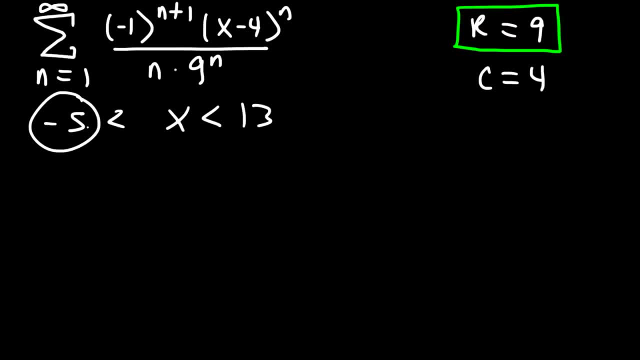 So if we plug in negative 5, will it converge or diverge? So let's replace x with negative 5.. So we're going to get the series Negative 5 minus 4, that's negative 9 to the n. 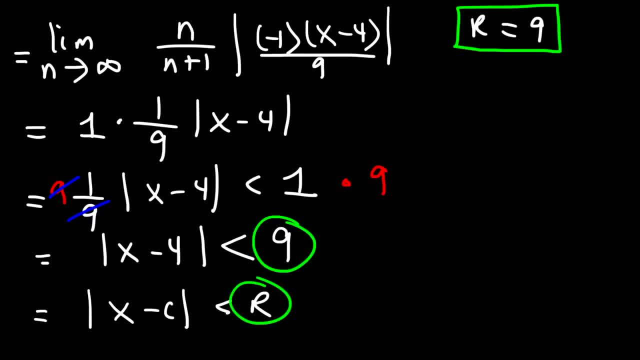 That's the radius of convergence. We can also see that c, the series is centered at 4.. So c is 4.. So now let's determine the interval of convergence. So we can say that x minus 4 is less than 9. 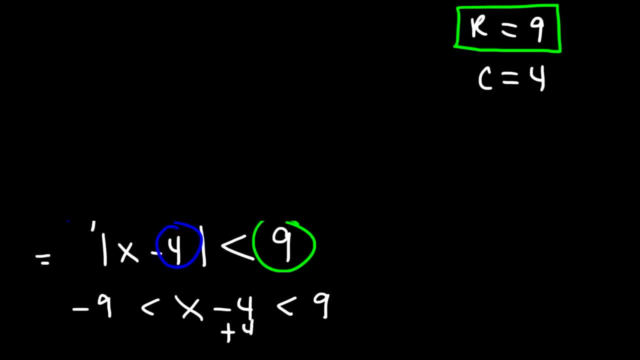 but greater than negative 9.. Now let's add 4 to both sides. 9 plus 4 is 13.. Negative 9 plus 4 is negative 5.. So this is what we now have. Now let's rewrite the original series. 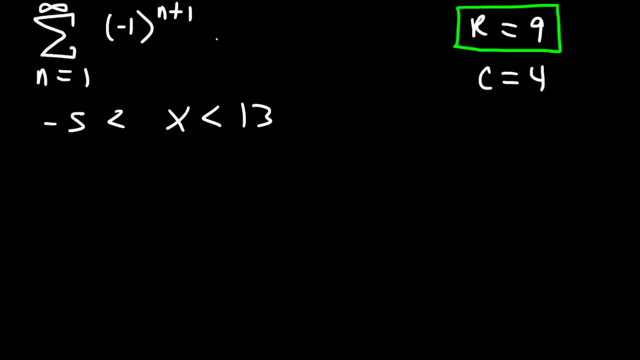 Which is negative, 1 to the n plus 1.. Times x minus 4 to the n, Divided by n times 9 to the n. So just by looking at it you can see that the power series is centered at c equals 4.. 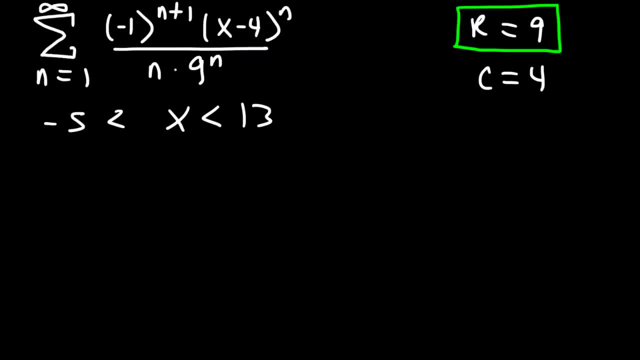 Because of the x minus 4 in it. Now let's check the endpoints. So if we plug in negative 5, will it converge or diverge? So let's replace x with negative 5.. So we're going to get the series negative 5 minus 4. 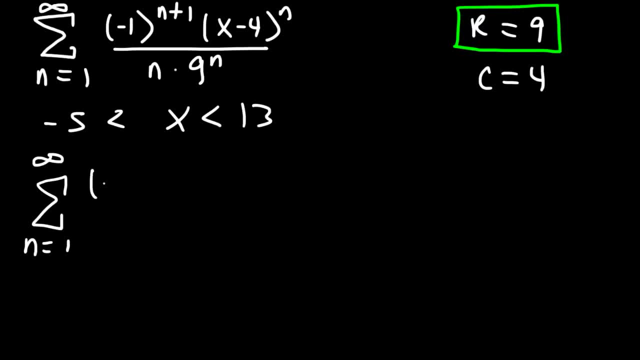 that's negative 9 to the n. So we're going to have negative 1 to the n plus 1 and then negative 9 raised to the n over n times 9 to the n. Now negative 9 to the n divided by 9 to the n. 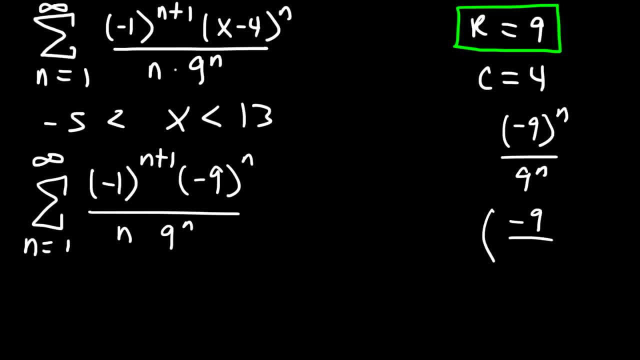 we can write that as negative 9 over 9 to the n, which becomes negative 1 to the n. And so if we multiply negative 1 to the n with negative 1 to the n plus 1, then that becomes negative 1 to the 2n plus 1.. 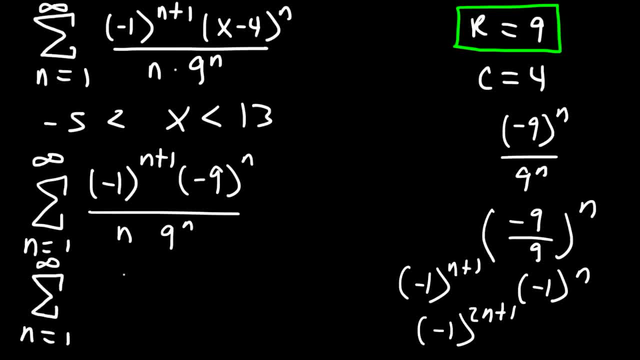 So this gives us the series negative 1 to the 2n plus 1 divided by n. So what can we do with negative 1 to the 2n plus 1?? So when n is 1, 2 times 1 plus 1, 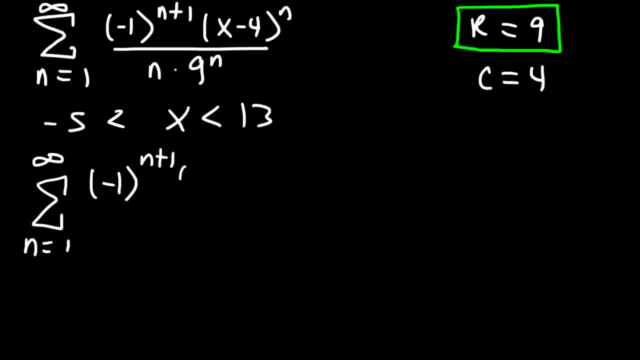 So we're going to have negative 1 to the n plus 1.. And then negative 9 raised to the n over n times 9 to the n, Now negative 9.. To the n divided by 9 to the n, We can write that as negative 9 over 9 to the n, which becomes negative 1 to the n. 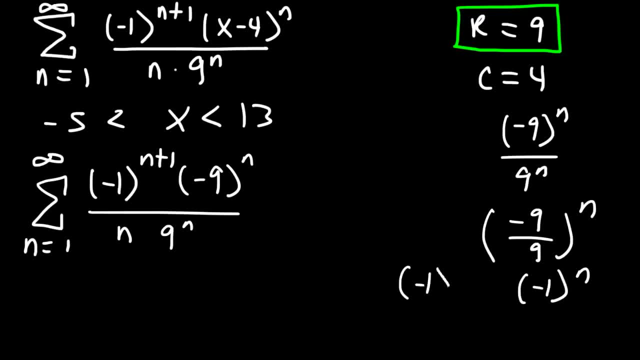 And so if we multiply negative 1 to the n with negative 1 to the n plus 1, then that becomes negative 1 to the 2n plus 1.. So this gives us the series Negative 1 to the 2n plus 1 divided by n. 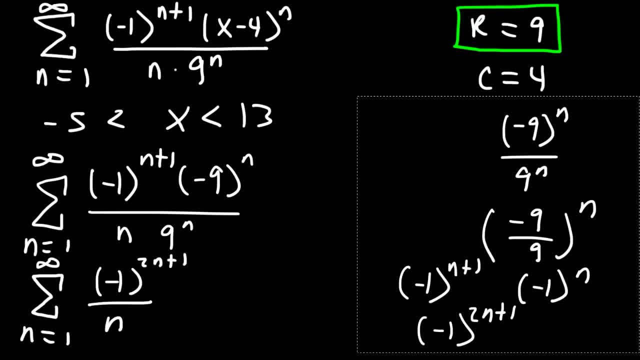 So what can we do with negative 1 to the 2n plus 1?? So when n is 1, 2 times 1 plus 1, that's going to be 3.. And negative 1 to the third power, that's negative 1.. 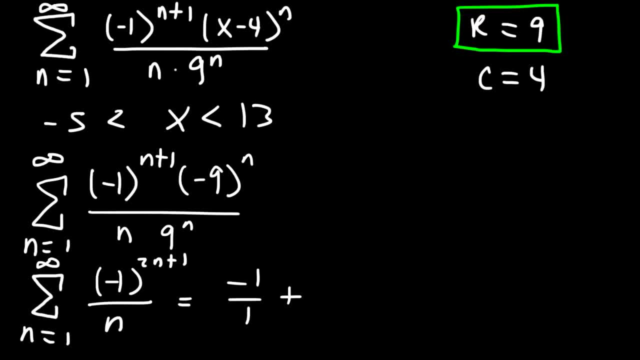 So we're going to have negative 1 over 1.. Now the next term: when n is 2, 2 times 2 plus 1 is 5.. Negative 1 to the fifth power is still negative 1.. And then when n is 3, 2 times 3 plus 1 is 7.. 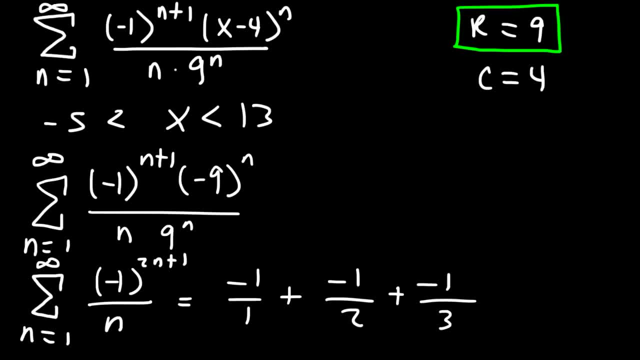 Negative 1 to the 7 is still negative 1.. So, as you can see, we don't have alternating signs, So we can reduce the series to this. We could say that it's simply negative 1 to the n And we can move the negative to the front. 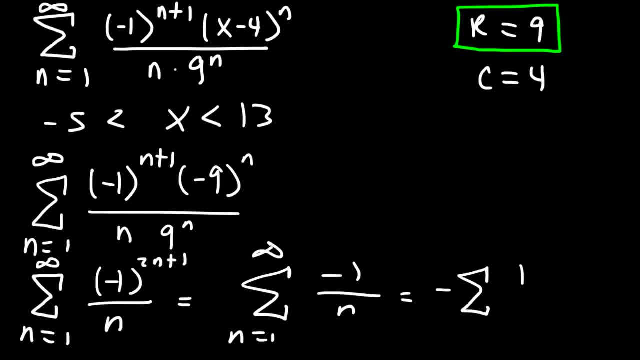 So this becomes negative. And then we have the divergent Harmonic series. So according to the p-series, p is 1.. And because p is 1, we can say that the series is divergent. So negative. 5 is not included. 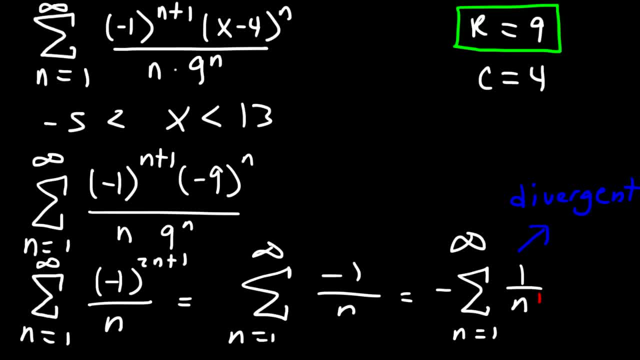 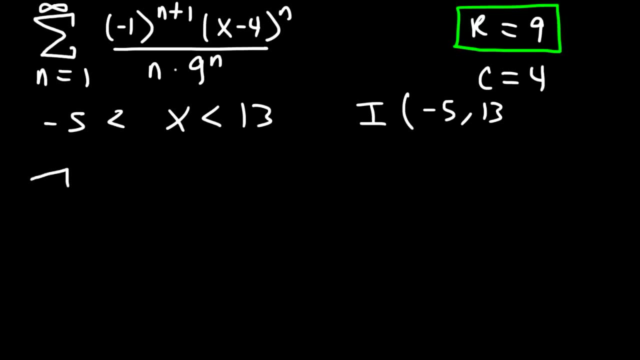 So we're going to have a parenthesis at negative 5.. So the interval of convergence is negative, 5 to 13.. Now let's check the endpoint for 13.. So when x is 13,, what's going to happen? So this is going to be 13 minus 4,, which is 9.. 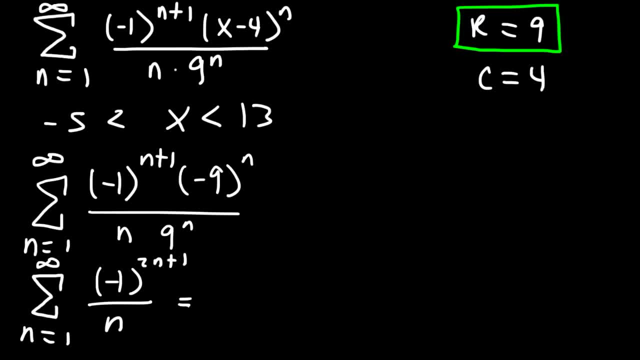 that's going to be 3.. And negative 1 to the third power, that's negative 1.. So we're going to have negative 1 over 1.. Now the next term: when n is 2, 2 times 2 plus 1 is 5.. 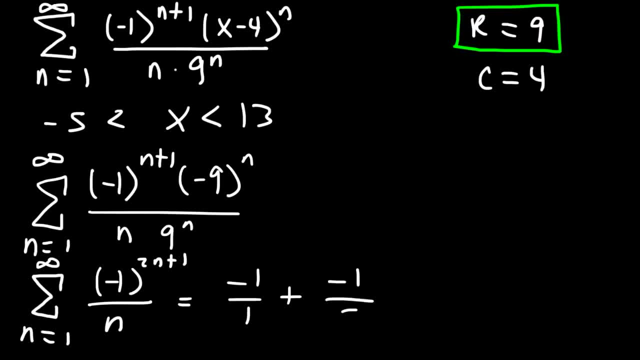 Negative: 1 to the fifth power is still negative 1.. And then when n is 3, 2 times 3 plus 1 is 7 negative. 1 to the 7 is still negative 1.. So, as you can see, we don't have alternating signs. 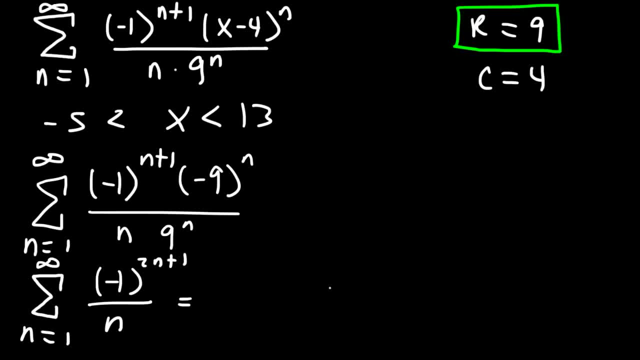 So we can reduce the series to this. We could say that it's simply negative 1 to the n And we can move the negative to the front. So this becomes negative. and then we have the divergent harmonic series. So according to the p-series, 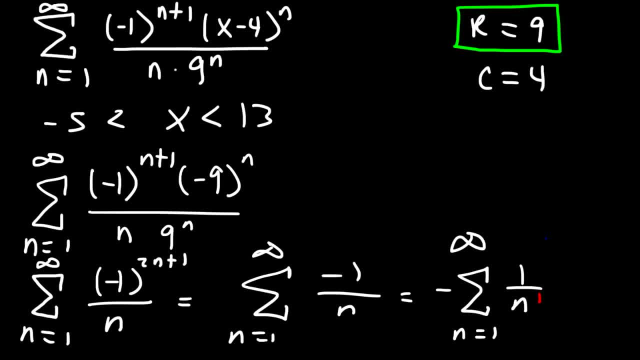 p is 1.. And because p is 1, we could say that the series is divergent. So negative 5 is not included. So we're going to have a parenthesis at negative 5.. So the interval of convergence is negative 5 to 13.. 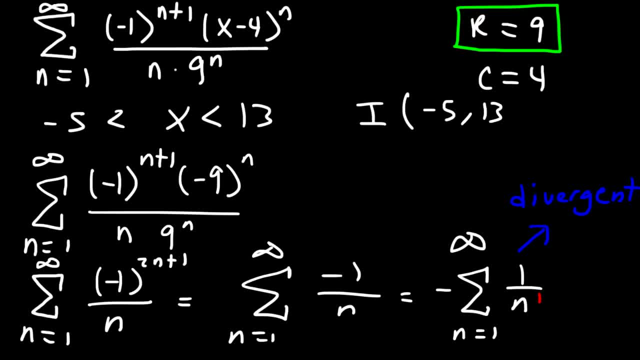 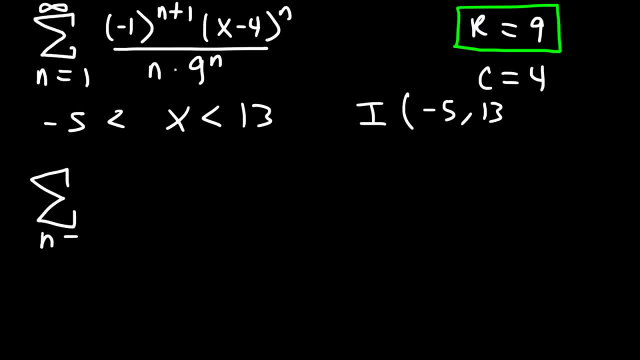 Now let's check the endpoint for 13.. So when x is 13, what's going to happen? So this is going to be 13 minus 4, which is 9.. So we're going to have negative 1 to the n plus 1. 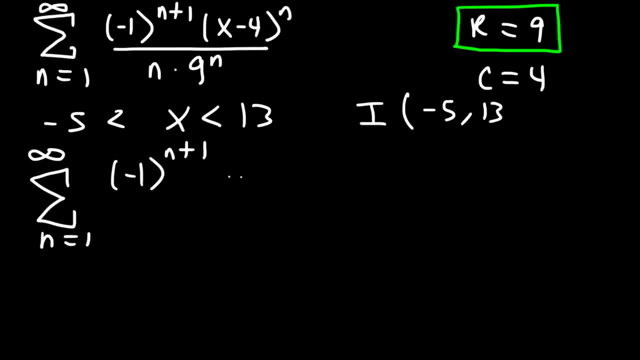 So we're going to have negative 1 to the n plus 1 times 9 to the n, over n times 9 to the n. So these will simply cancel. And now we have the alternating harmonic series, So we need to perform the alternating series test. 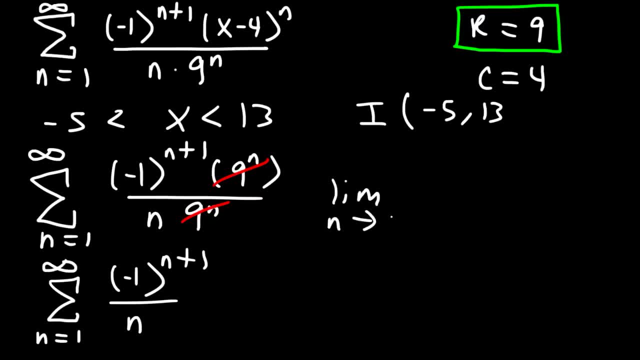 So let's start with the divergence test. So the limit as n goes to infinity. for a sub n which is 1 over n, that's going to go to 0.. Remember to ignore this. So it passes the divergence test. At this point the series may converge or it may diverge. 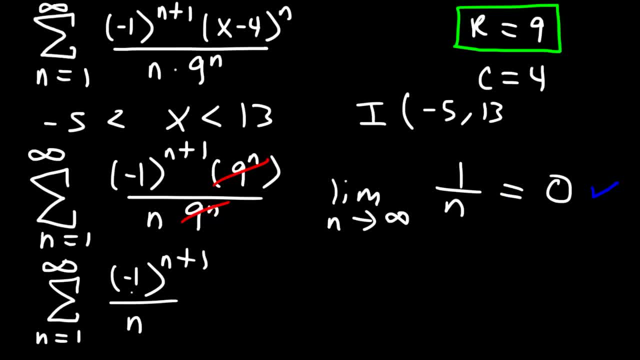 If it doesn't equal 0,, then it diverges. Now we need to show that a sub n is 0.. n plus 1 is less than or equal to a sub n. So a sub n is 1 over n And a sub n plus 1 is 1 over n plus 1.. 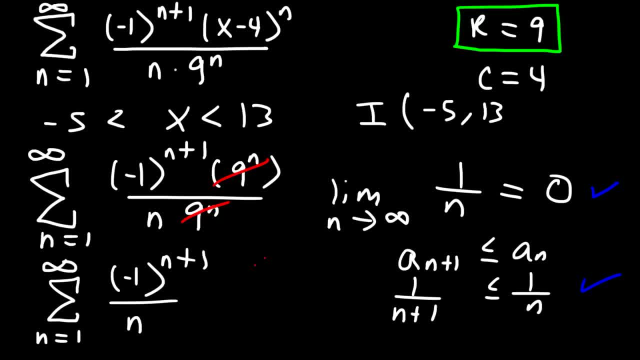 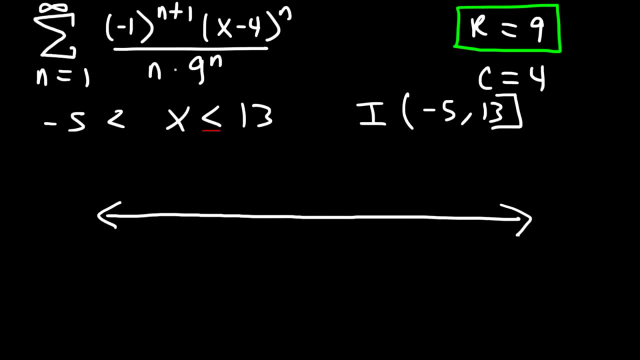 So that's true. So by the alternating series test we say that the series converges, Which means that 13 is included. So the interval of convergence includes 13.. So we're going to use a bracket for that. Now let's plot the solution on a number line. 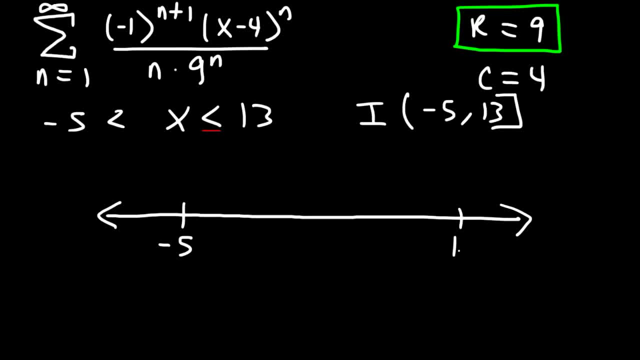 So it's going to start from negative 5 and it's going to end at 13. And it's centered at 4.. So 4 is right in the middle. So we're going to have an open circle at negative 5 and a closed circle at 13.. 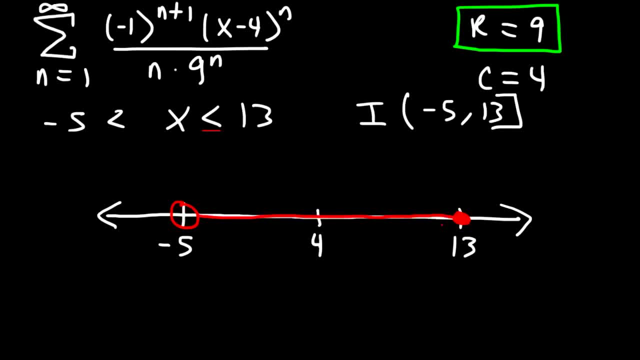 So this is the interval of convergence. Whenever x is between negative 5 and 13,, the power series will converge, And so in the middle we have our c value. It's centered at x, equals 4. And the radius of convergence is 9.. 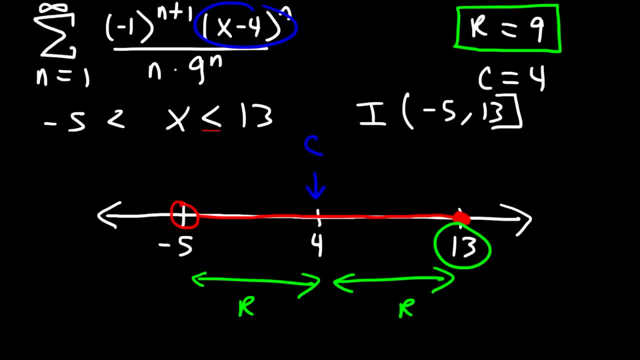 So 13 minus 4 is 9.. And 4 minus negative 5, that's also 9.. And so that's it for this video. Hopefully it gave you a good understanding of power series and how to find the interval of convergence and the radius of convergence. 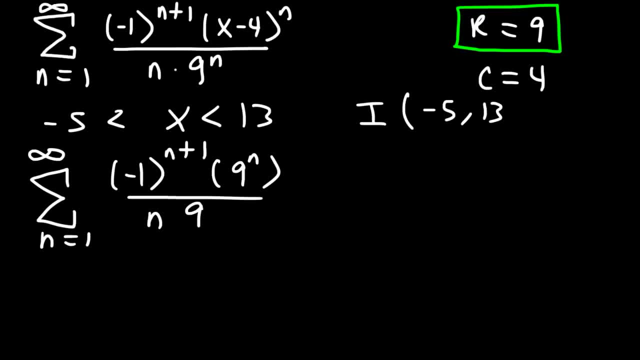 times 9 to the n, over n times 9 to the n. So these will simply cancel. And now we have the alternating harmonic series, So we need to perform the alternating series test. So let's start with the divergence test. So the limit as 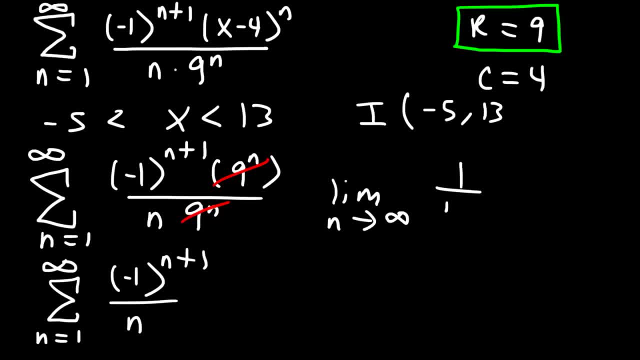 n goes to infinity. for a sub n which is 1 over n, that's going to go to 0. Remember to ignore this. So it passes the divergence test. At this point the series may converge or it may diverge If it doesn't equal 0. 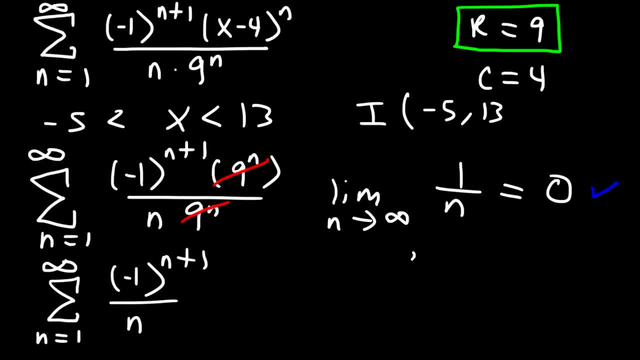 then it diverges. Now we need to show that a sub n plus 1 is less than or equal to a sub n. So a sub n is 1 over n And a sub n plus 1 is 1 over n plus 1.. 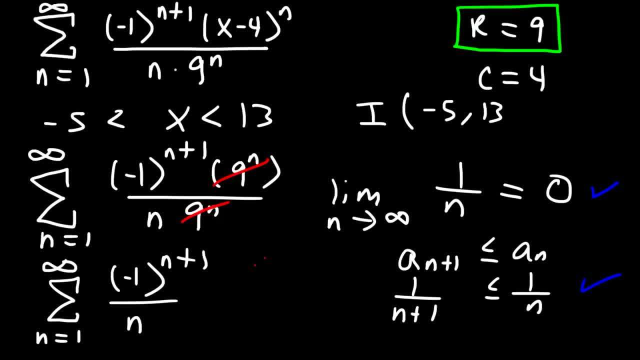 So that's true. So by the alternating series test we say that the series converges, Which means that 13 is included. So the interval of convergence includes 13.. So we're going to use a bracket for that. Now let's plot the solution. 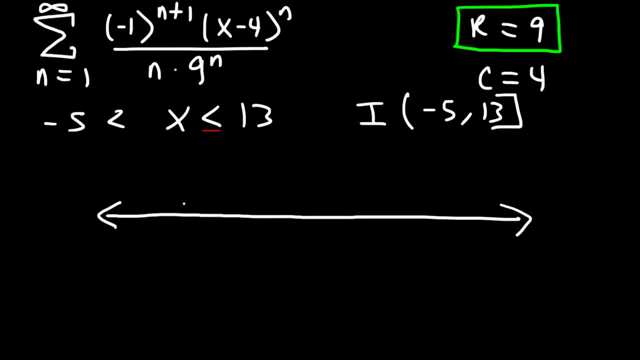 on a number line. So it's going to start from negative 5 and it's going to end at 13.. And it's centered at 4.. So 4 is right in the middle. So we're going to have an open circle at negative 5. 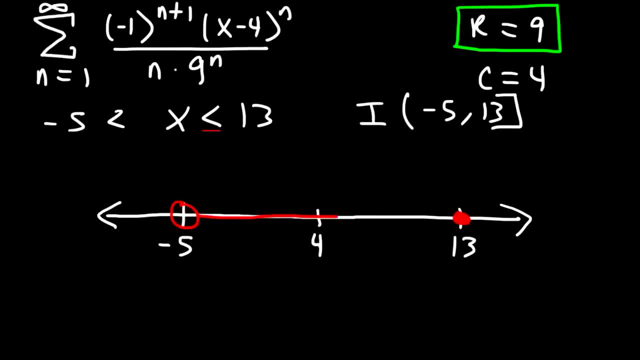 and a closed circle at 13.. So this is the interval of convergence. Whenever x is between negative 5 and 13, the power series will converge, And so in the middle we have our c value. It's centered at x equals 4.. 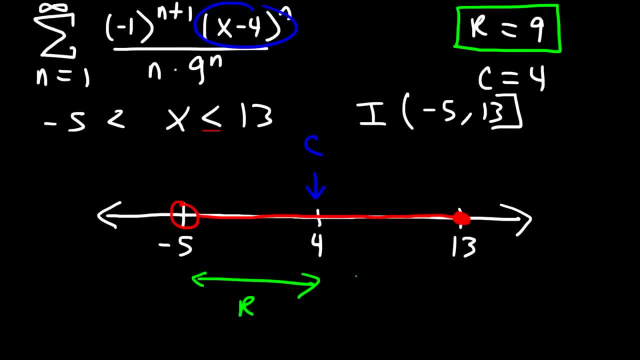 And the radius of convergence is 9.. So 13 minus 4 is 9. And 4 minus negative 5 that's also 9.. And so that's it for this video. Hopefully it gave you a good understanding of power series. 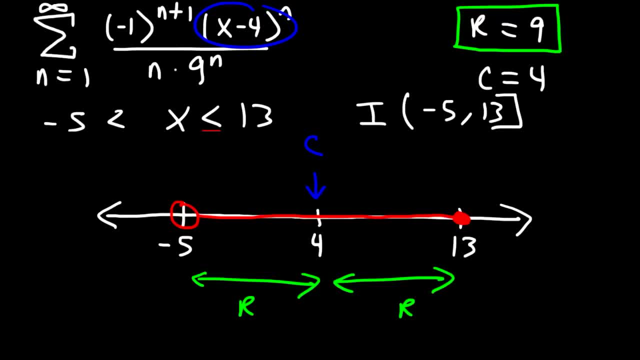 and how to find the interval of convergence and the radius of convergence. Thanks for watching. 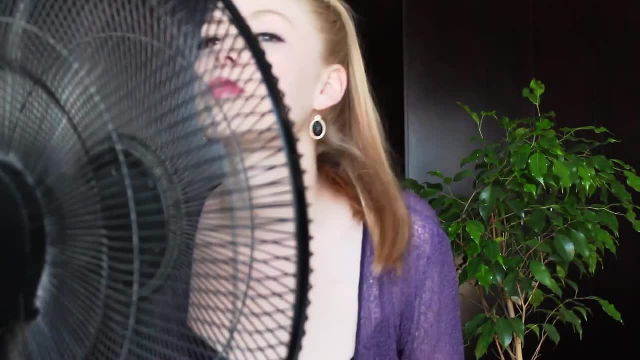 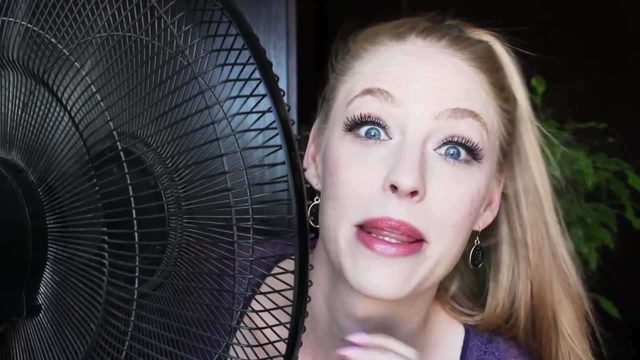 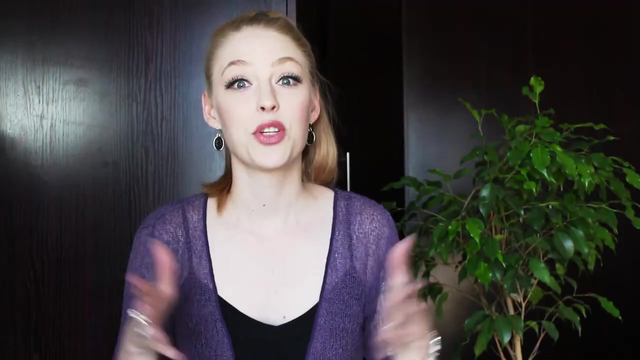 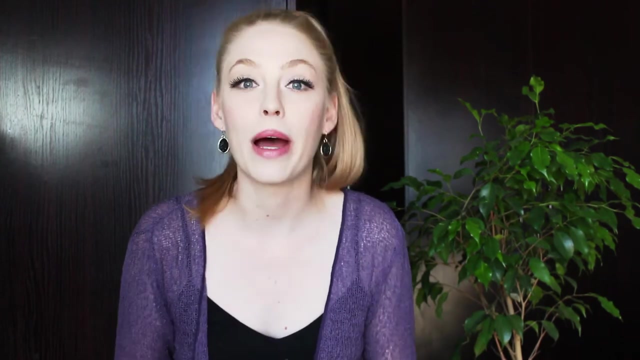 In this video we'll be talking about the movement of air. To understand how air moves around our earth, we need to understand the differences in pressure that exist. Now, when we talk about air pressure, we are talking about the weight that the atmosphere 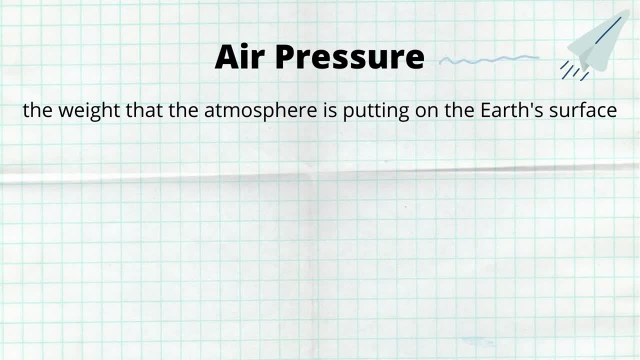 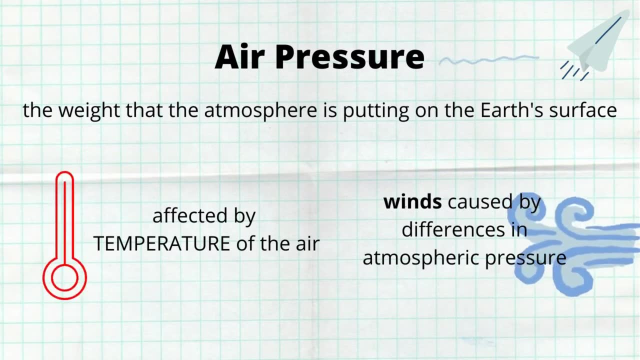 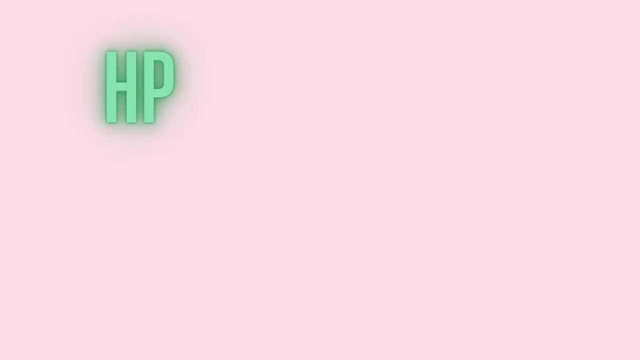 is putting on the earth's surface. Air pressure is affected by the temperature of the air and wind is caused by differences in atmospheric pressure. We get two main types of pressure: high pressure and low pressure. High pressure cells are associated with cold, dense air.